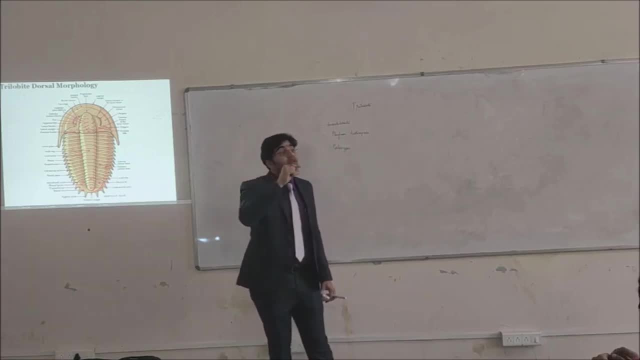 and, most importantly, short stratigraphic range Means it should be able to evolve quickly. If it won't evolve quickly then it will not be, you know, acting as a good index fossil. So the first occurrence, the global first occurrence of Trilobites was during. 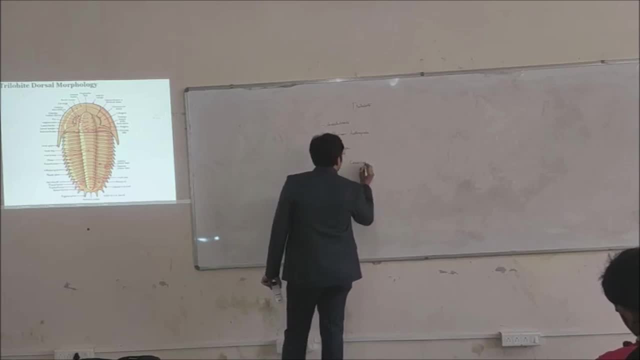 the Cambrian, So the beginning of the Paleozoic Era, So Cambrian period, the Cambrian explosion that we talked about. these were the important groups. Then the last occurrence: Permian. The PT extinction, the Permian Triassic Extinction. it saw the complete wipe out of the Trilobites. 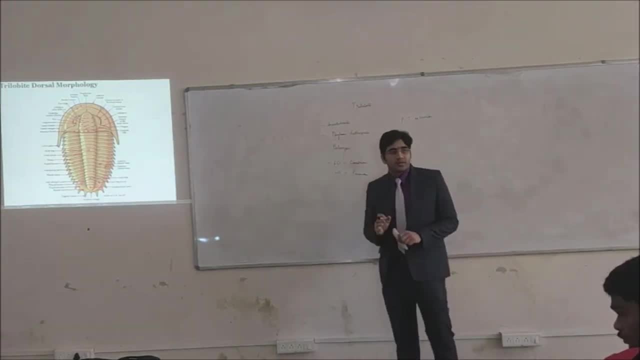 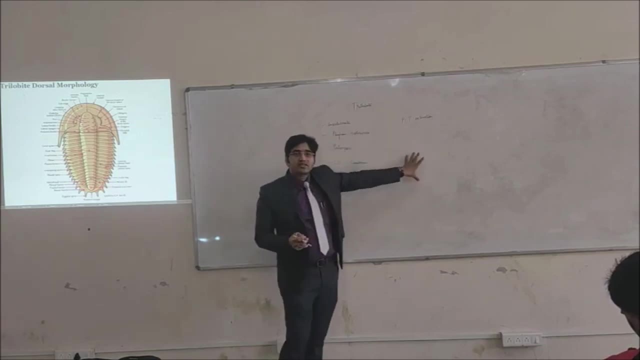 from the Earth. Okay, So they got extinct in Permian. You will not find the record of Trilobites beyond Permian. Therefore, such a small stratigraphic range, Trilobites, they are very important, Okay. 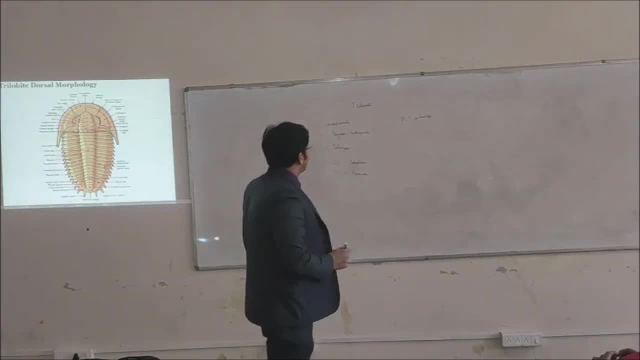 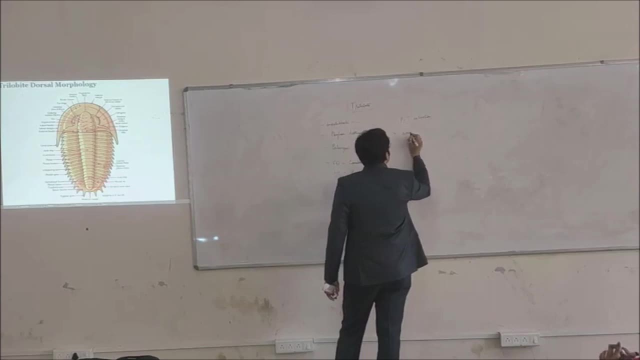 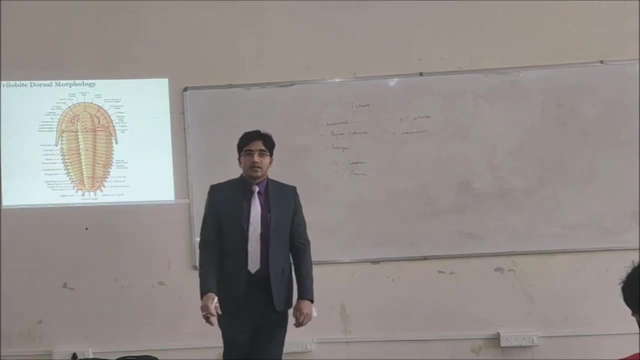 A few other things. The Trilobite weakened in vertebrae, It had exoskeleton, Exoskeleton, Okay, And this exoskeleton, which we classify in the Phyla-Martha quota, is known as Carapace. 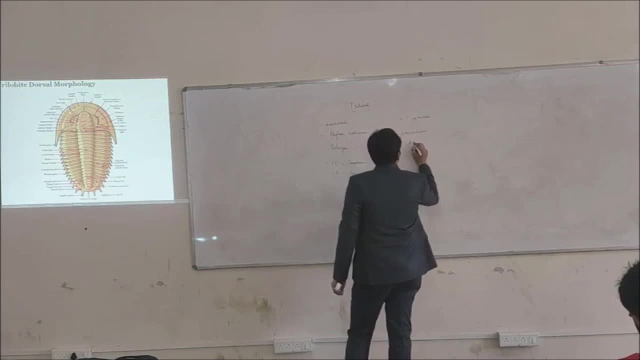 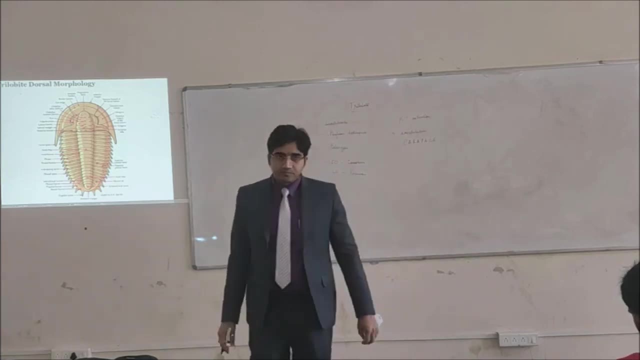 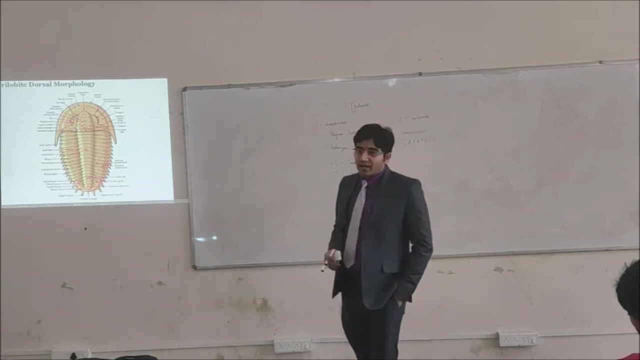 So what is the name given to the shell of, or the exoskeleton of Trilobites? You should remember this word: Carapace. Okay, Carapace. A very important thing is, which you should also know, that if in an area we go and we find, let us say, 100 Carapaces, 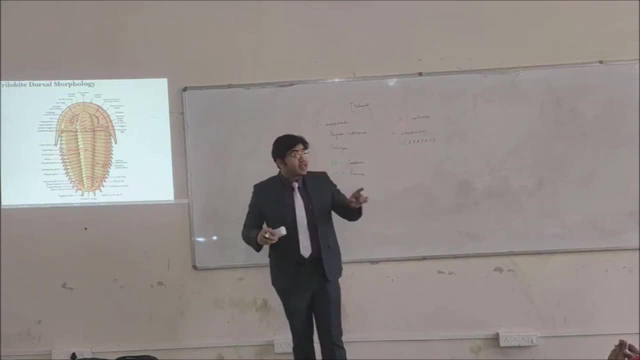 100 Carapaces. it is not that there are 100 different Trilobites, It is not. 100 Carapaces may be represented by maximum 8 to 10 or 12 Trilobite genus. only Because the Trilobites, they, had a very, very important characteristic which is called as Echidiasis, or molding. Okay, 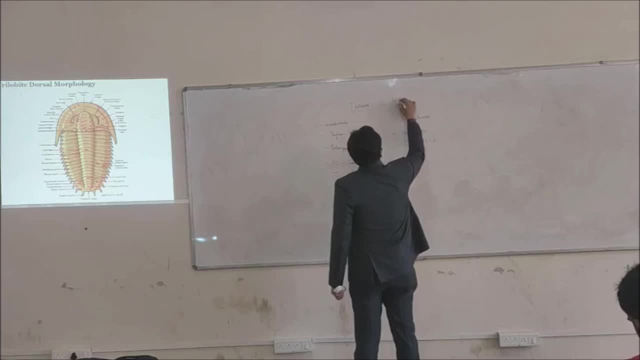 Trilobites, they could change their shell. Okay, They could change their shell. Echidiasis is also called as molding. This is a very common question asked in GSI exam. what is Echidiasis? So Echidiasis is the property of an organiser to change its shell and make a new shell. 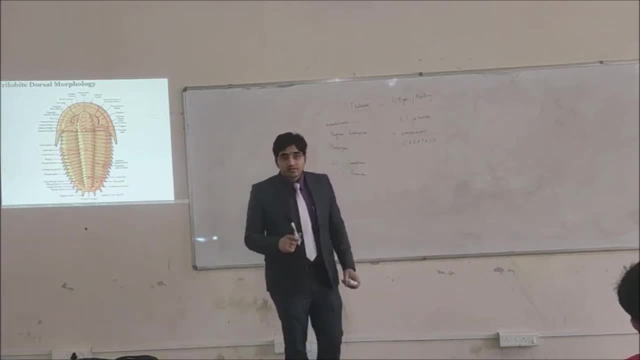 It has been found in research papers: Carapace. Carapace, It is the name of the exoskeleton of the shell of Trilobites. The diagram which you were making in the practical, you are actually drawing the diagram of the Carapaces. 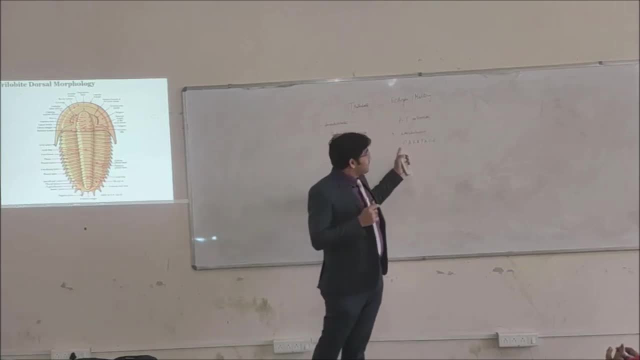 Okay Now, as I was telling, in research papers, if you read, you will come to know across that one Trilobite could do, or could make, 8 to 10 molds in its lifeline And it can change its body 10 times. 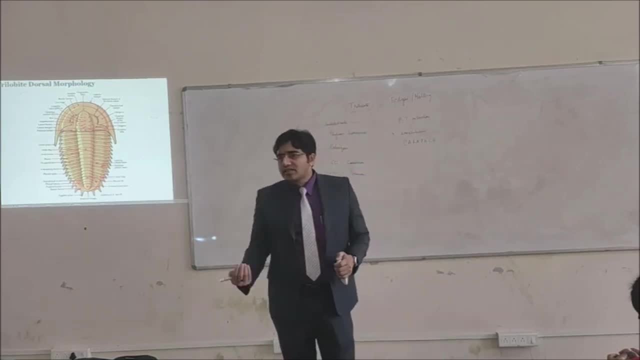 What was the need to change the body? Its growth in size? Okay, Okay, Okay, Okay, Okay. Yes, of course it survived. It had to change its body, So as it grew in size, it used to change. 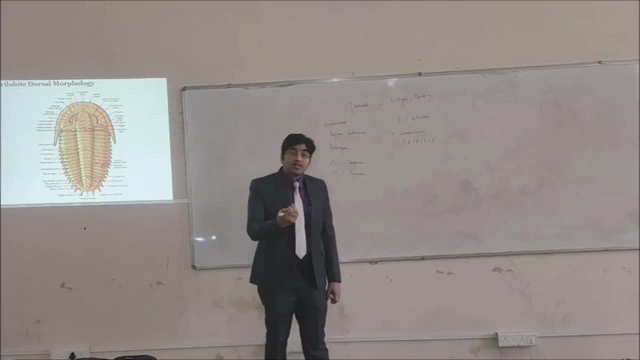 You will see what molding was And what are the fossil evidences of molding. So one Trilobite could make 10 to 12 molds in its lifespan. So if in an area you get 100 Carapaces, it is not necessarily 100 Trilobites. 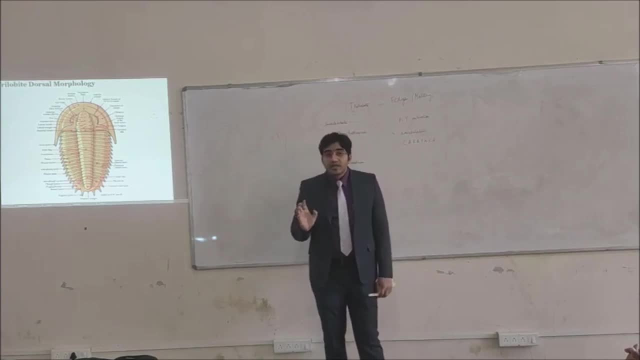 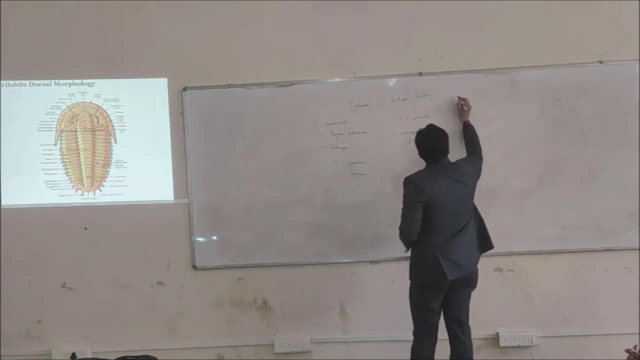 They could be 10 or 12 Trilobites only, which have made these. Therefore, Trilobites can also be called as ECDISO-ZOA, ECDISO-ZOA. ECDISO means to change its skin. 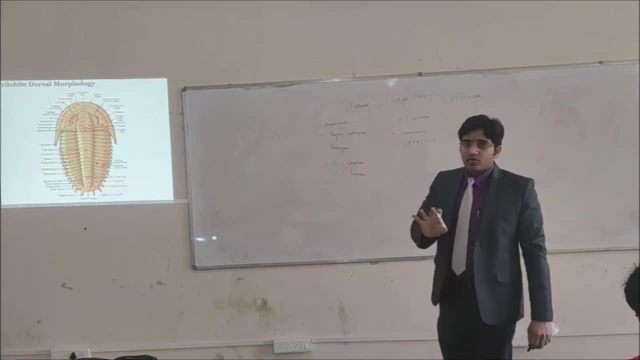 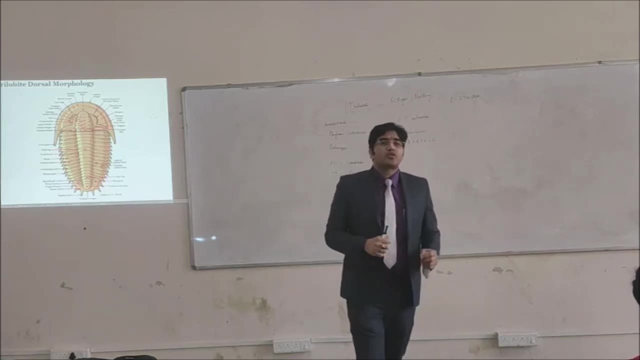 ZOA means hair. This introduction you understood, Sir. the first skeletal organism was Trilobite. The first skeletal organism was small Shelly fauna, The small Shelly fauna or SSF, which occurred as the first first Shelly organisms. 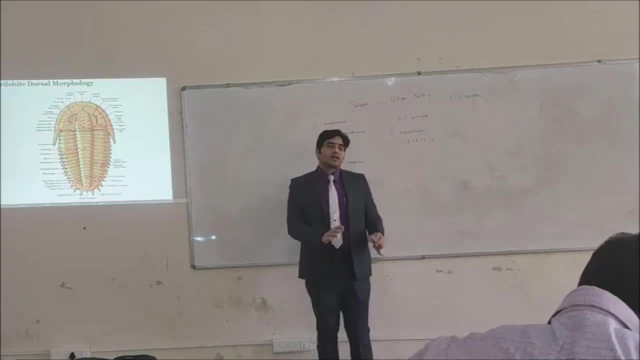 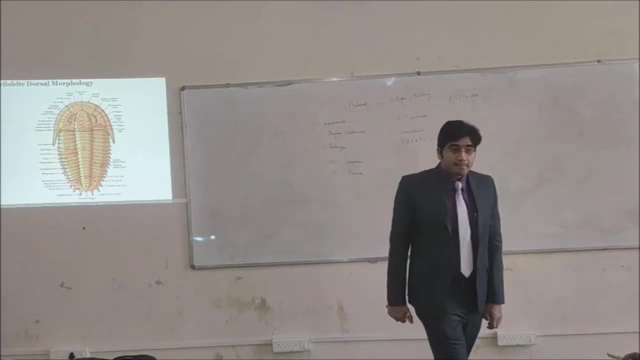 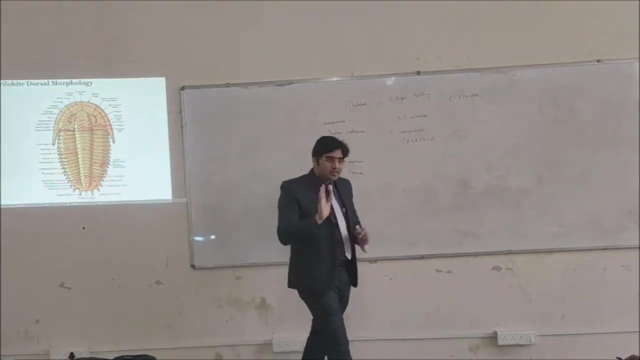 After that, we have this complex organism which we call Trilobite. Okay, Sir, what Glabella, or Carapace? Glabella is this ocean. It is a part of the Carapace itself. Whatever you see which is preserved is only a part of the Carapace. 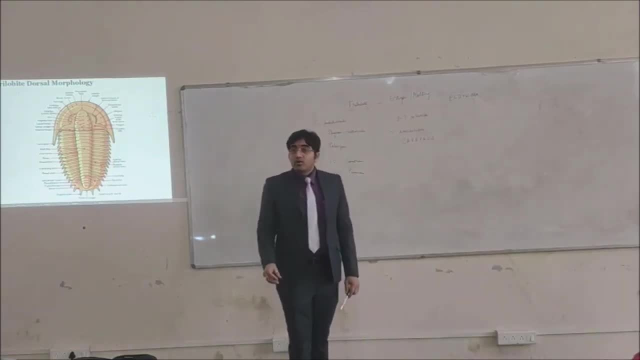 Okay, No, From which organism did it evolve? What was the predestination? What was the predestination? Because, if you remember, I had told you about the Adiagora fauna, soft bodied metagormans, soft bodied organisms. 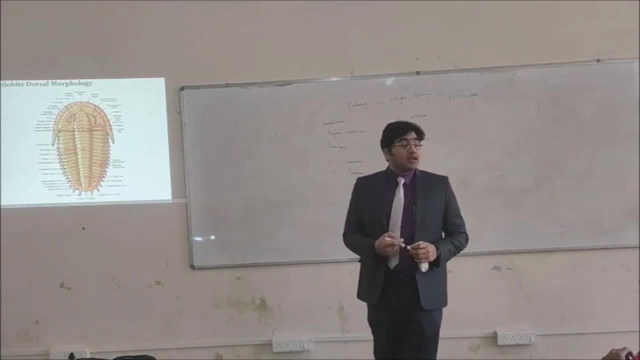 which did not have those such hard skeletons. So there is a Adiagora genus Parvanchorina P-A-R-V-A-N-C-O-R-I-N-A. I will show you the diagram, also Parvanchorina. It is considered to be the ancestor of Trilobites. Ancestor of Trilobites, Ancestor of Trilobites. Parvanchorina P-A-R-V-A-N-C-O-R-I-N-A. It was an Adiagora fauna. 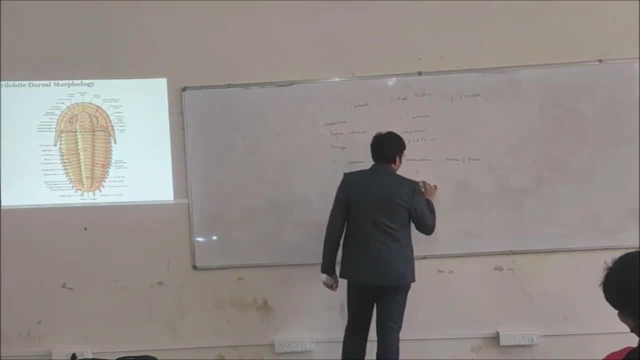 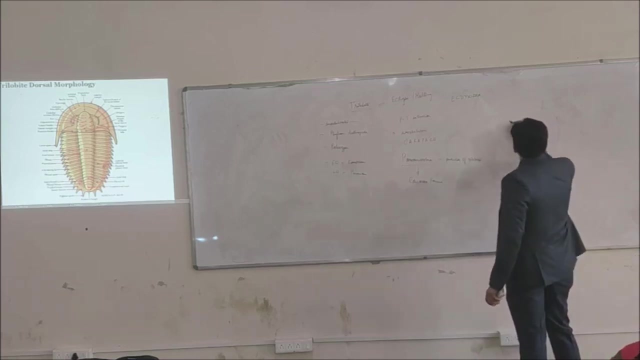 Soft bodied metagormans: Adiagora fauna. Okay, The Parvanchorina looks somewhat like this. This is the diagram. It probably could be the ancestor of Trilobites. You see its picture? It probably looks like this. 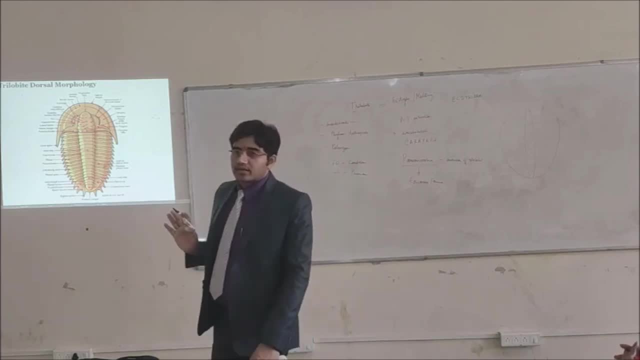 And therefore we consider it to be the ancestor of Trilobites. Okay, You understood this introductory part. Can we move ahead now? So the Trilobites: first of all, we need to have a brief about its morphology. 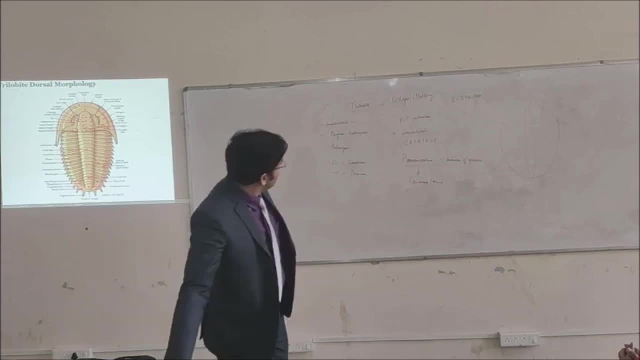 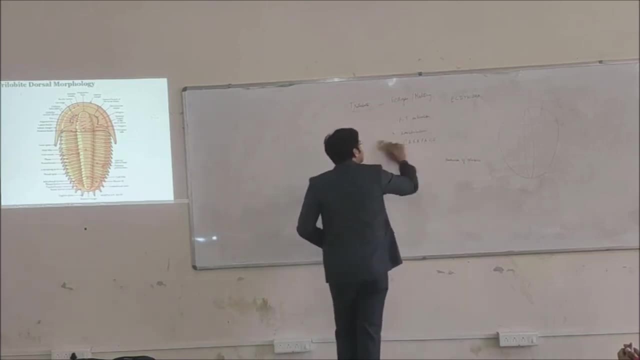 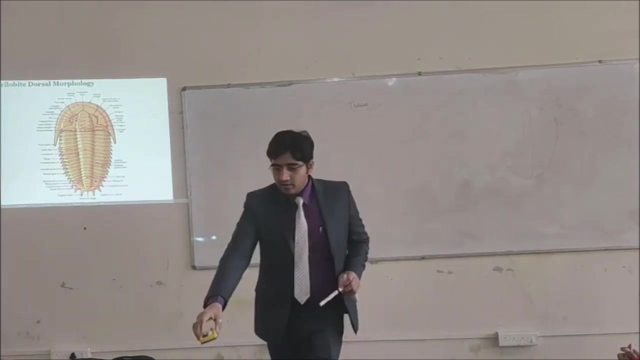 Then we go ahead with the functional morphology. So the name Trilobites, as I have already told you in the practical briefing, it is because of the three lobes which are there in its carapace. So what are those three lobes? 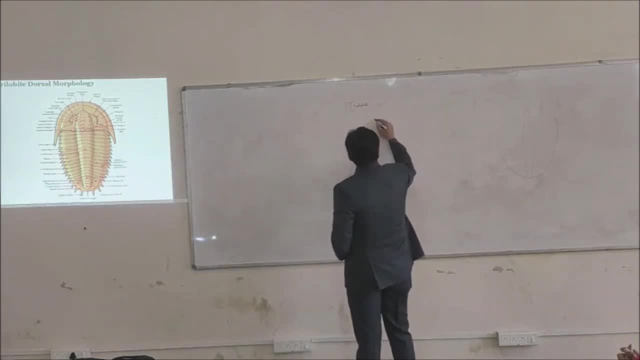 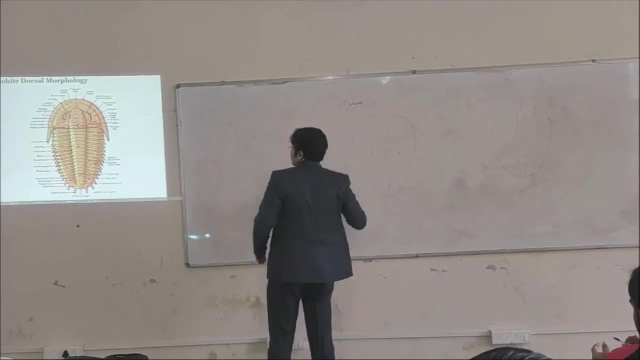 We have Cephalon. thorax and pgm are not the three lobes, They are the three segments. It has segmented bodies. So we have these three lobes: One axial lobe and two pleural lobes. 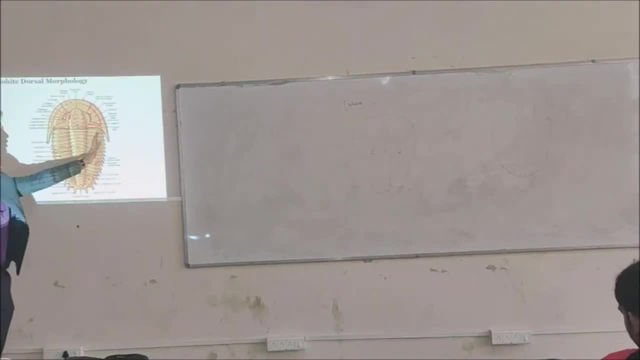 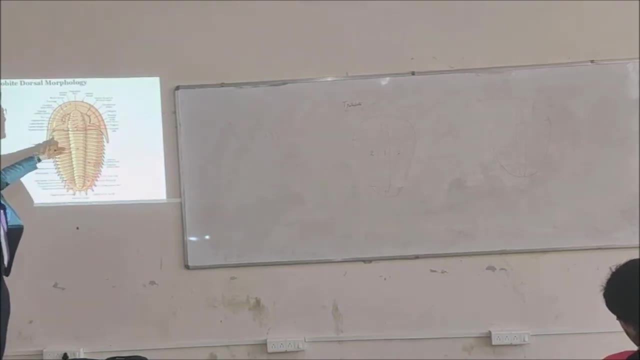 As you can see here, one axial lobe, two pleural lobes. Axial lobes is the central portion, which consists of the glabella, thorax and the glabella, While these pleural lobes they consist of the pleurae, which have these appendages on the carapaces. 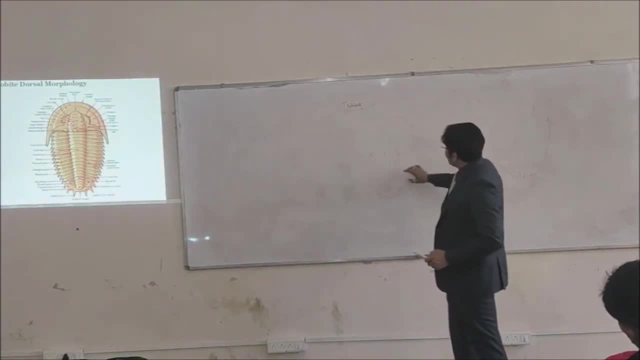 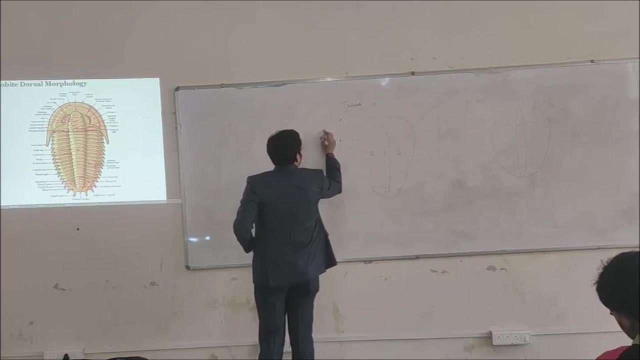 So if you look at the general outline of the morphology of a Trilobite, it would look like this that it has three lobes, One axial and two pleural lobes. While it has three segments, The top first segment is the cephalon or head. 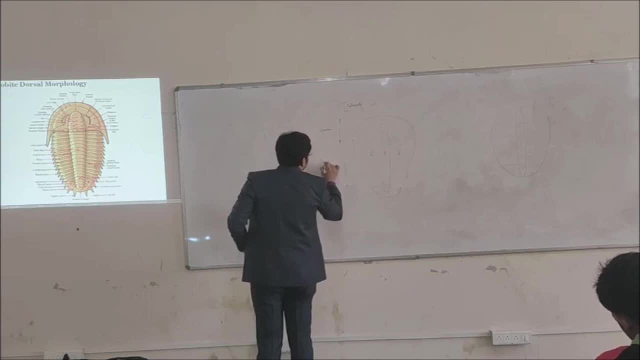 Followed by the thorax or trunk, And the third one is the tail or the pgm. So here you can see the cephalon thorax and the pgm. So what we look at is the dorsal morphology. Okay, 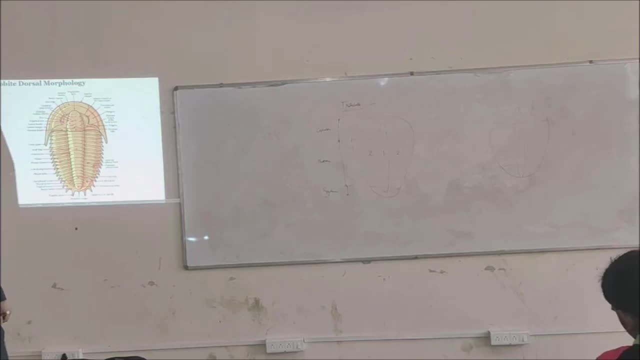 It means there should be a ventral morphology also. This is the decayed diagram. I am not discussing it here because we have already discussed it in your patented class, But you need to level the diagrams like this, Okay, So you should learn this. 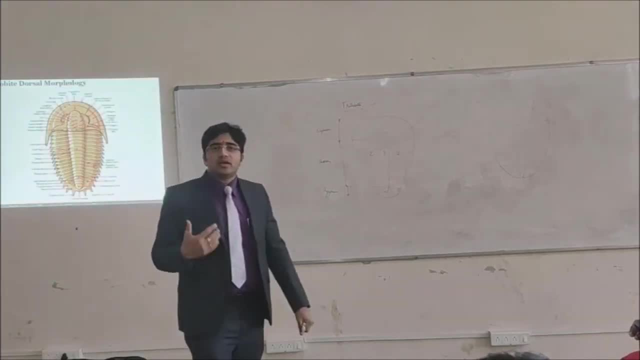 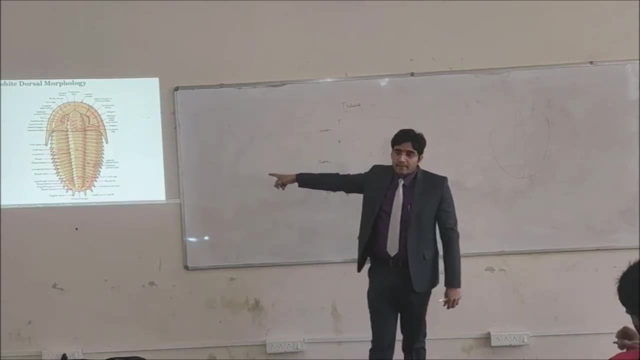 If a question is asked in the JSI exam, draw a full-page diagram of a Trilobite and level its part. This is how you should level it: The dorsal morphology. Is this okay, Did you understand? Now we will discuss all these parts separately. 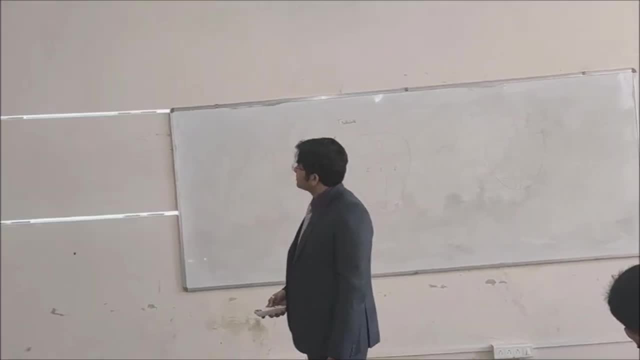 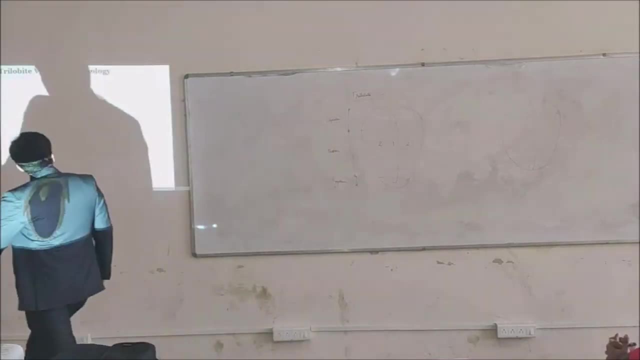 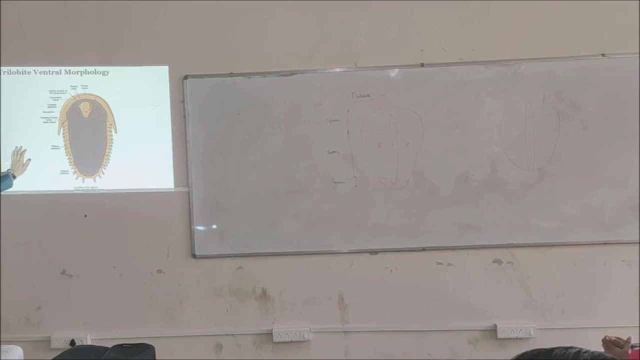 Okay, Look at the ventral morphology. This is not possible for you to see in a fossil, because the carapaces that we get, they are the casts which are embedded on some rock surface, So you will not be able to see. 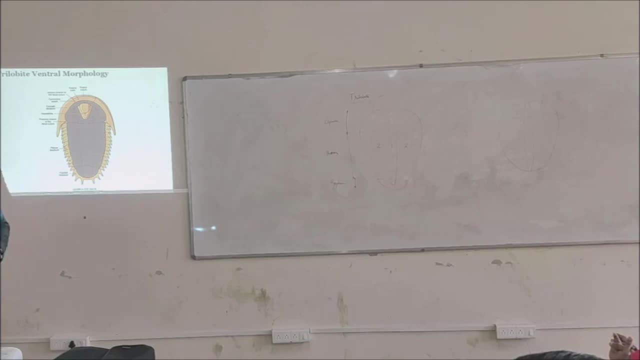 But if there is a place in Canada, the Burgess Shale, The Burgess Shale National Park, If you go over there, that is called as the heaven for Trilobites Seekers. This has been in, you know. people are visiting there for several decades now. 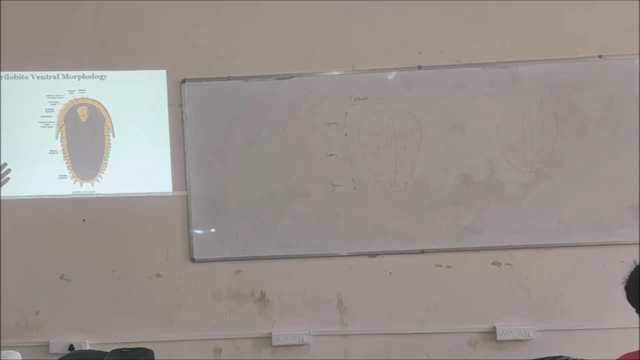 But still, if you go, you will each time get some new genus of Trilobites, Full of Trilobites. Trilobites, they were shallow marine organisms, shallow marine creatures. They turned from aquatic to amphibians. 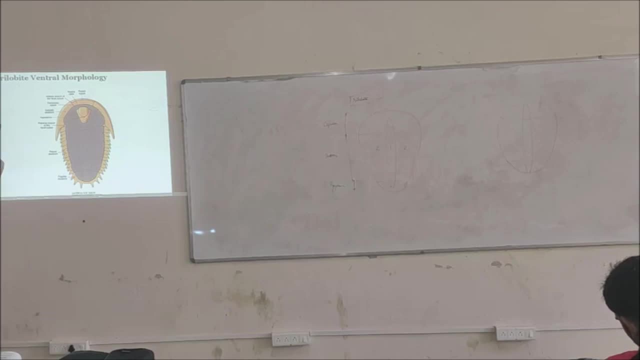 Amphibians. They could live in water or they could move on the land. Trilobites were among the first organisms to have eyes. They were not blind. The first Trilobite genus which we call as Red Lychia. 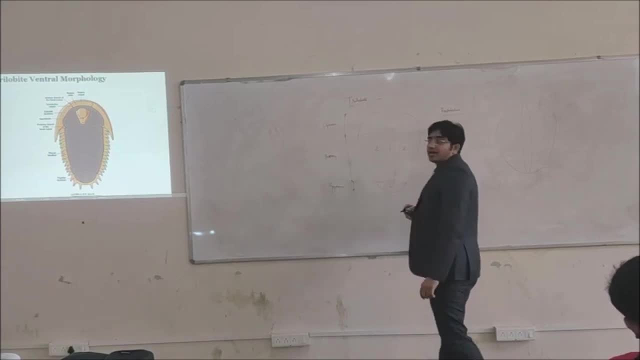 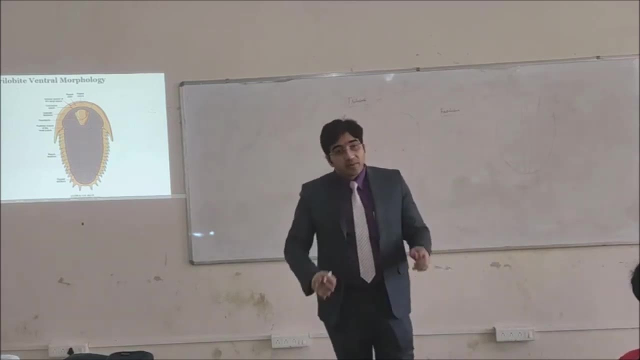 which was the first Trilobite which you remember saying Red Lychia, not Libby Red Lychia. we are going to give a copy. Order Red Lichida. So these were the first Trilobites, but they had eyes. 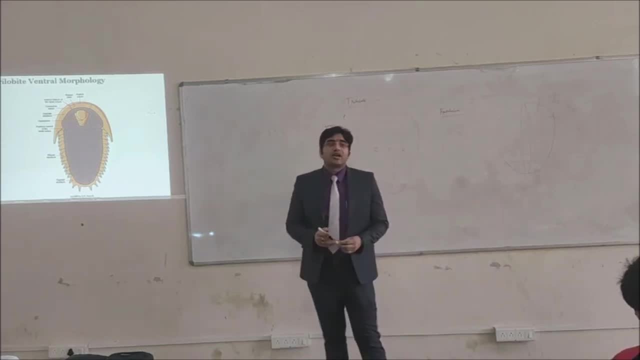 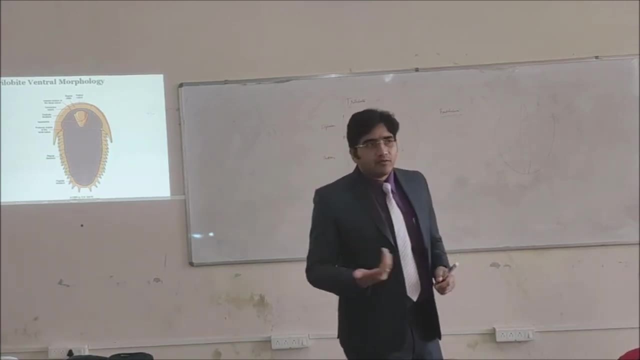 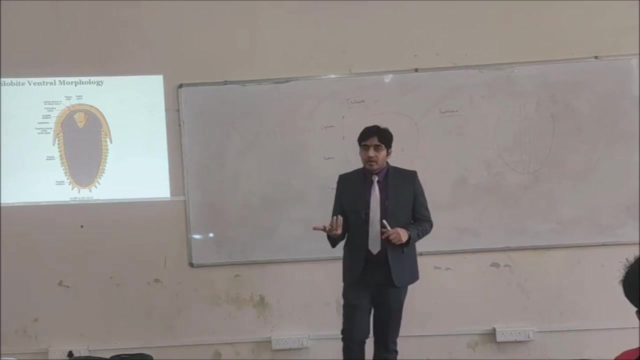 In subsequent course of time, the Trilobite lost its eyes, Means, they became blind. We will see why this would have happened. We can only make guesses, right. We can only guess why this happened. Why did this happen? Then, later on, the Trilobites: they again had eyes, but they became secondary, eyeless Trilobites. So blind Trilobites. there were two kinds: Primary Eyeless Trilobites and Secondary Eyeless Trilobites. So I will give you an example of Primary Eyeless Trilobites which did not have eyes. Agnostic, Agnostic, Trimediasis. All these were blind Trilobites, Primary, Eyeless. They did not have eyes In the order Trachopida, they are Pecops. It was Secondary Eyeless Trilobites. 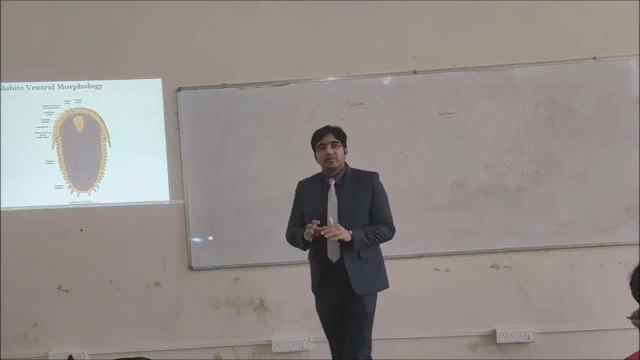 Means. it had eyes in the beginning. In the due course of time, this genus lost its eyes. So all these, you know, you need to know and you need to make the best guess, why this would have happened. Why did it have eyes? 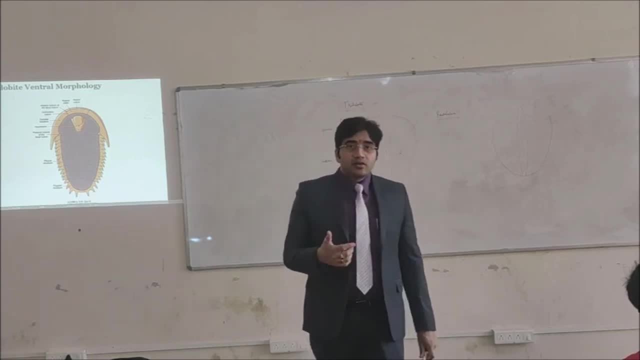 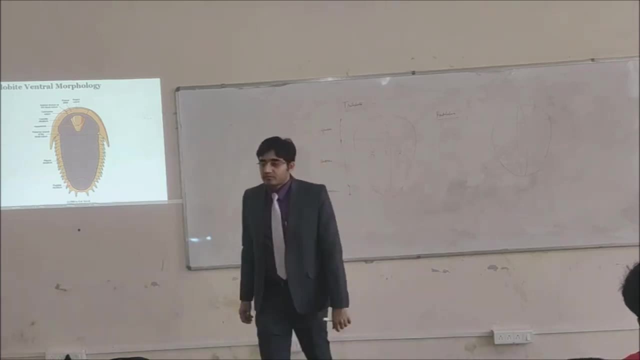 Then it lost its eyes. Then why did it come back? Okay, So we will see. We will see the structure of the eyes, We will see the lenses of the eyes. in this class Now, one very common question which is asked is the mouth of Trilobites. 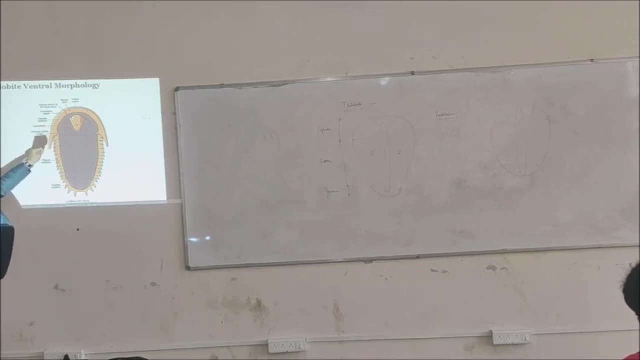 Hypo stove. Hypo means below Stove means opening Hypo stove. So whatever I have told you here, you should remember, as I have told you, what is the name of the disk or the shell of the Trilobite. 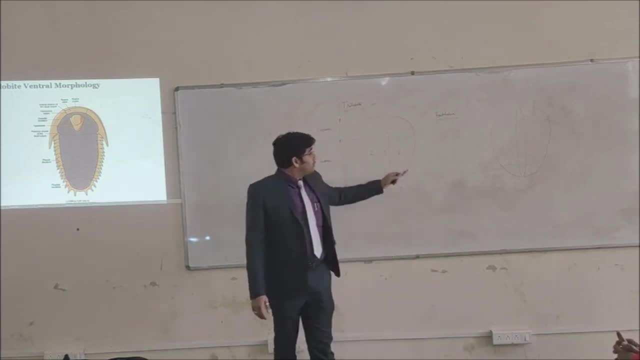 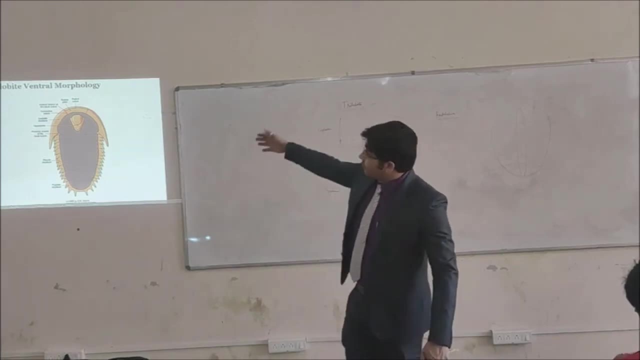 Keramase, Then which was the first Trilobite Redlichia, Ancestral, Trilobites Permethorina, Then which part is known as the mouth of the Trilobites, Hypo Stove. 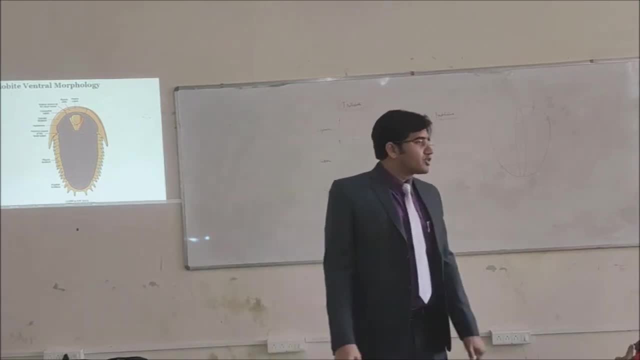 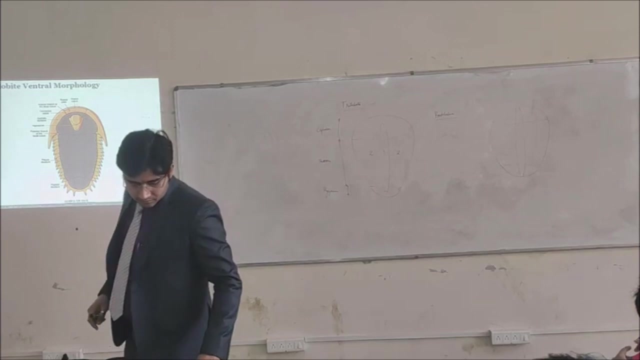 When we will be looking at the subsequent different fossil groups. what is considered to be the mounds of Gastropoda, that is, the Radula, means. these were probably those parts which were used for feeding medicines. Now let us look at the Cephalon. 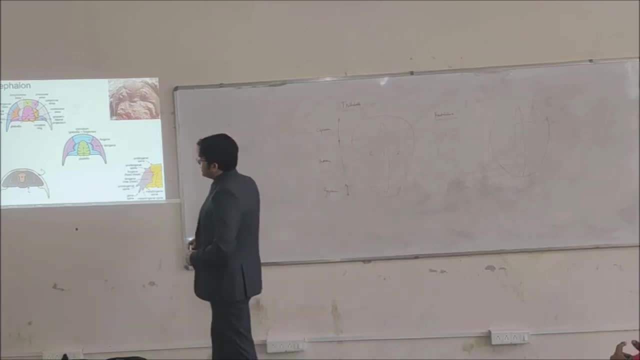 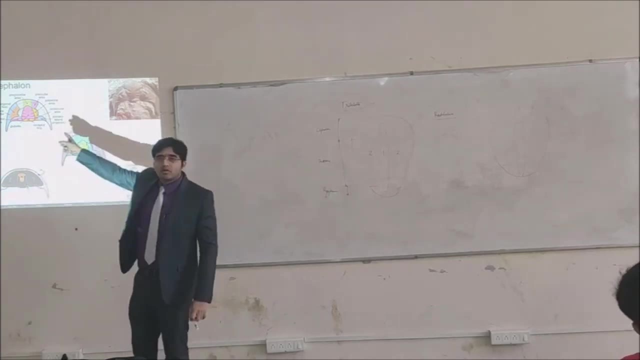 the top most part. To help you out, I will not be discussing about the ventral part. I will be talking about the dorsal part, because that is what you are going to see in the fossil record. So if we look at the Cephalon, 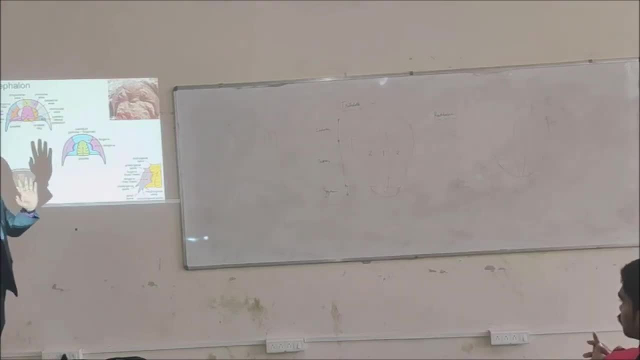 there would be different types of Cephalon depending on the genes. Sometimes Cephalon is larger in size than Pigeon, at other times it may be, so you can have this kind of a mound. This is the Cephalon. 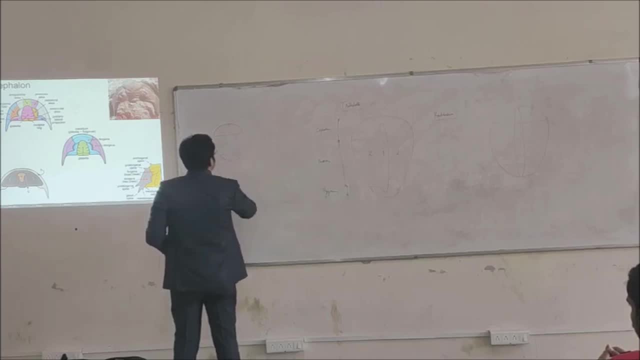 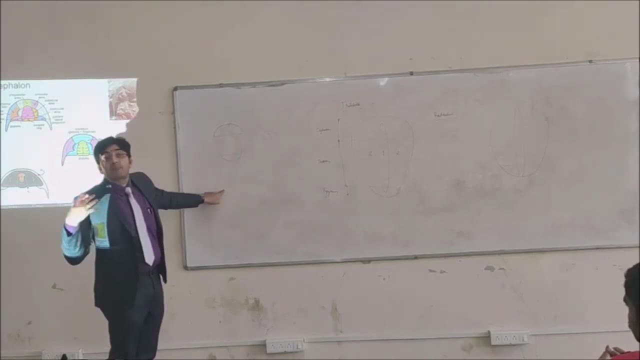 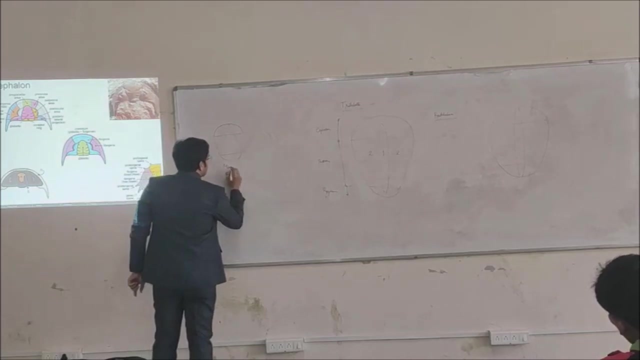 and this is the Pigeon. So since Pigeon is smaller than Cephalon, we call it as Micropyrus, Pyrus or tail of Pigeon. micro means small, So this is called as Micropyrus. 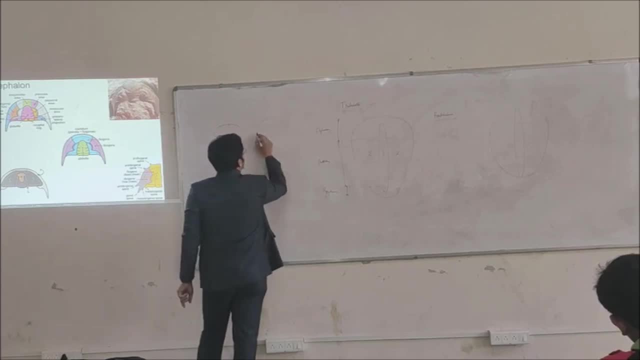 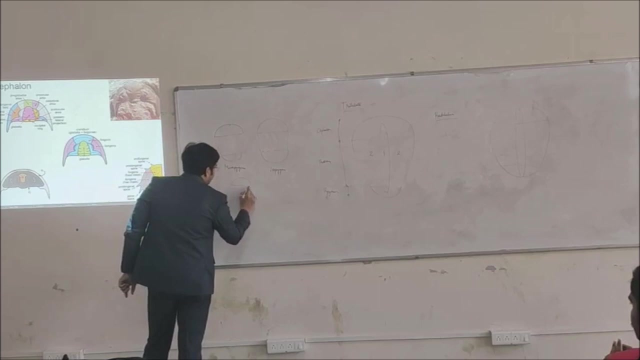 Then suppose they both are equal in size, Almost equal in size, so we will call them Isopyrus. Then if Cephalon is smaller and the Pigeon is larger, we will call it as Micropyrus. So 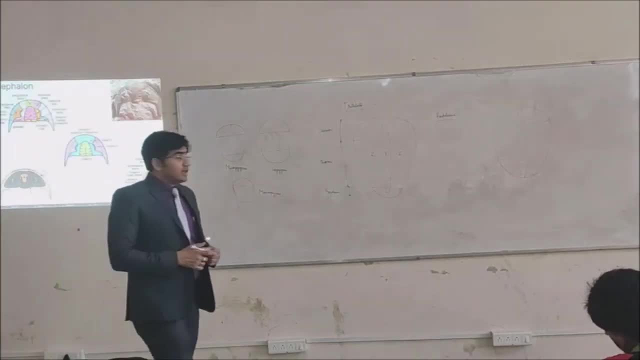 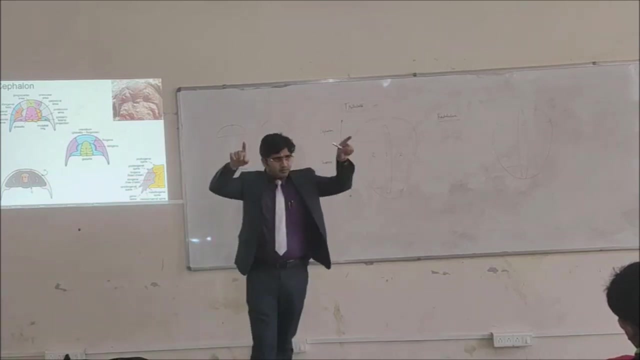 we can have different types of shapes of Cephalon. If you look at this, this is called as the head shield, the top most part, the head shield. Head shield is kind of semi-circular to elongate. It can be, for example, 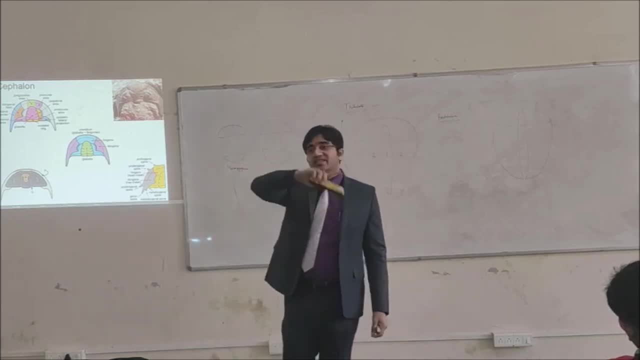 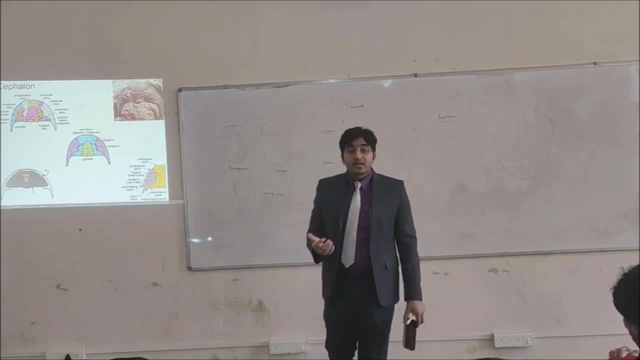 you saw Paradoxides, which had semi-circular head shield. You saw Olinus, which had slightly linear and elongated head shield. Then you saw Trinucleus, which was a very, very large, huge head shield. So it can vary Now. 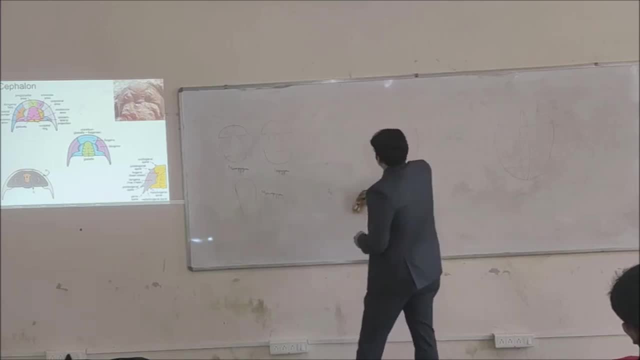 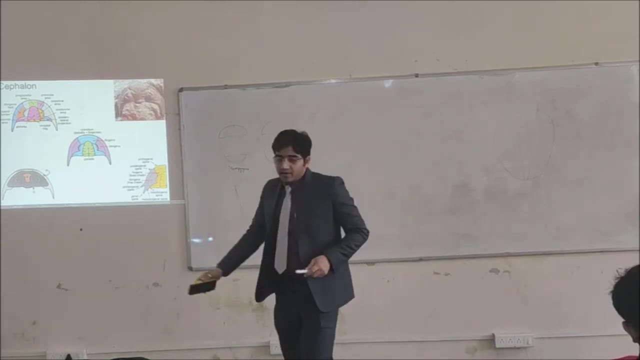 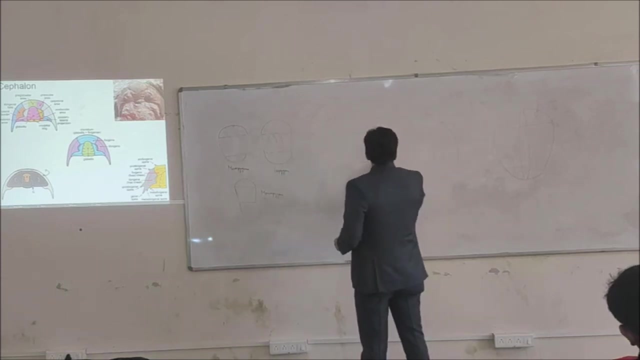 in the Cephalon there are several parts. The raised portion in the middle of the Cephalon. we call it as the glabella, the glabella portion. You should remember how to make these diagrams. So this part becomes the head shield. 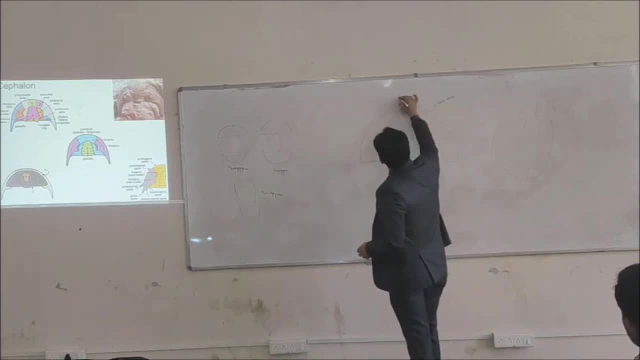 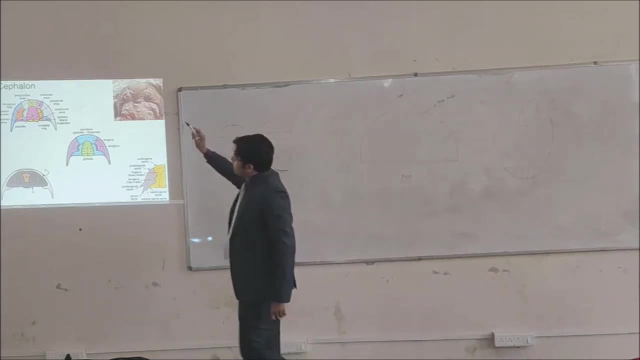 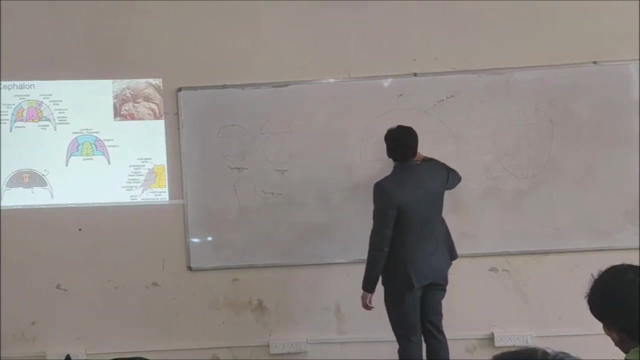 Alright, this is the anterior portion and this is the posterior portion. Now you can see here this glabella portion, glabella. Now glabella can vary in shape, shapes and sizes. Sometimes the glabella may extend up to the head shield or its italic shield. 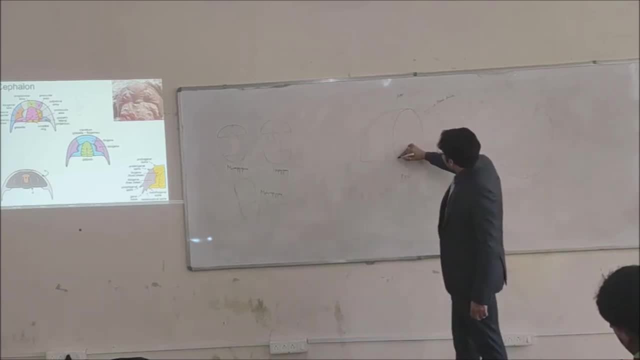 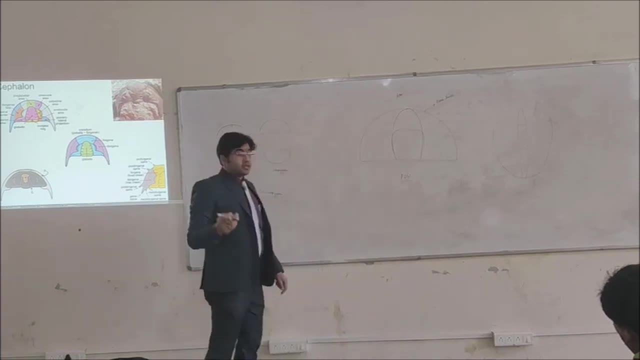 Sometimes the glabella might be smaller in size, Like in Calamine. you saw, the glabella was made up of globules. It was globular like this with lateral curls. In some Trinobites you can find the glabella. 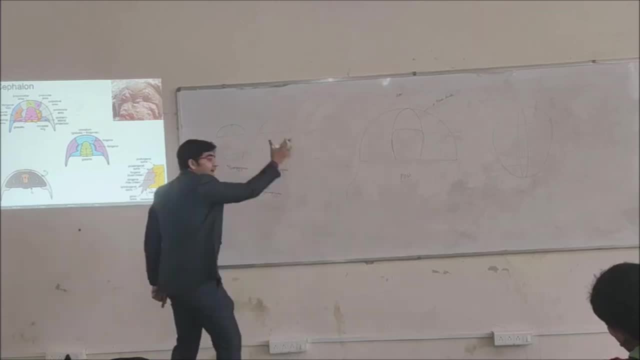 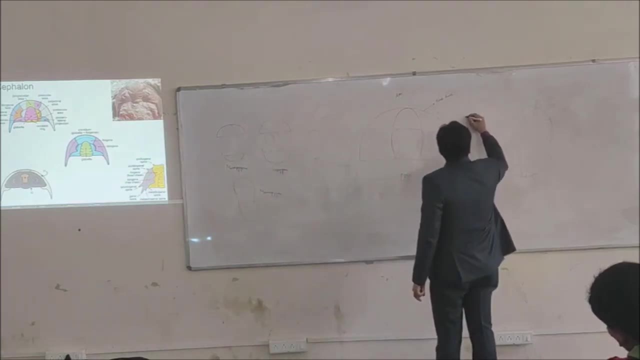 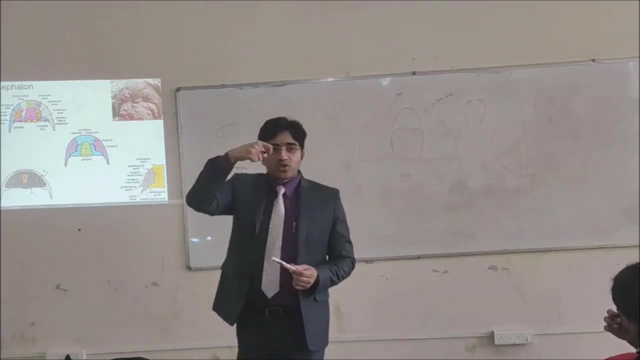 which is very wide. in the anterior side, In Trinobites, you will find the glabella which is pile form. Like this, Pile form means pear shape. You have seen pear, right? How does a pear look like? If you reverse it, it looks like glabella. 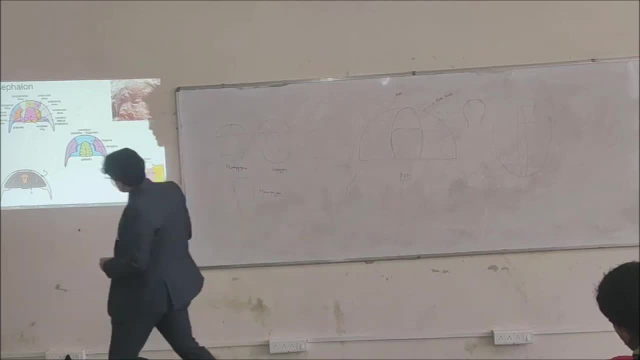 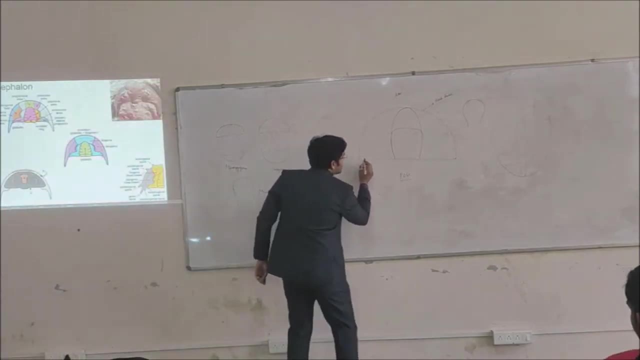 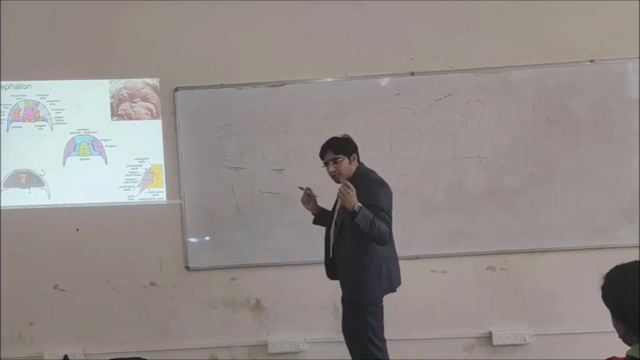 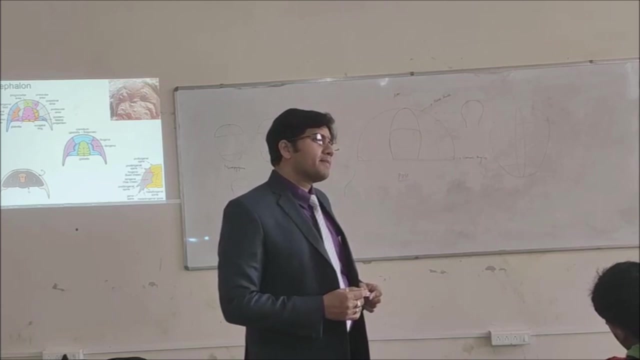 The central raised portion. Then these are the genus angles, These, This portion, it is called the genus angle. Now these genus angles may be pointed, may be rounded. Yes, Sir, what is the genetic difference between the genus and the glabella? 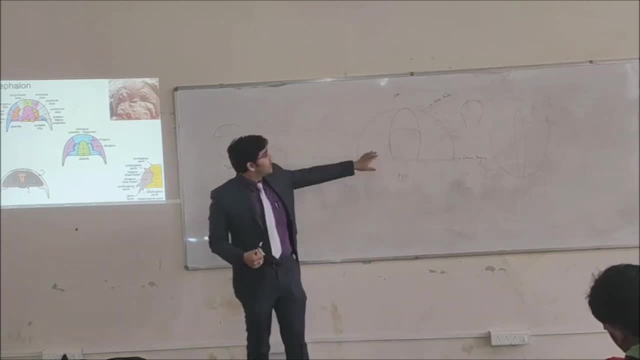 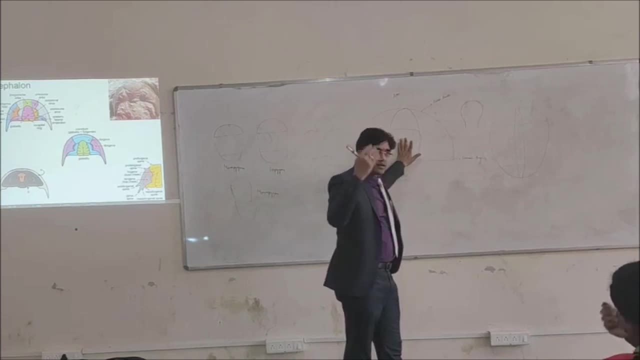 According to different genus. Different genus can have different glabella. If you look at the shape of the nose of different human groups, you will find that not everybody has elongated nose. not everyone has a chakta nose. not everybody has a chakta nose. 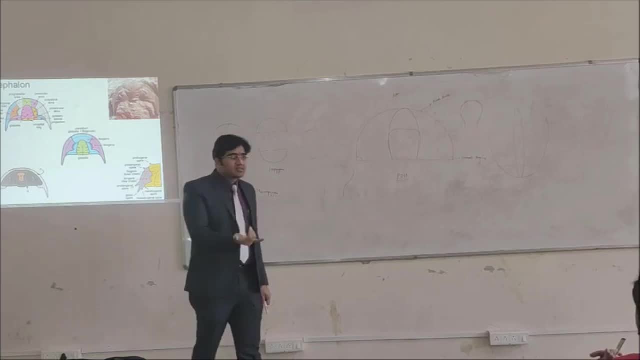 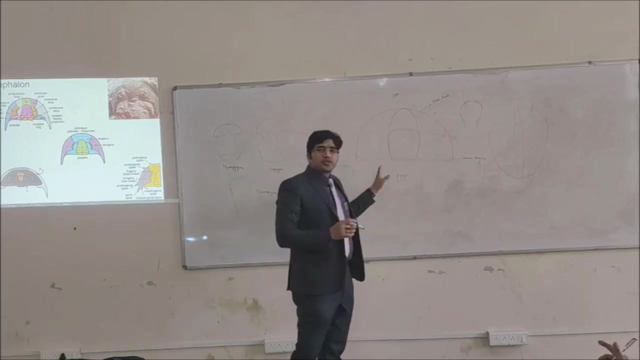 somebody has larger nose Depends. Genetics is the main thing which controls that. So these were most primitive organisms. Different genera had different glabella sizes and shapes. The genus angles could be smooth, genus angles could be rounded, they could be pointed. 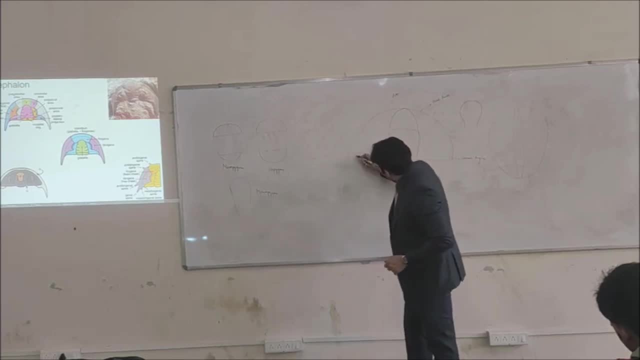 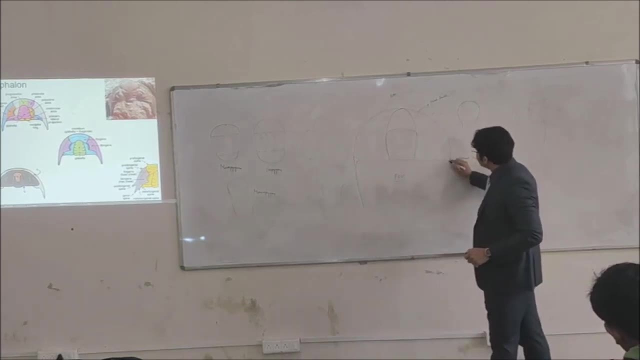 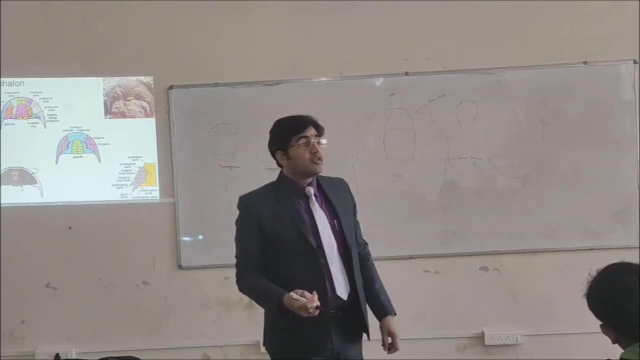 In some genus, in some groups of glabella, the genus angles could be modified into spines This way, And the shape of these spines could also vary, For example, in paradoxites or in red lichida order. you will find that 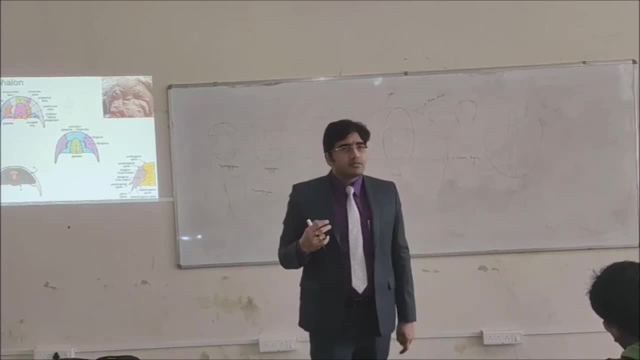 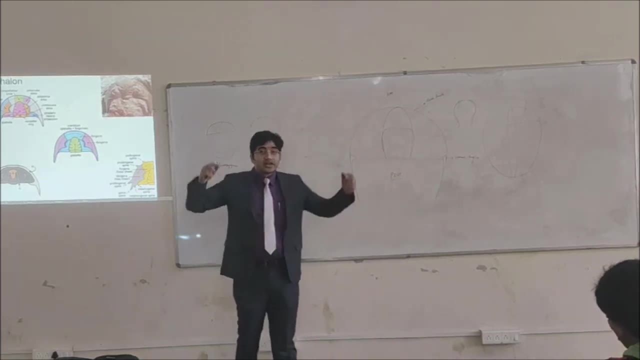 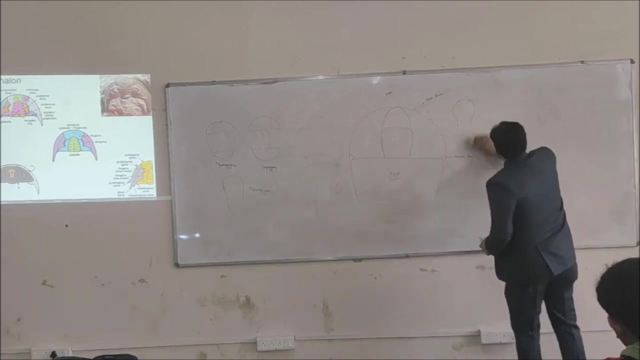 they had very long and slender and pointed genus spines. In oleus, you saw it had very small genus spines. In triglycerides, you saw it had again very thick and longer genus spines. So if you would like to know, 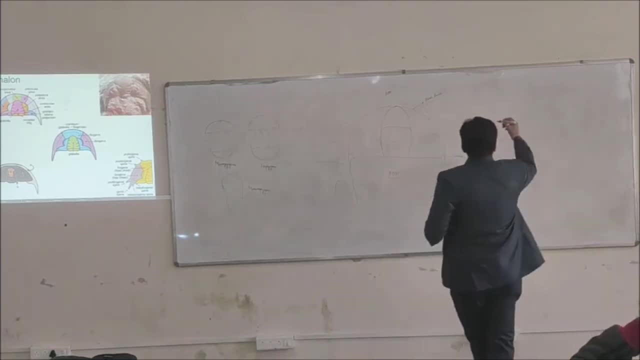 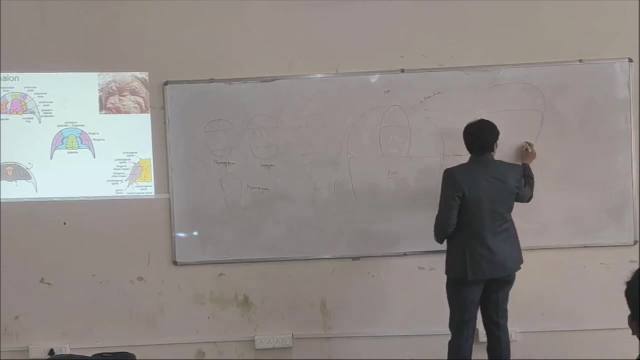 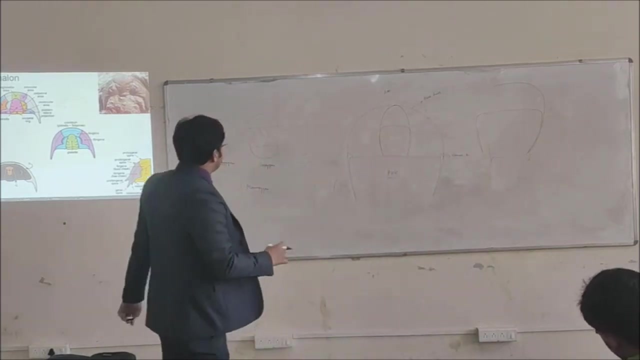 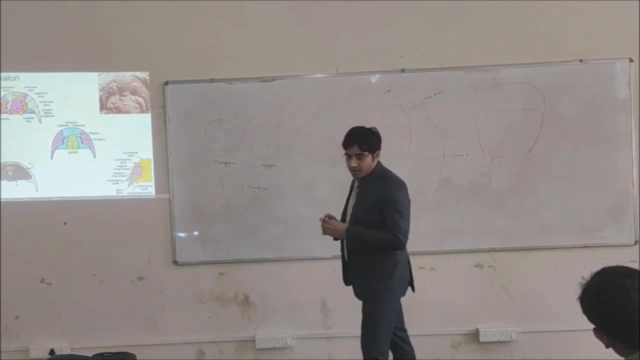 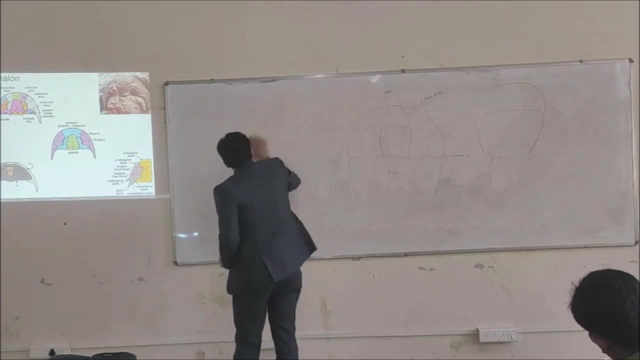 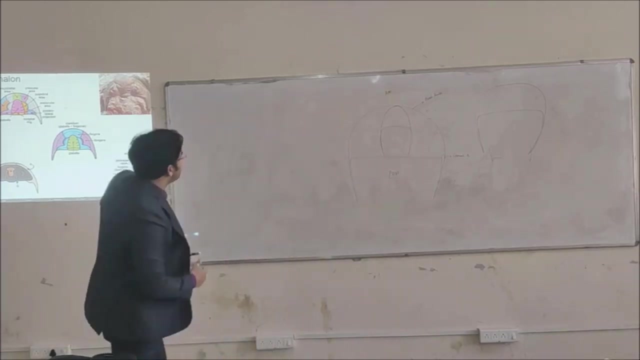 about the genus spines. you will have different shapes Or you could have genus spines with different genus spines. This way depends. Then in the zetalon you have the facial sutures. The facial sutures were very important. 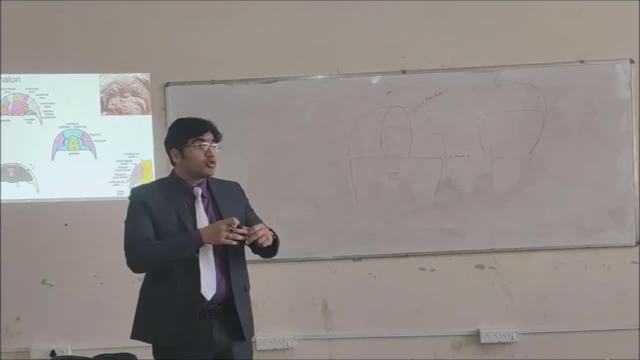 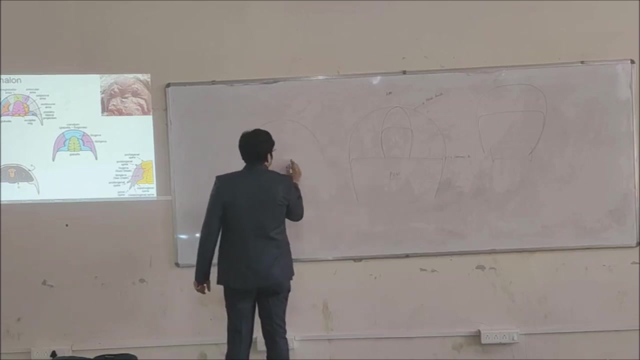 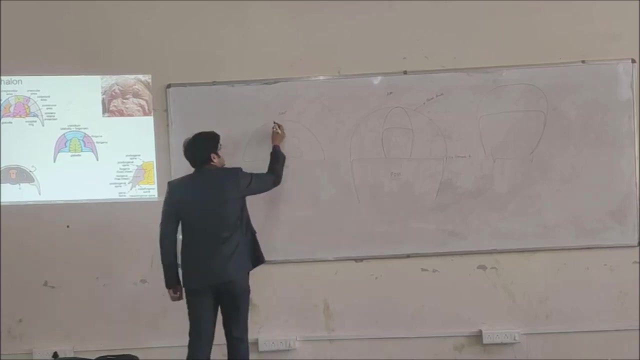 because these were the zones where the shell or the carapace would open during molding. So if you look at this zetalon anterior side, this is the posterior side. Let us make the glabella a bit integrated. Now the facial suture. 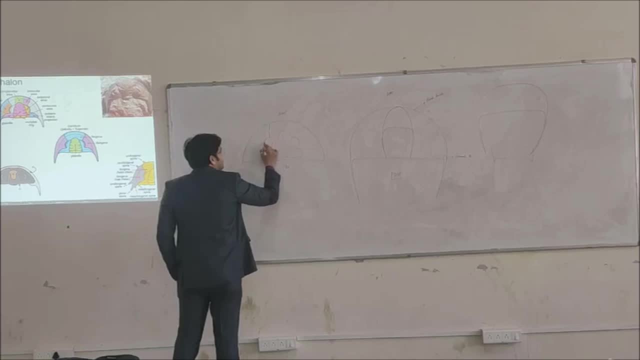 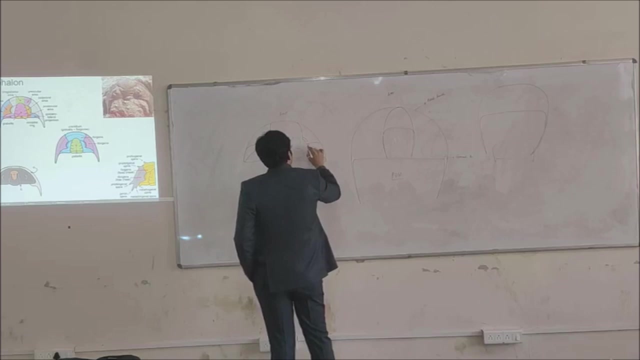 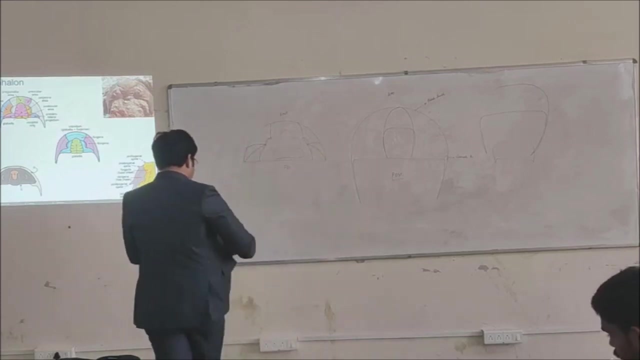 might extend from the anterior side, go and touch the ocular platform of the eyes and then may end at the lateral border, at the genal angle, or at the posterior border, Lateral border, posterior border, So the facial suture. 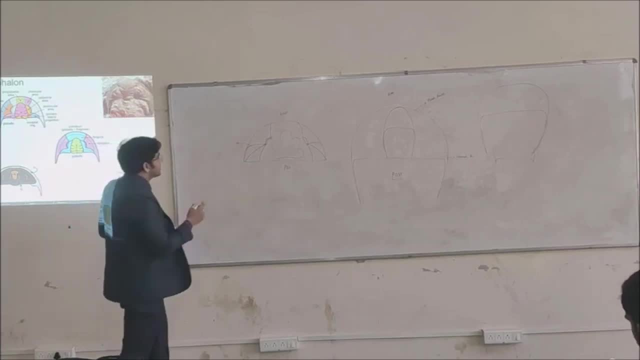 you know what is a suture: A line that joins two surfaces. So the facial suture which ended at the lateral border, leaving a very smaller area here It was called as properion suture, The one which used to end at the. 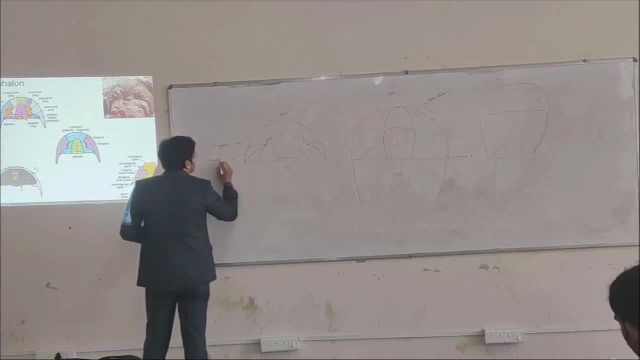 genal angle gonatoperion suture Gonatoperion And one which used to end here on the posterior border. it was called as occius properion. Since this is the facial suture, we are talking about means. 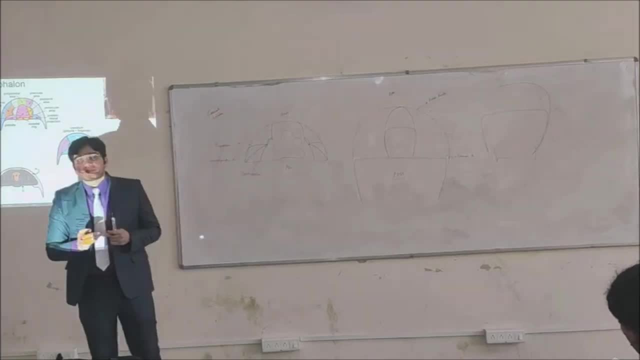 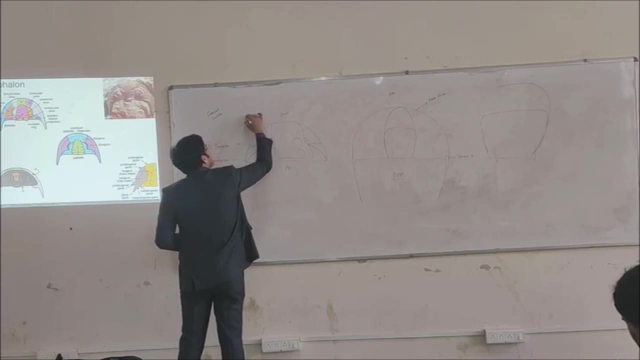 it had to join two surfaces or not Two surfaces, right? So what are those two surfaces? This one, This is called as free cheek or livery gena, And this portion here, both they will be called as fix cheek. 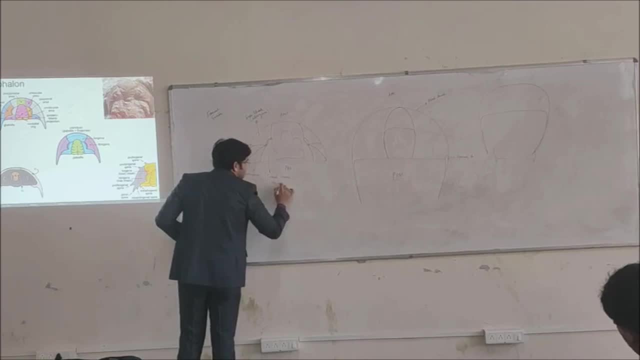 Or fixy gena, Fixy gena, Fixy gena As the sutures they change. as the facial sutures of trilobite change, the size of livery gena and fixy gena would also change, Yes or no? 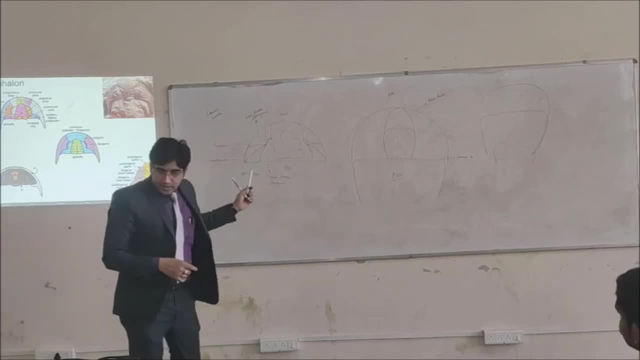 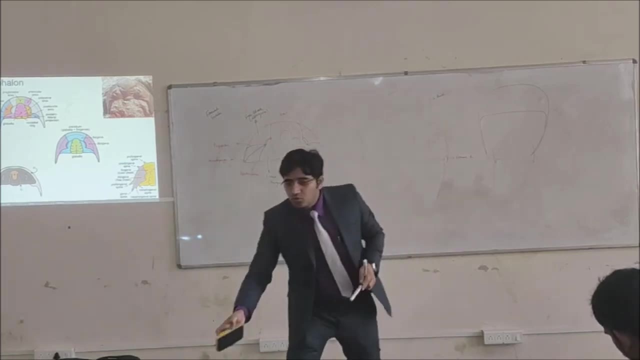 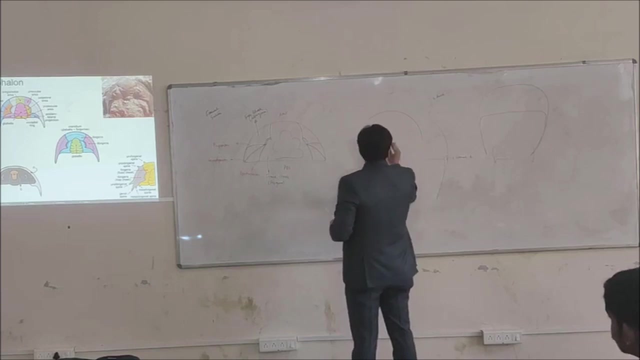 So what was the importance of this facial suture? That when the trilobite had to do a podiasis, it would do something like this. So this is the cephalon and this is the facial suture. 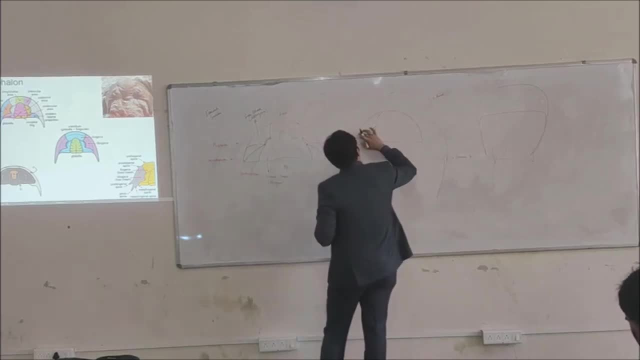 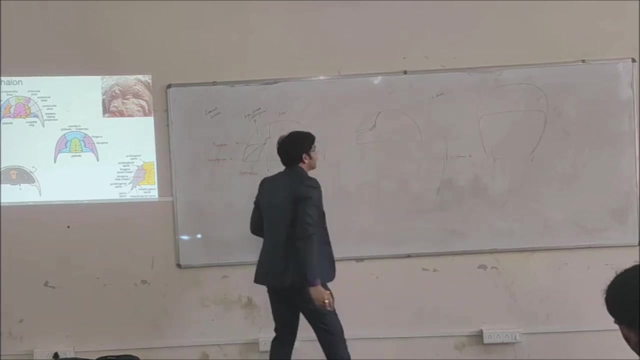 So why did a podiasis used to happen? This would be the montanus. Yes, This portion would open up. This portion would open up. Now, will it be like this, Or will it be this, Or will it be like this? 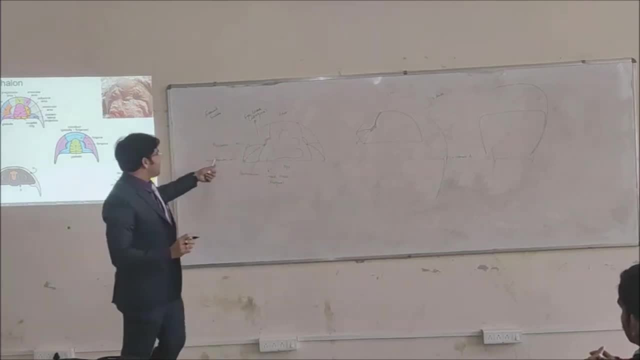 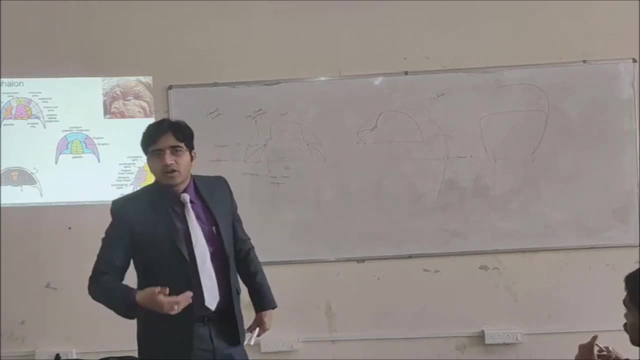 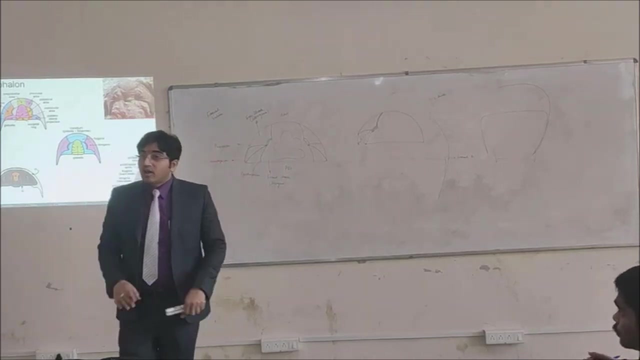 It would be depending on the type of facial suture. Propeller oldest- this was the oldest facial suture. Then doratoperium and distoperium they came into existence. That was also the old style Free cheek. 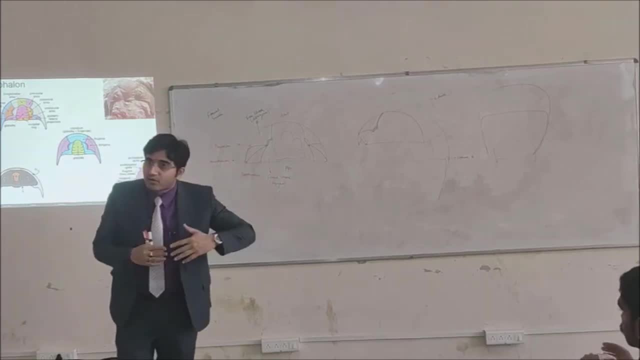 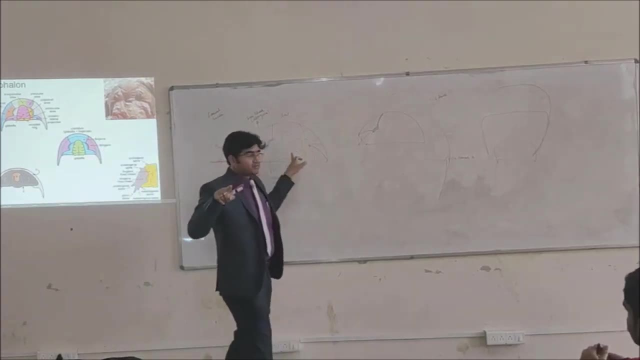 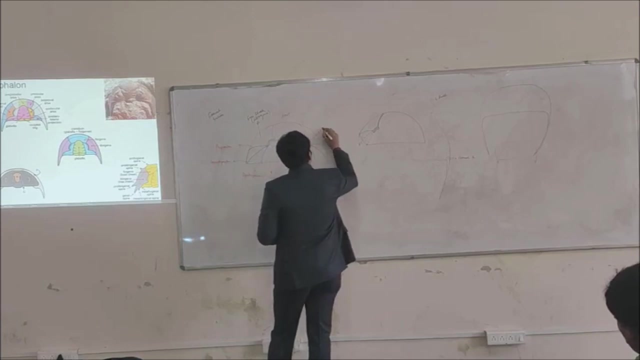 see this free cheek which used to get liberated open The eyes. they were attached to the fixed cheek, Fixed cheek. These are the eyes, The eyes they made the trilobites very unique. on them, Eyes were with several lenses. 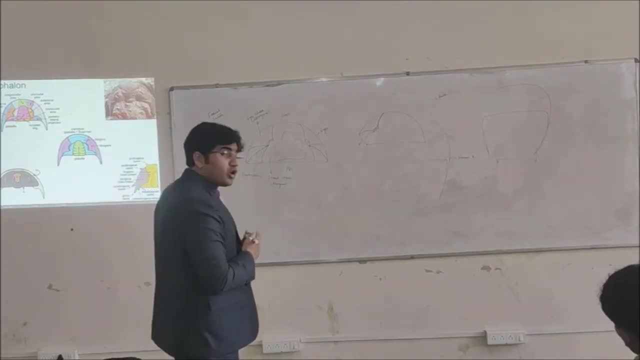 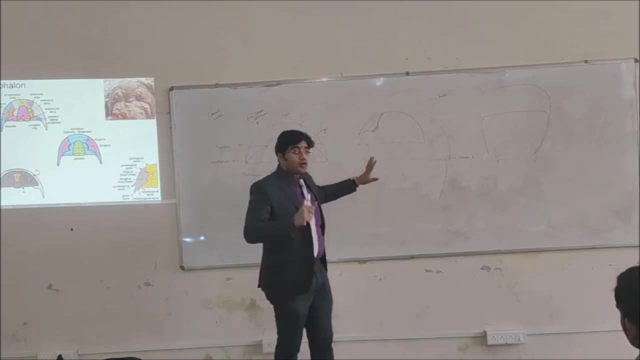 and various types of eyes. So you understood now the facial suture and its importance, How they so, if a question is asked- what are the various types of facial sutures found in trilobites, What is their function? So you will have to write that these are. 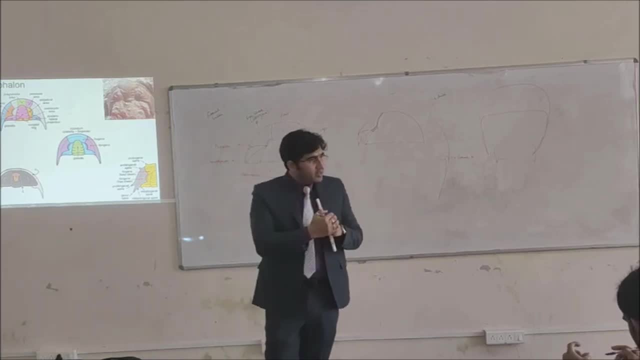 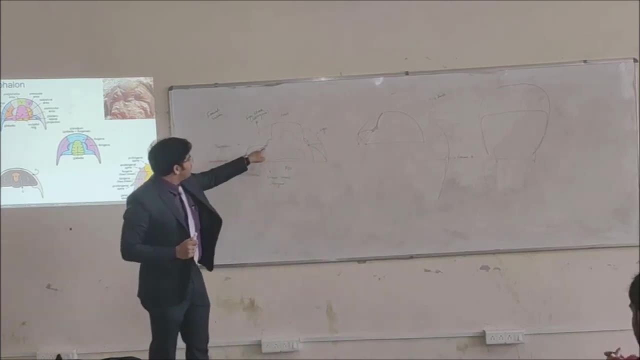 the surfaces which join the free cheek and fixed cheek on the cephalon There are three kinds Propeller: doratoperium and distoperium. So if a person had brought these three lines and leveled them, the answer will be that 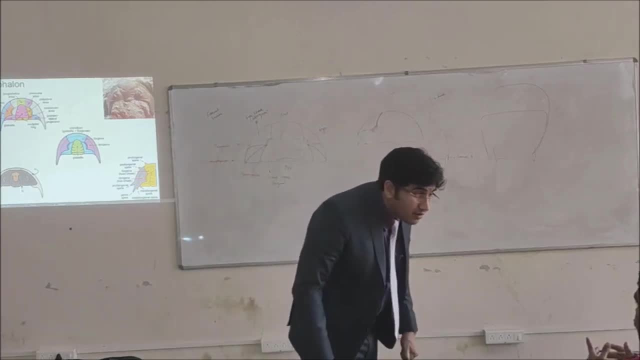 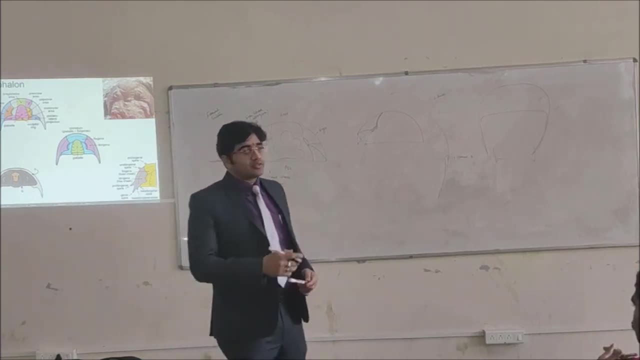 So what is hypoperion? Hypo, Hypoparion, Tell me. Hypo means These terms. where are they found? PCF, Try and find out. PCF. What do you do? PCF? What is hypoperion? 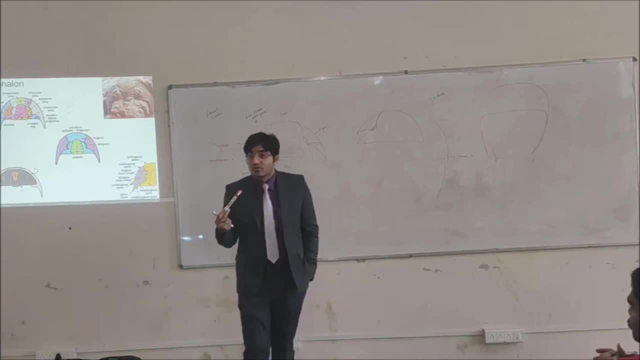 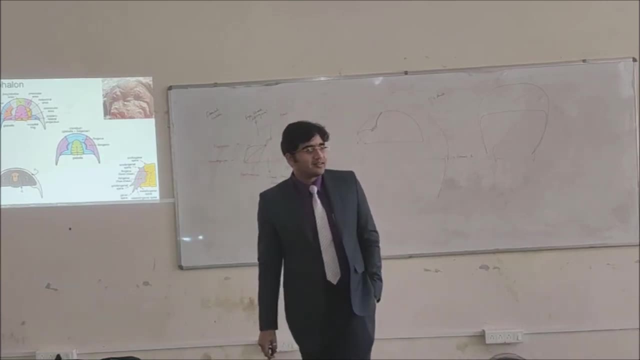 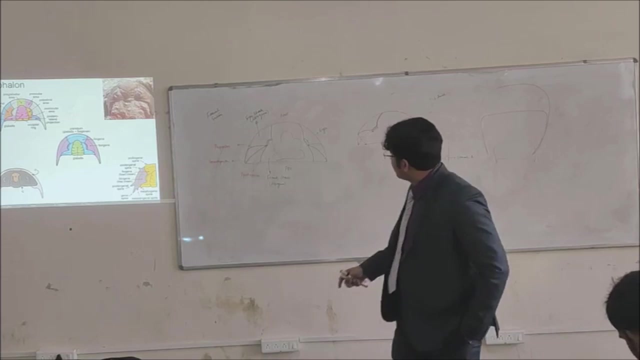 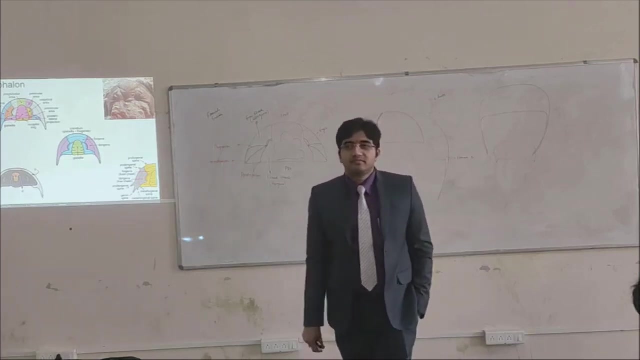 PCF? Hardly. Yes, What is your diagram? Show me your diagram. PCF- Anybody- PCF- This is not PCF. This, The one which is on the right bottom: PCF, PCF- This is PCF. 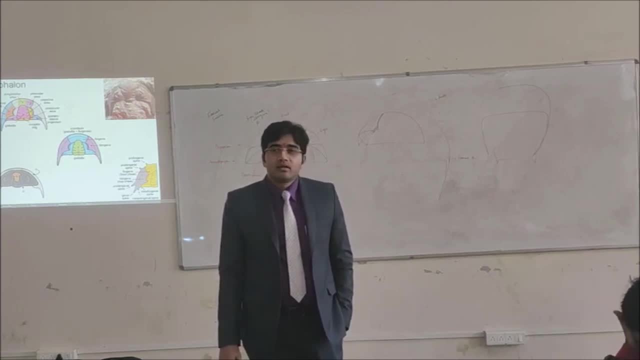 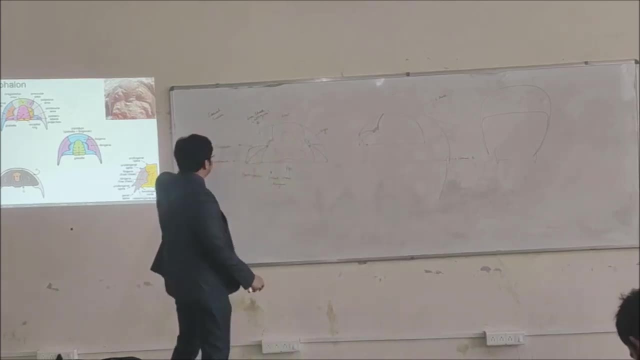 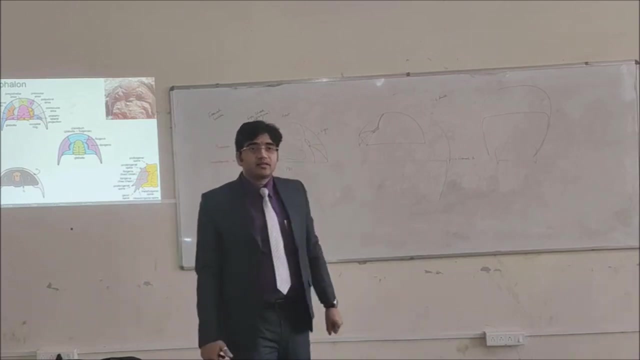 PCF. There is a I don't know What Show him. These are the three main patients. I'm going to ask you about the question about the ice. You saw that ice. ice is as dry or insensitive, but its density is lower. than a quarter. What is it? Since the water molecules become closer, the hydrogen bonds start to repel. You know that the density of hydrogen depends on the number of molecules that come close to it, But when the hydrogen bonds start to repel, the density of water molecules decreases. 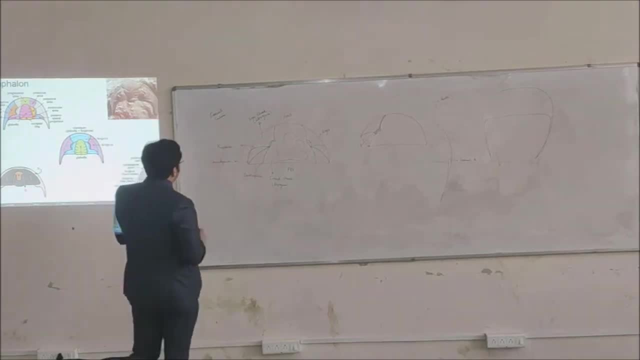 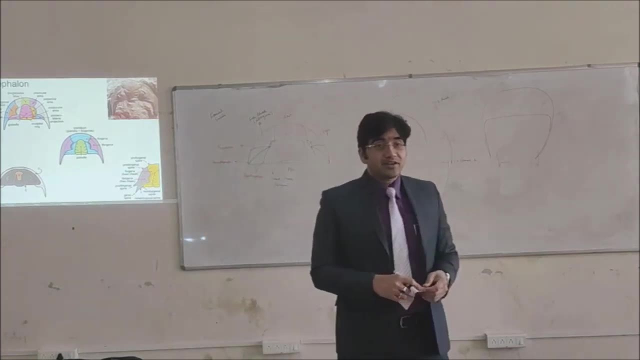 Show me the diagram. So we have these three facial sutures. There is one more protist? Yes, protist. Tell me Diatom. Diatom is a protist. Who told you that? No, Aviva. 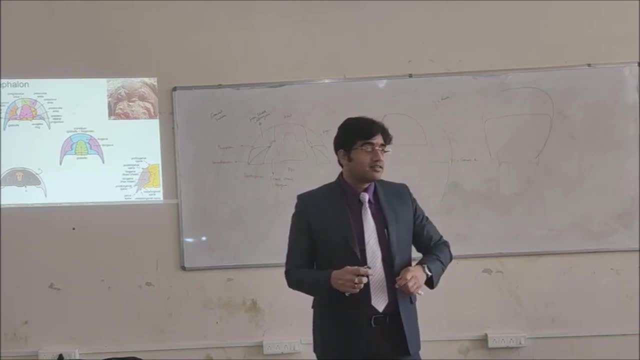 Yes And Rahim, sir Protozoa Protozoa. Protozoa Name, a very common protozoa, Plasmodium Plasmodium. Plasmodium To cure malaria. Okay, One more. 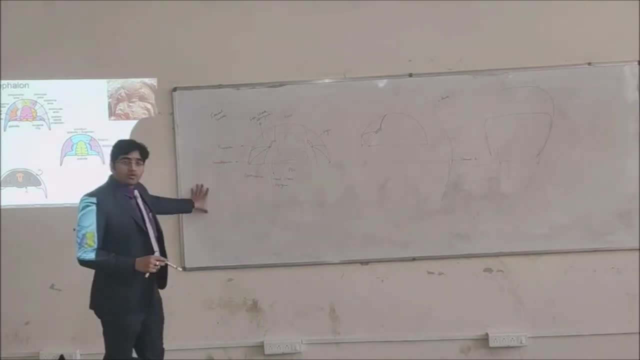 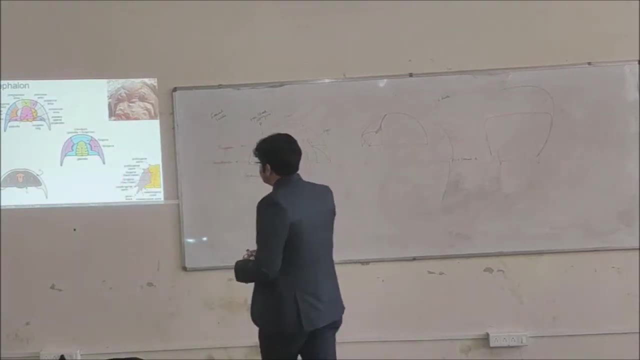 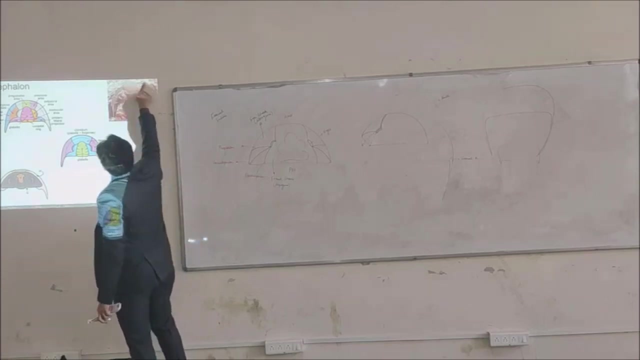 So we have come to know about these facial sutures. Yes, is that All right? So this is a care face where you can see Spine eyes and inflated glabella. This is a fair shaped glabella. Can you see that it is reaching to the anterior body? 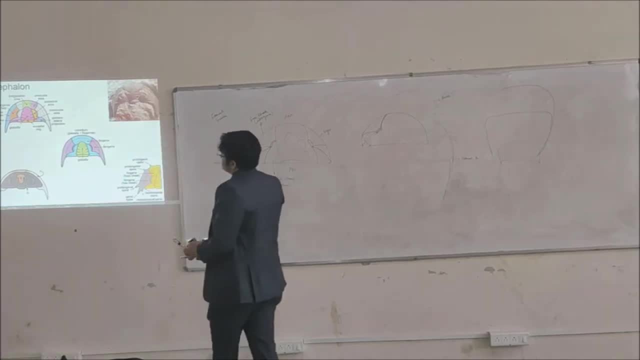 Yes, sir, All right. This portion, which consists of glabella plus fixigena, or the fixigena, is called as crinidium Crinidium, Crinidium Crinidium. Here, if you look at his right eye, you have crinidium. 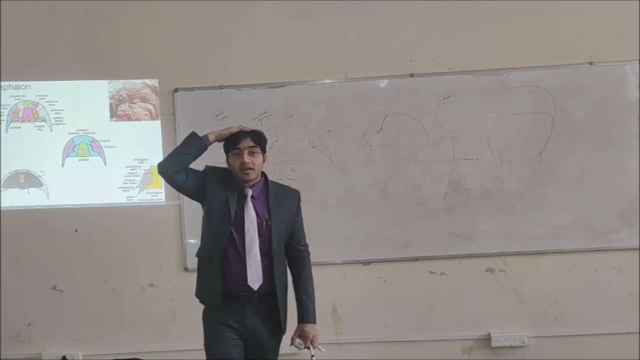 Do we have the crinidium You have? This part is called as the crinidium. Okay, aren't you Okay, Isn't it? choti chote? what are hard questions? accidentally I ask: What is crinidium? 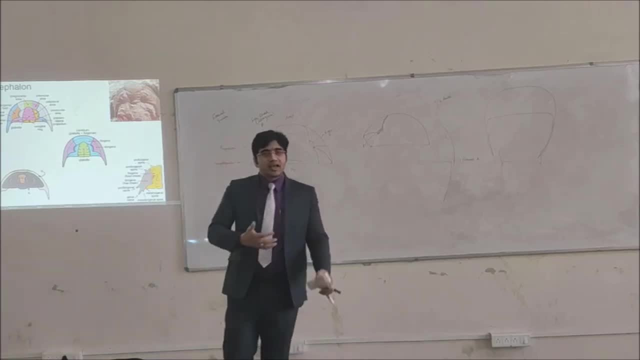 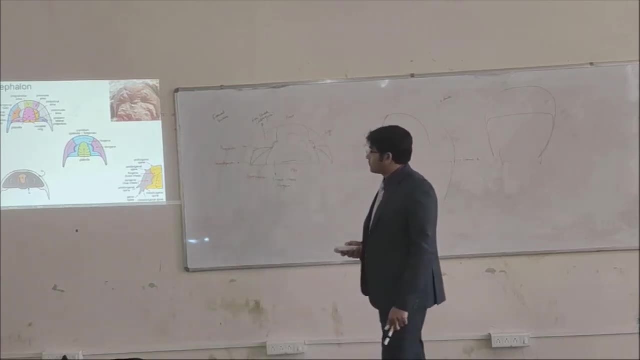 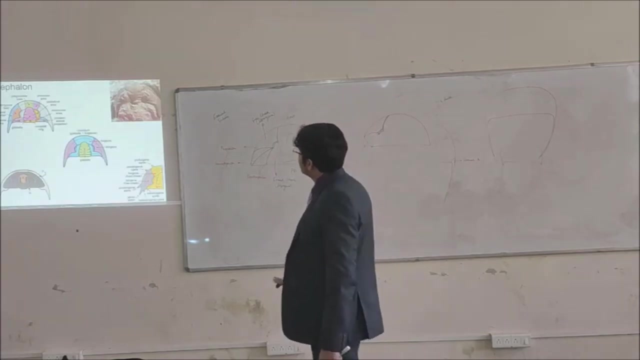 So glabella and fixigena together are called as crinidium in triglycerides. All right, Sir, wo wala bour nho konati whare raha ihme thakto E Isme haan. 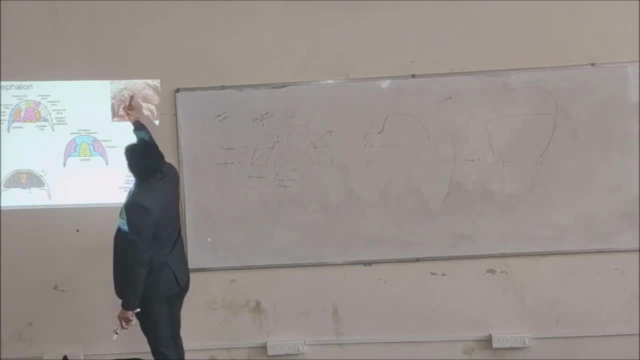 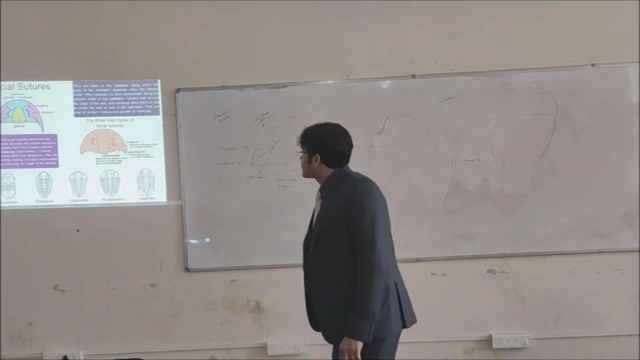 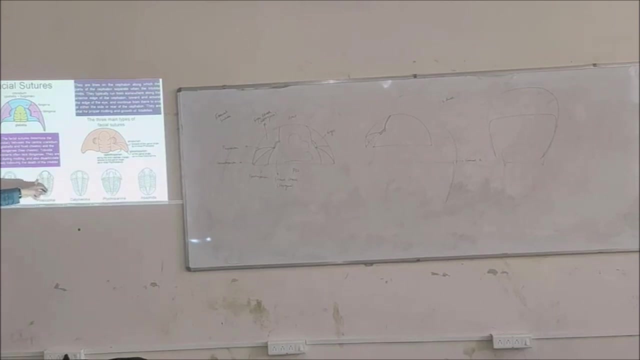 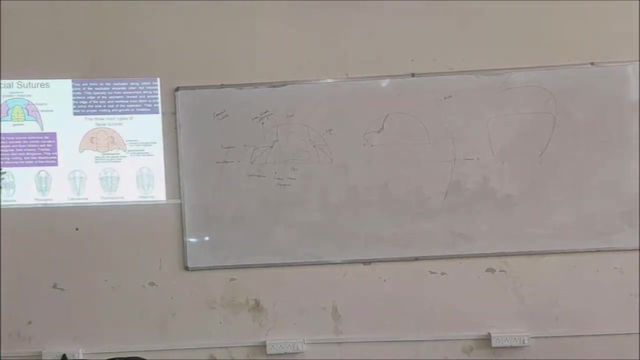 So this is what we have discussed. see, look at these different orders. EO is you know what we have discussed? you can see it this way. is it clear to everybody? any questions on facial sutures? Yes, Sir, what is the function of genus spines? Function of genus spines. see, genus spines were an extension of the shell itself, so people have thought they will have several functions either. they would have been used to scare the predators, rather, because there were trilobites which had several spines. 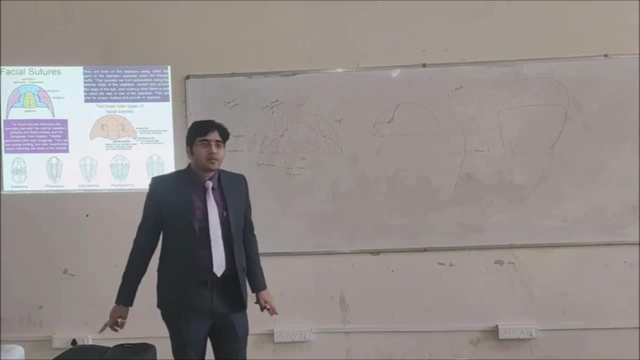 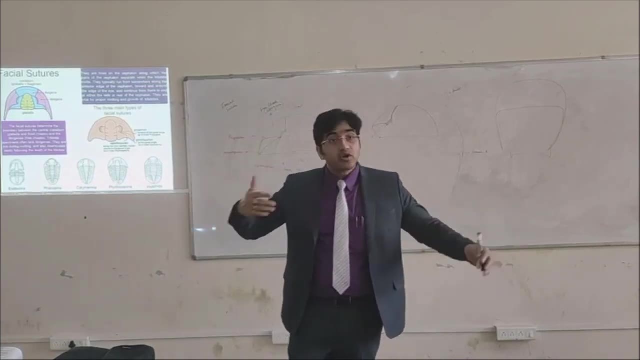 cephalic spines, thoracic spines, cutaneous spines, subcutaneous spines, all of them, so you can see if a trilobite used to you know. show those, because during the time of trilobites, daemonium was the time when jawed fishes had also come in. jawed fish 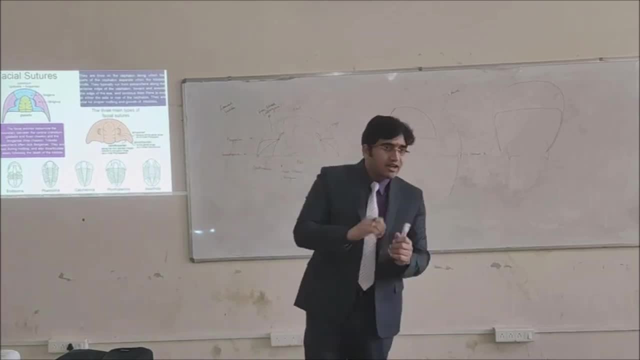 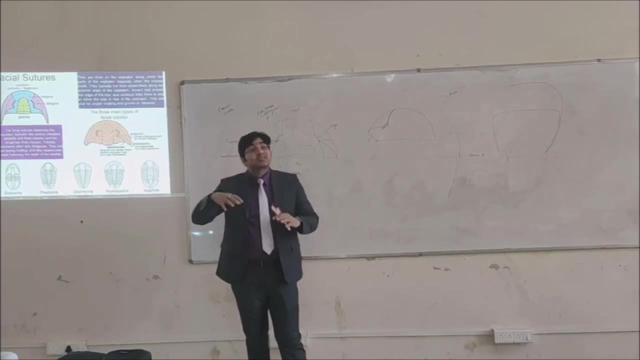 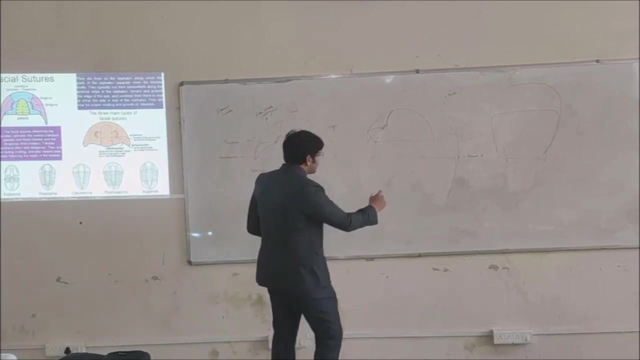 so what they used to do. they could break out these trilobites. so maybe it was a mechanism. it was a mechanism to scare the predators away, scare them away, save themselves. second, which I read somewhere that: what does it mean? 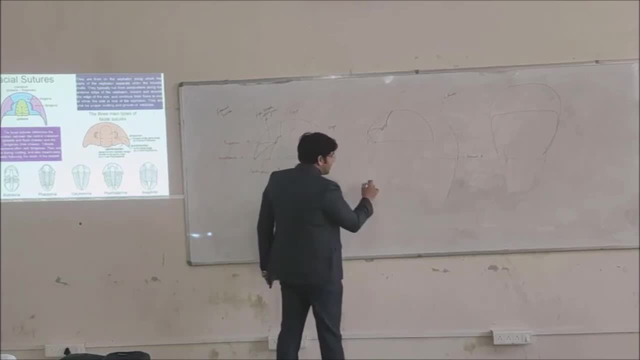 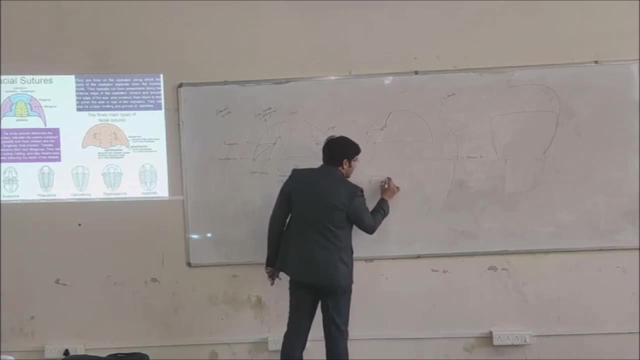 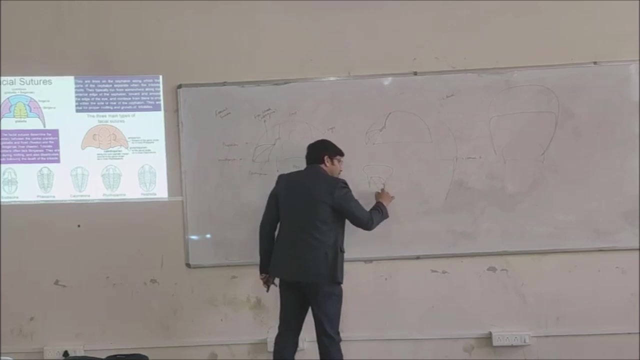 What they could do with the spines was that, if this is the soft mud and they push their spines in this mud this way, and if suppose this was the cephalon and the body they could sway in the water, the body would be chilling in it. this was acid and this was. 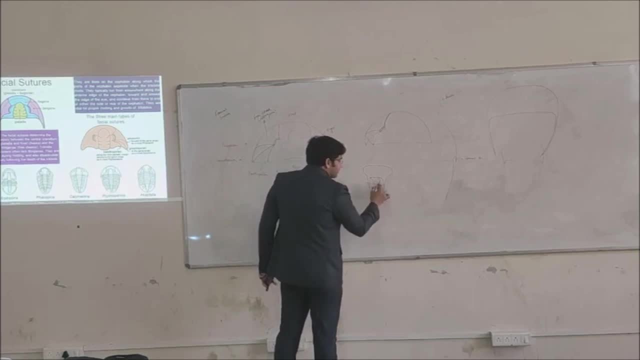 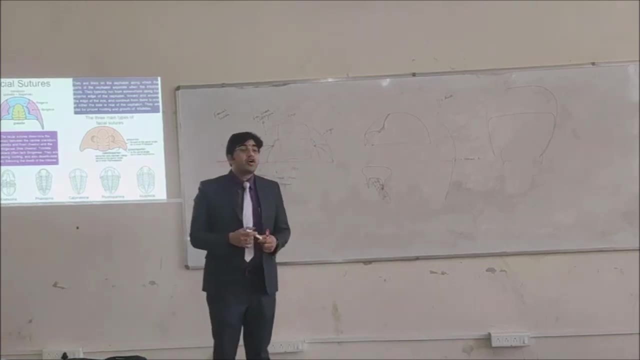 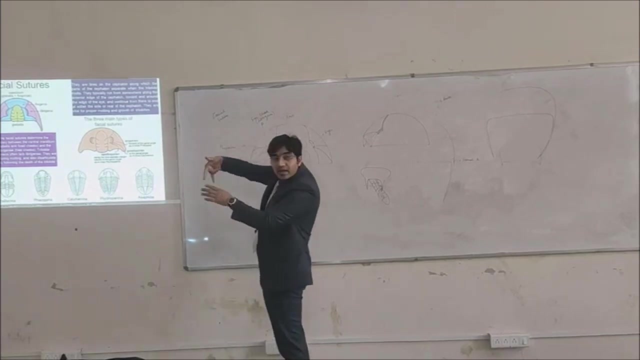 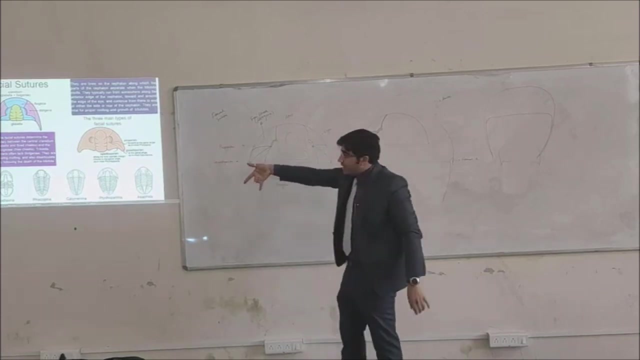 the thorax, this was the pigerium, These were like totals. So if this is the cephalon and this is the spines, push it inside the body. is this the thorax and the pigerium? is this? go inside, it would provide buoyancy and they would. 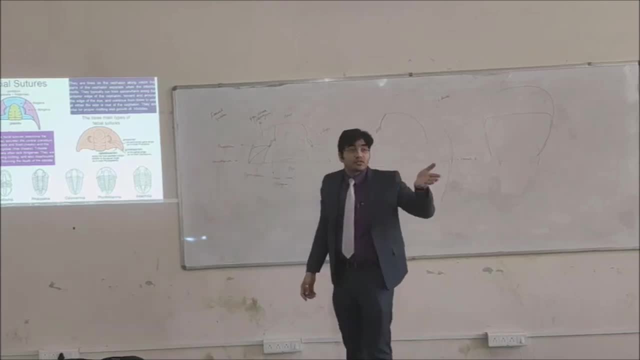 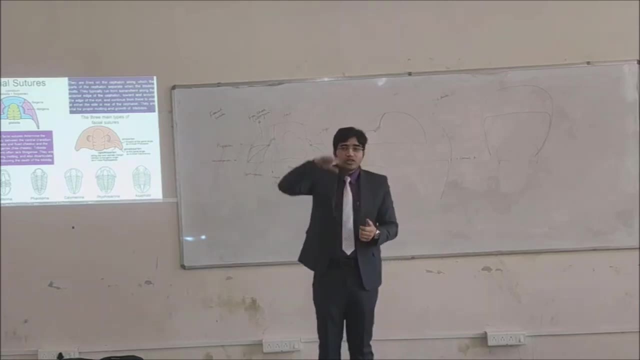 flap the water, because the colloidal substances which are there in the you know, which are floating in the water, they cannot sometimes be eaten that easily. You need to flap the water to release them. Okay, So what happened now? 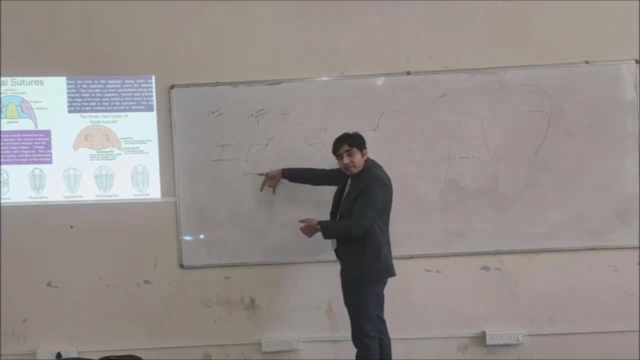 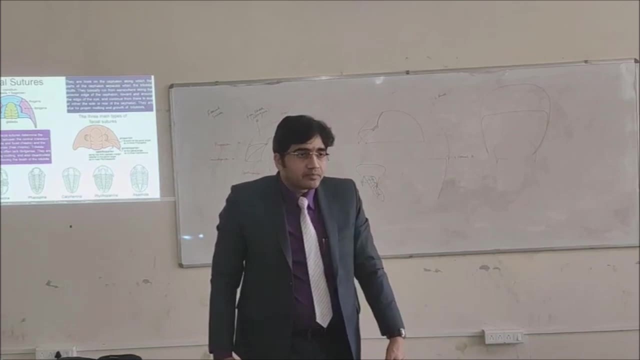 They went inside like this and they used to flap it. So what would happen? They could get the food, This, this is one explanation which is given for the function of spines. Okay, So it was kind of survival mechanism- and then for feeding themselves. 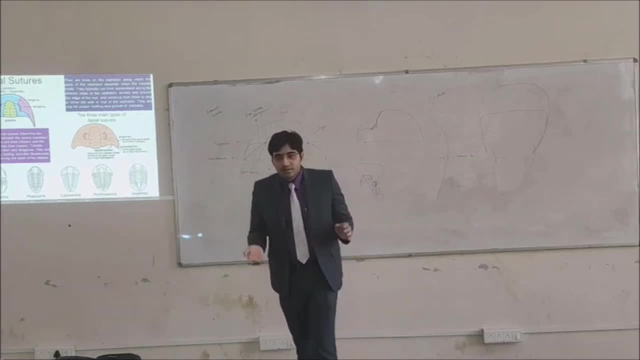 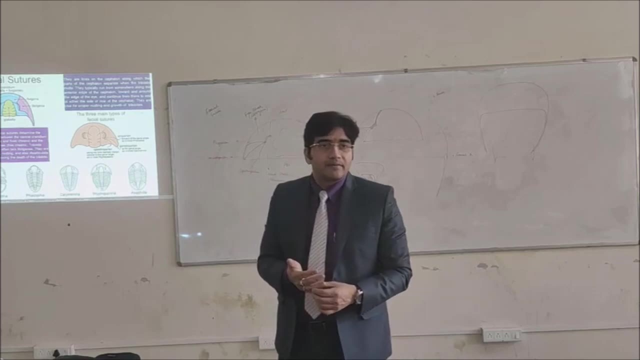 Thus spines could have been used. Okay, Sir, this frog, what is it? Oh, Yeah, Yeah, Prawn fish, Prawn fish, It is not a thalopite. It is not a thalopite. 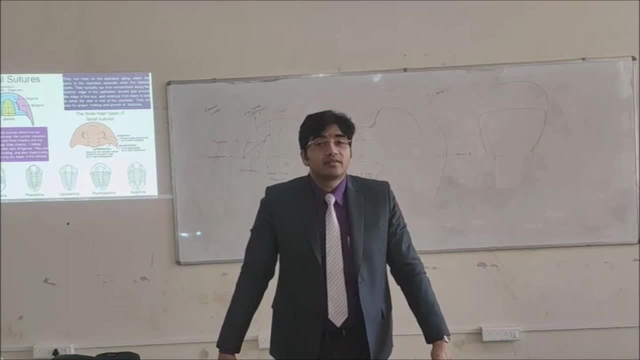 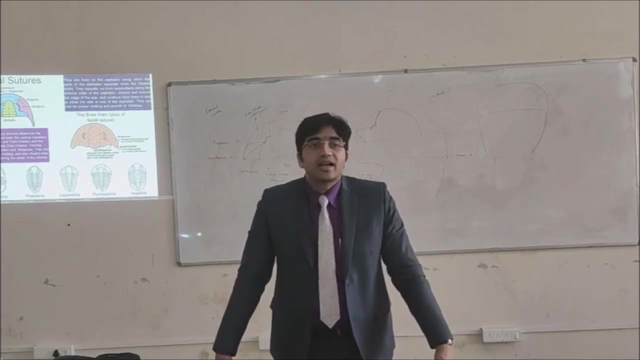 But which filament belongs to All the organisms which have segmented body? belong to the phylum arthropoda Scorpene Insects, All the things which have segmented body is the class insecta of phylum arthropoda is the biggest class in terms of population. 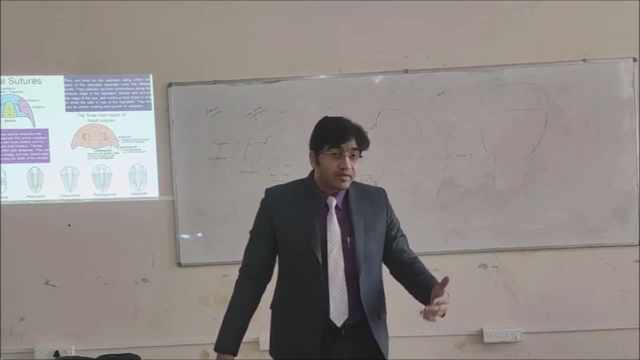 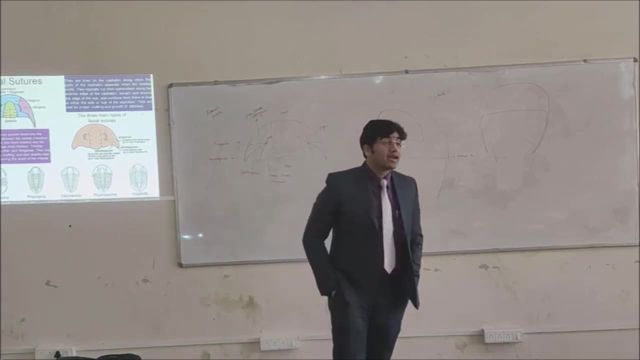 Yes, There are several insects about which people do not even know today. Okay, Sir, how do you think pterobites had no eyes? Which Agnostics? yes, They were facing a lot of troubles. How did they survive? 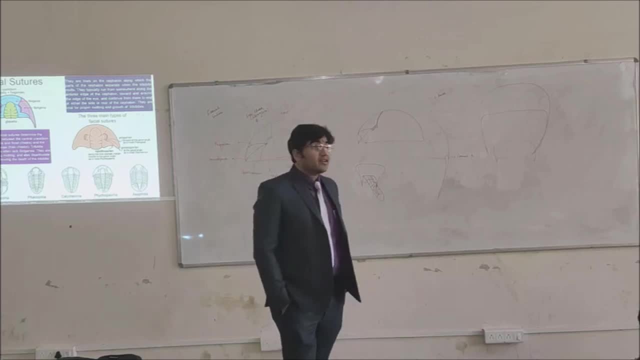 We can guess that to avoid the troubles, they lost their eyes. To avoid the trouble, Let us make up a story That the pterobites, the first pterobites, had eyes and they were shallow marine. They used to live in water. If some organism has eyes, it means that it would remain where the light would come. It needs light to use its eyes, or not? Okay, It means that they had more chances of being preyed upon If they were living on the surface. they could eat their predators. They were also there, They could eat them. So probably to avoid these predators, they changed their habitat from shallow marine and they moved. They went to the wintry portion, They went to the deeper part. Now, the deeper part doesn't mean 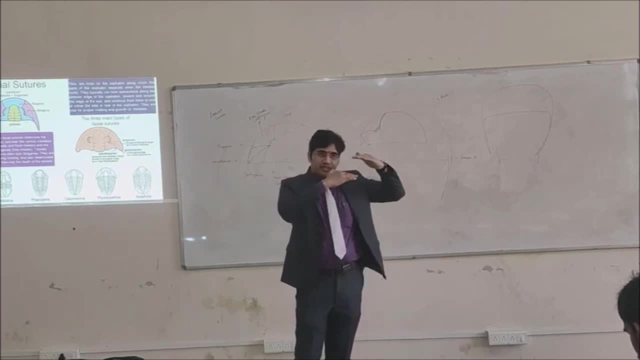 that they are 4,000 feet deep, As yesterday I had told you. if, even if we have a shallow sea, the surface of water is the shallow portion, the ocean floor is the deeper portion, Right? So maybe they shifted from. 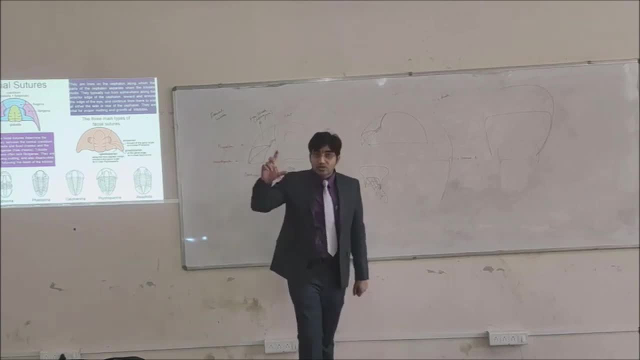 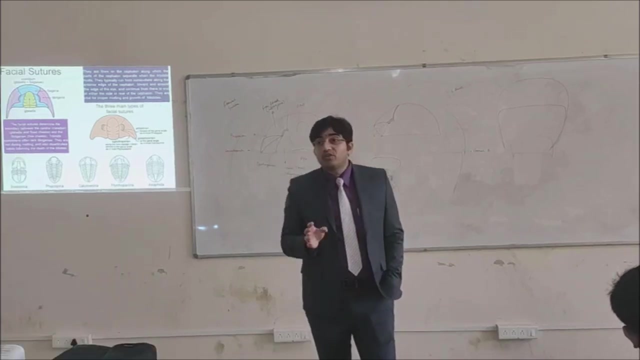 photic zone to a photic zone. From the photic zone, they went to darkness. If they went to darkness and adapted their lifestyle for that place only, why would they need eyes, And what this adaptation was? Probably to protect themselves from their predators. 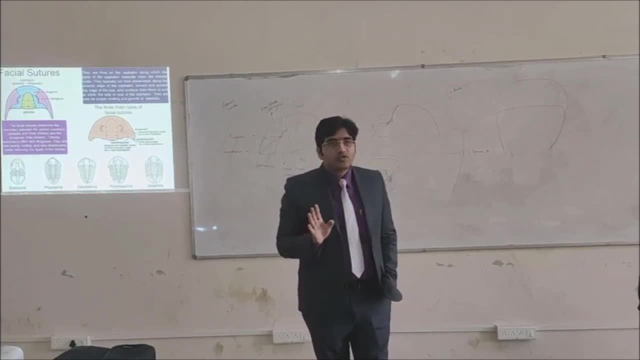 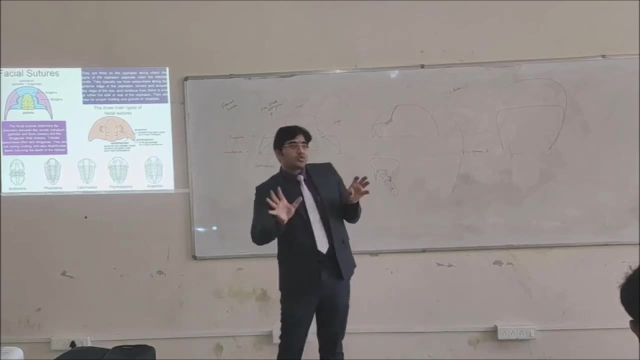 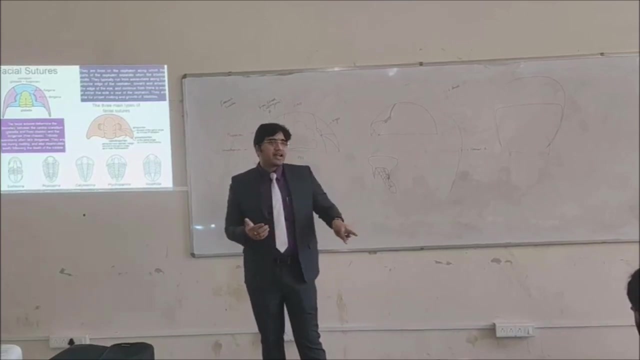 Are you following? Probably to protect themselves from the predators. So they lost eyes. But it's not that one group will give eyes to other group. only There were several other groups which were being evolved. So if the second order, agnostic. 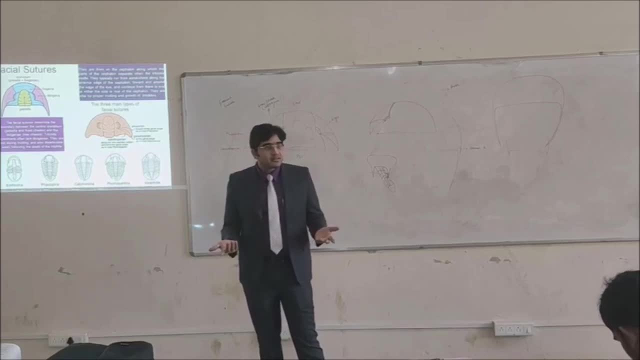 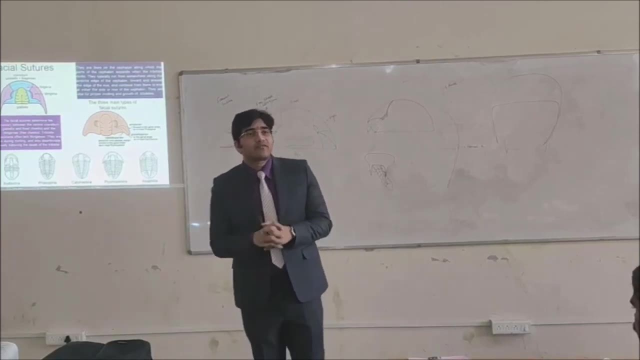 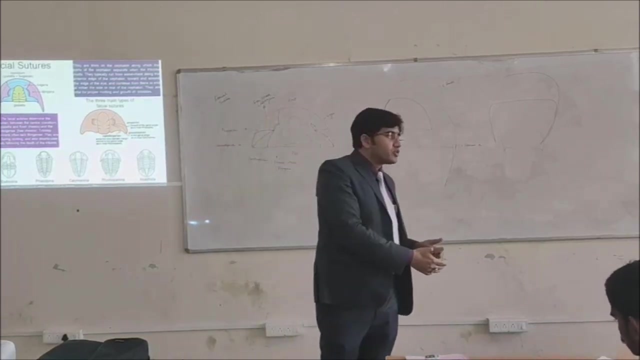 will not have eyes for the predator. then they will have to use their hands. But this is the. this would be the best way out to protect themselves from predators. They would have lost their eyes Because they shifted from well-lit zone photic zone. 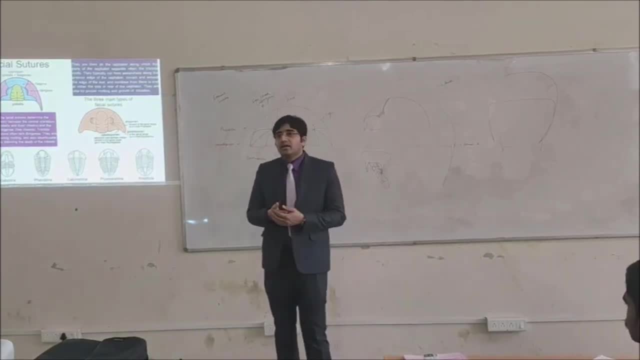 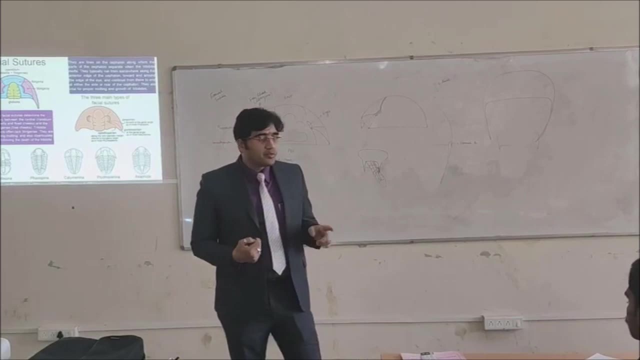 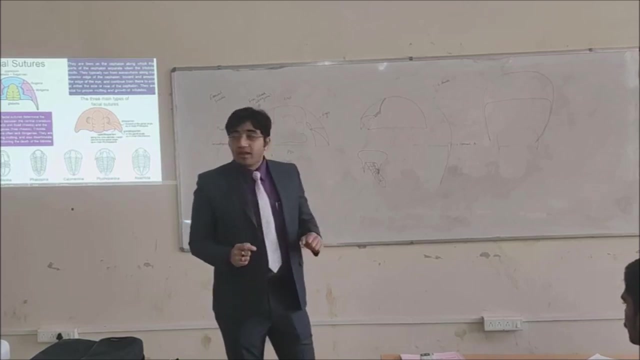 to a photic zone. Why we lost the tail? We are a descendant of the monkeys. only They have tails. We do have a tail bone. Why we lost the tail? Because we did not have the use of the tail. Can I enter this classroom? 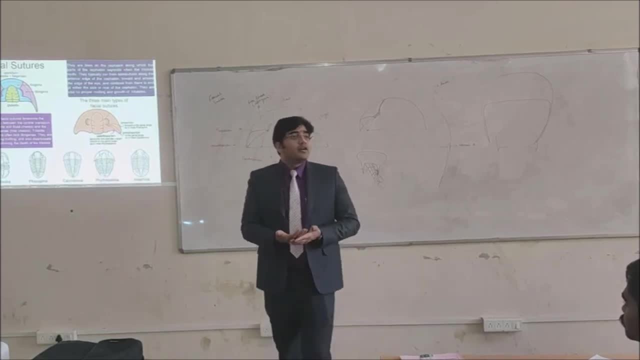 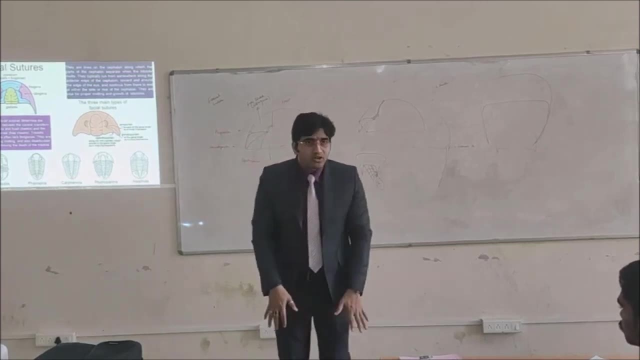 by opening this door by my tail. No, it is of no use to us. Why did the bipedalism? you know the chimpanzee or the gorilla? they are bipedal, they can walk on two feet also, But why do they always? 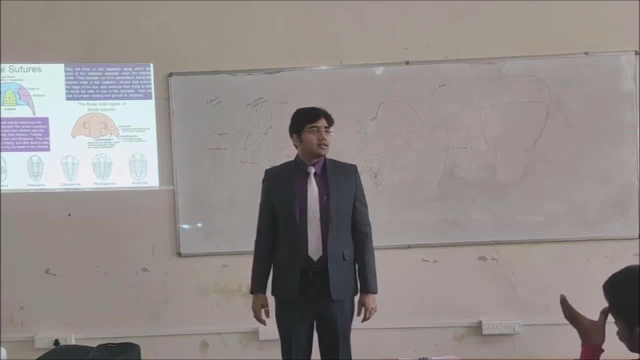 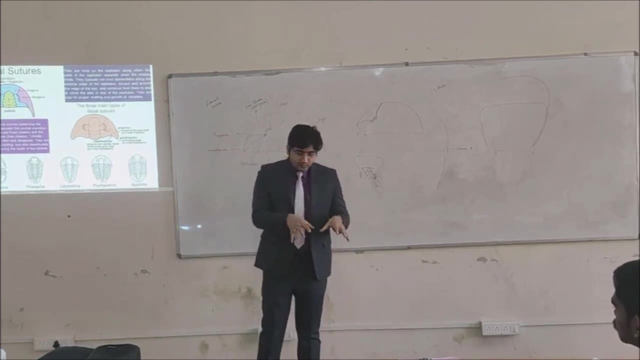 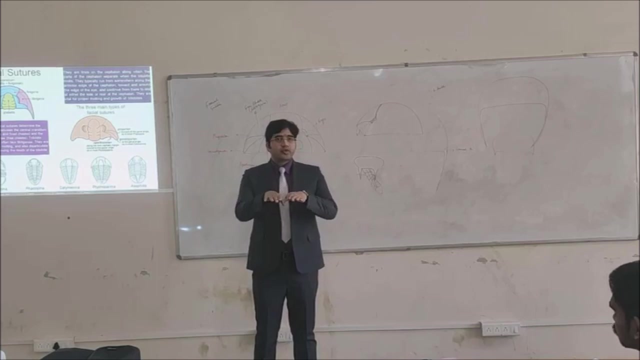 you know they cannot walk straight like us. This is an evolution, Especially in the human race. you will find that the human beings- they were bent and slowly they became straight and started walking on the two feet properly. This was very important evolution. 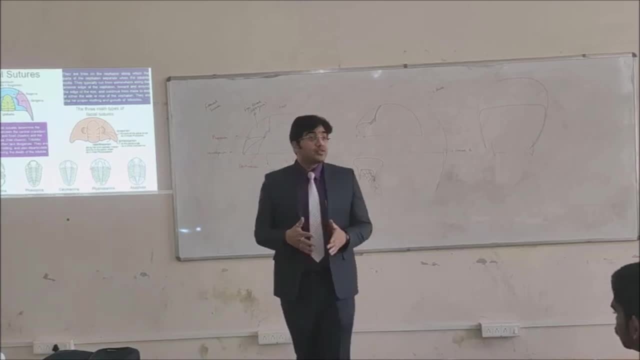 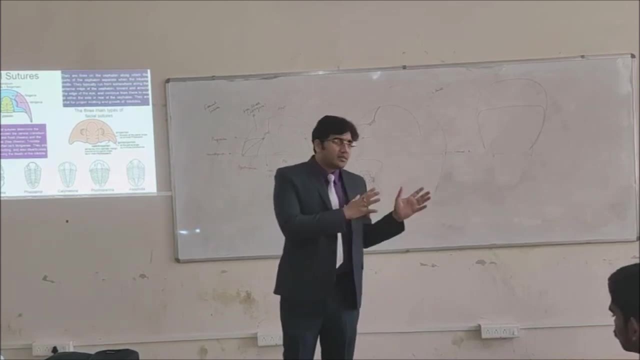 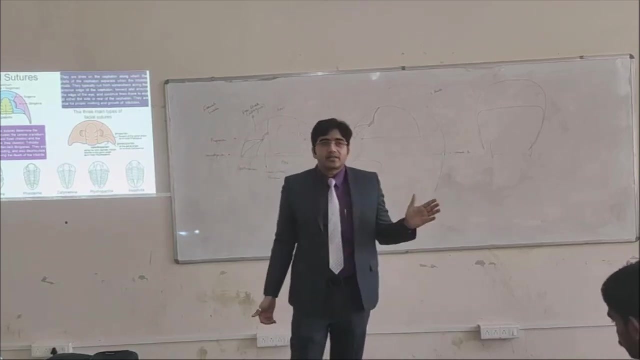 that took place. Can you tell me why these chimpanzees which either, or rather, we look very close to them, We get a lot of morphology from them? Yes, of course they are bulky, But then it seems that they are descendants. 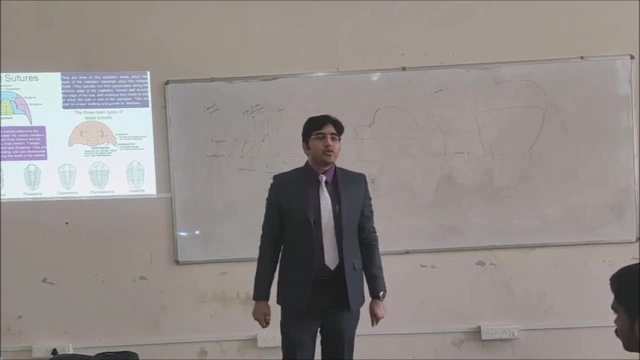 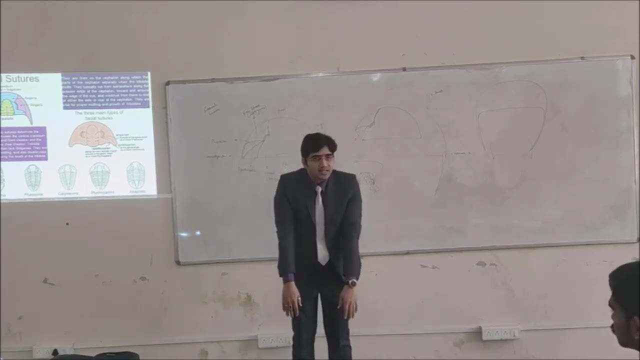 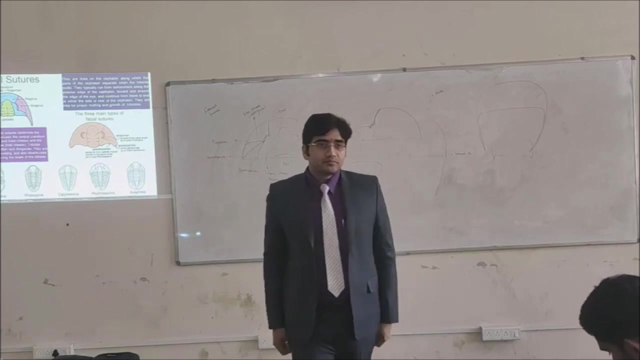 But why is it that they are like this? The limbs are longer. Yes, their four limbs are longer. If I pull one of your hands, you cannot walk straight, You will have to bend. So these are the aspects of evolution, Sir, apart from the environment. and climate. the first factor is survival. In survival, you have to protect yourself from predators. If your population ends, how do you reproduce? Apart from this, then, the speciation process. Suppose there is a geographical barrier somewhere, What does it do? It divides a large group into two groups. One group has better conditions and one has tough conditions. So either they will perish, they will die and go extinct, or they will become a better species. These are also one of the reasons where the evolution takes place. changes. So these would be the factors. So let us now move ahead to the three main types of facial sutures. This is just that we do not have any well-developed facial suture. Don't get confused with this word: No well-defined facial suture. 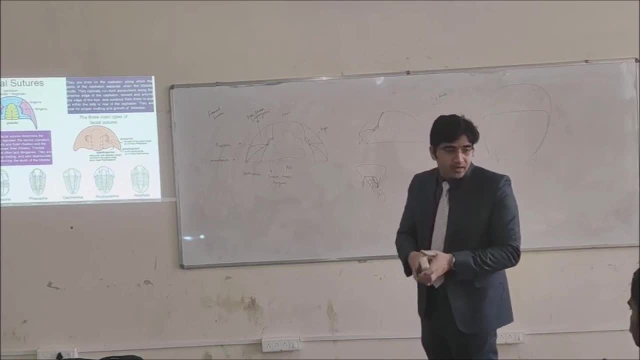 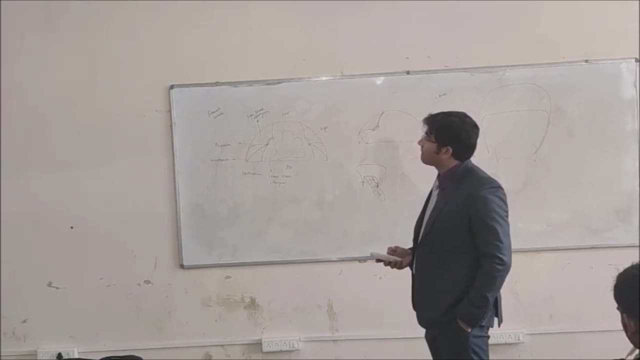 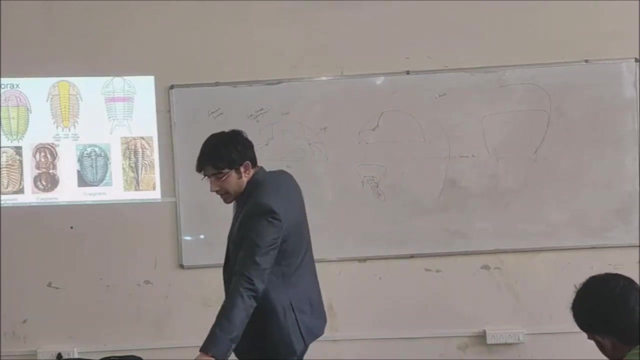 Hypotensils. yes, This is just that it is hidden. Now you understood about the cephalon, So let us now look about the thorax. The thorax may have several segments. Look at this. This is, you know, the oldest one. 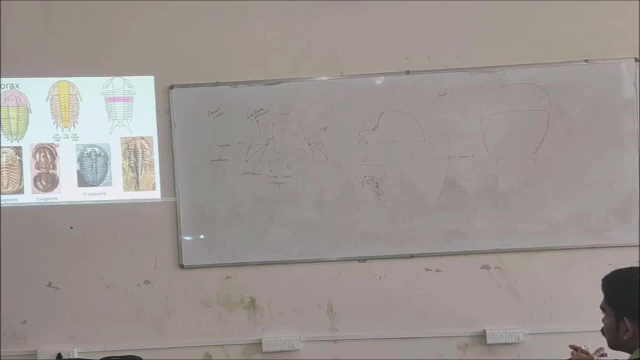 I haven't told anyone about this. There is no descendant of this. Where the thorax is not well-defined into segments, They are fused. Segments are not well-defined. Look at this. This is hypostasis. Look at this. Can you see these two? 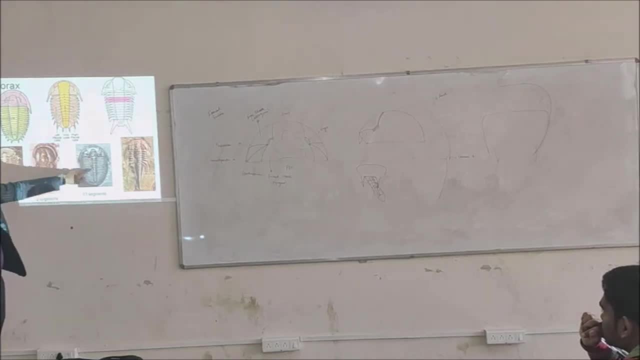 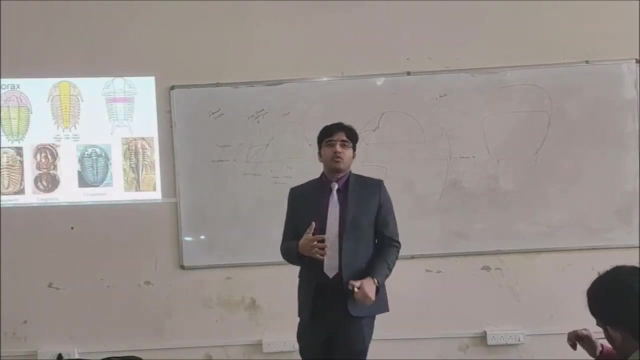 segments only Then count. it Looks like almost 13 segments and then more than 100 segments. There is this website called as phallobitesinfo. If you want to read more about phallobites, you can visit this Very good website. 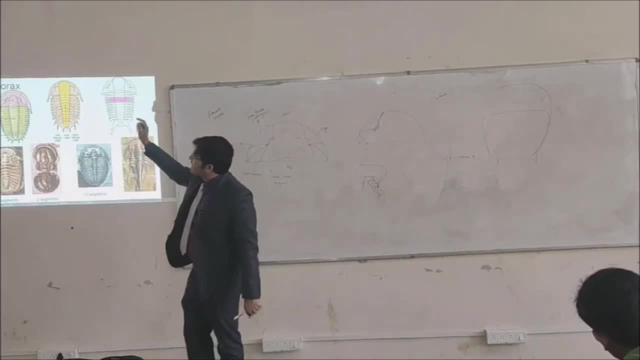 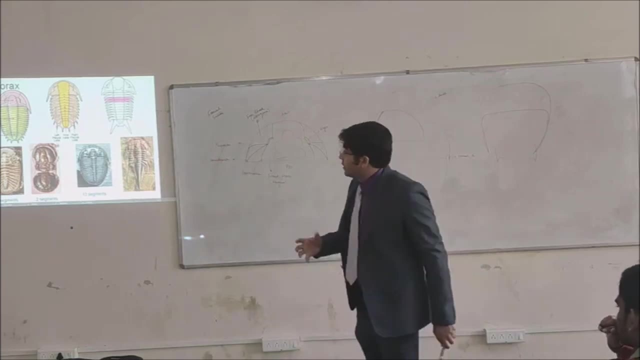 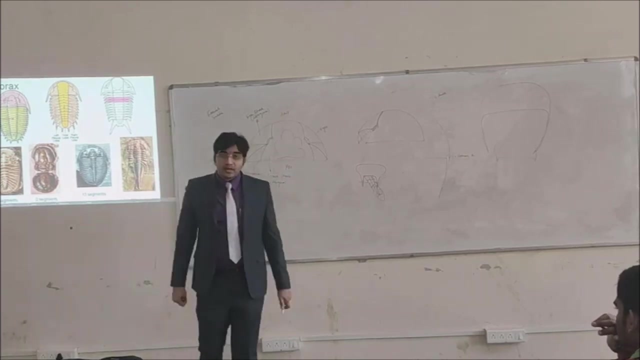 So these thoracic segments? they can range from few to more than 100.. The longer or the more the number of these segments, the slender the body would be. Are you following it? Are you following it? The lesser the number of segments. 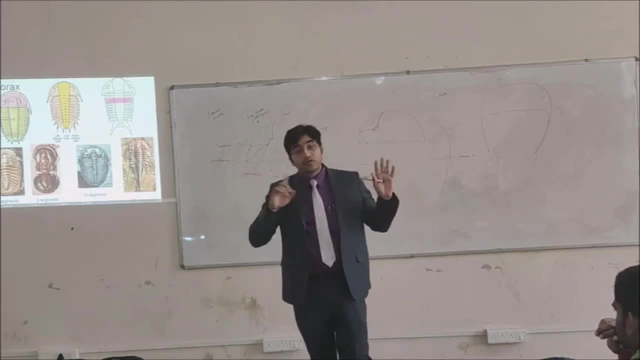 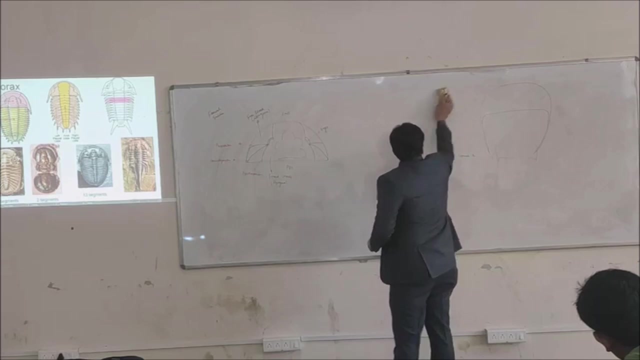 the stout or the wider the body would be If you look at paradox sites, how long its thorax is Slender body. So this this way, These thoracic segments which constitute the axial lobe, they have the puree attached to it from the two. 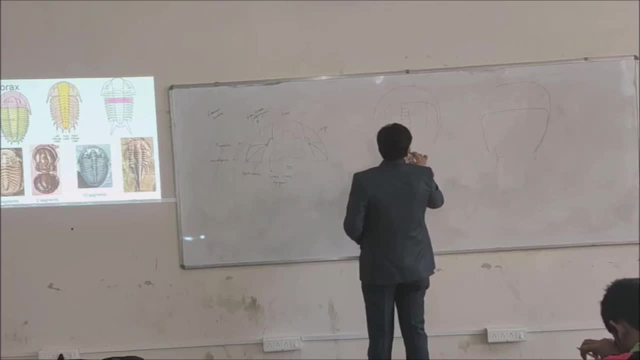 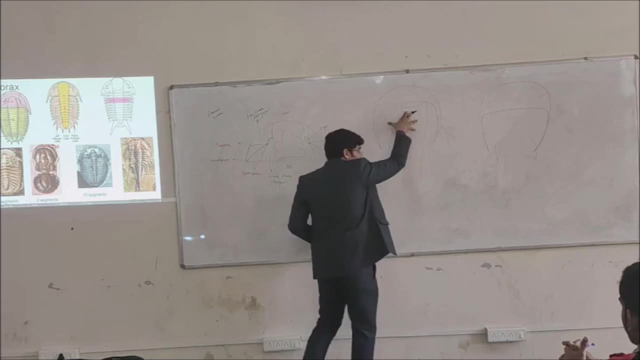 purer lobes to which are attached the legs or the feet of the tributaries. So this is the thoracic segment. See, as we increase this number, the body would become slender. Then these are the puree, The groove. Puree may have grooves. 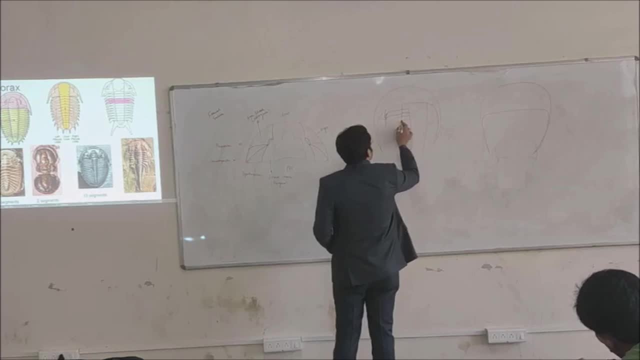 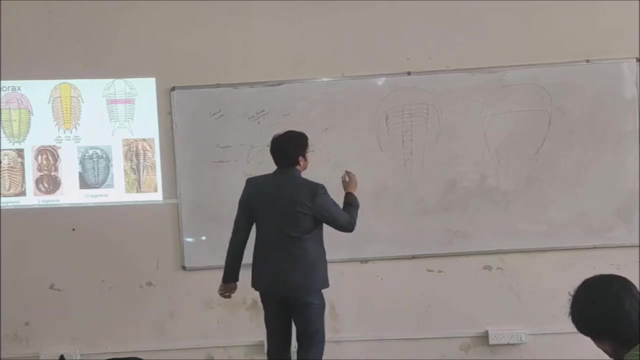 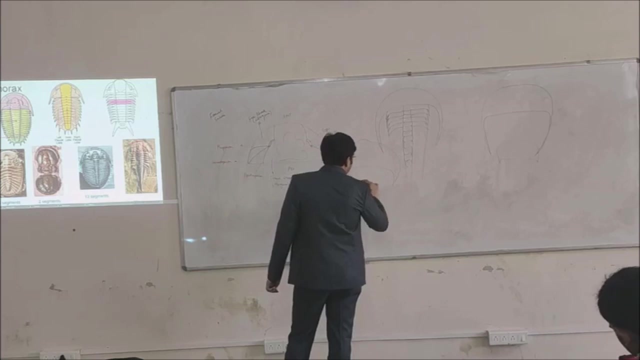 Puree may be faceted, or like a knife blade. Okay, As you can see, it is slender, All right. If you remember trident case, it had a very small, a large head shear. it had This way: 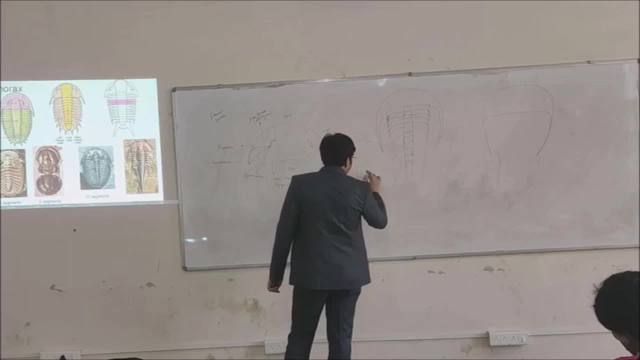 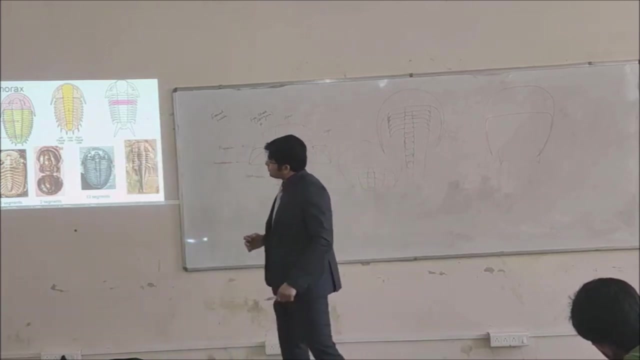 But this body was very, very small. This way, it had a fused perineum, So this was the thorax, A few segments like this, Okay, And also this example is here with you Now, if you look at this thorax. 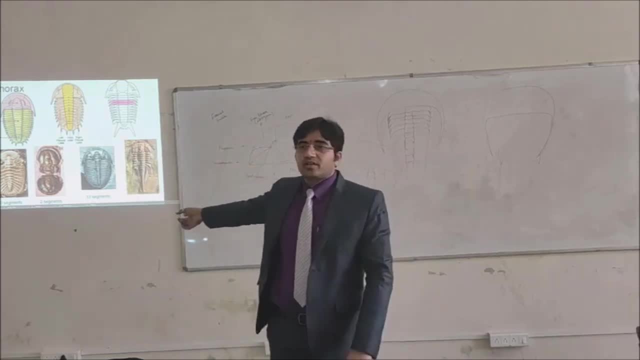 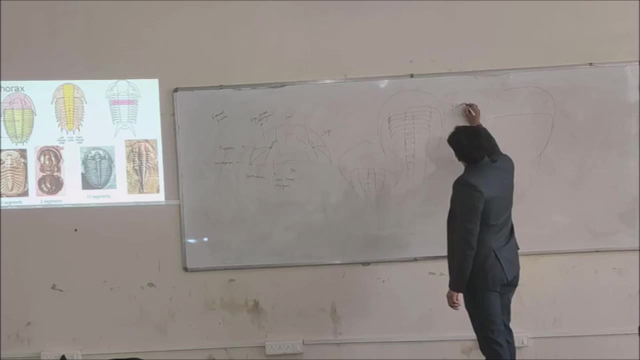 and the appendages associated with it, the puree. there was something called as Biram's foot- Biram's foot, So it used to look like this S R? U? N, And then there was a ligament attached to it. 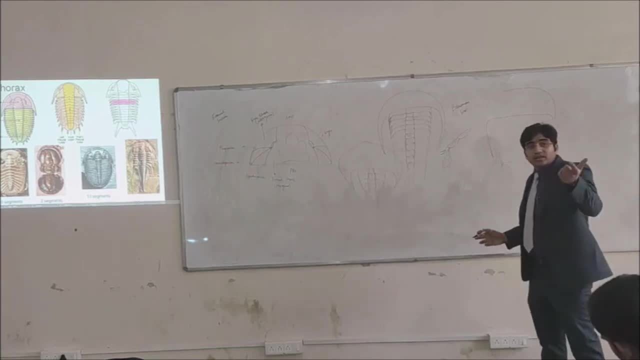 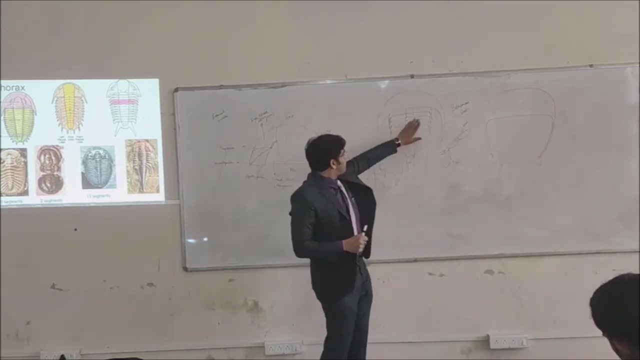 Because they were varying organisms, They had to breathe. So the foot of the trilobite had the limb on the walking part and the breathing part as well. Okay, It was attached to this puree Imagine. I put it, I flip it. 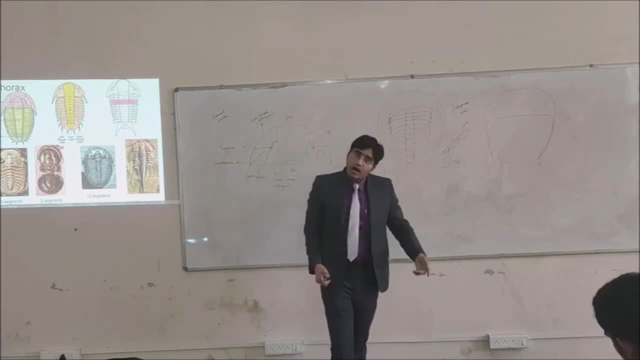 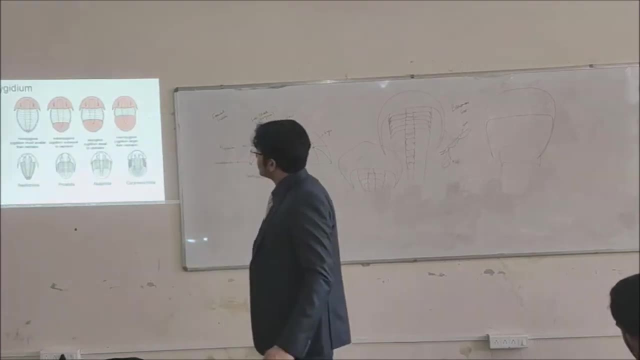 So, from here, Sir, all the plurals are there. Yes, all the plurals. They had several legs. Okay, Sir. what is the material in which the agnostos is preserved? What is the material in which the agnostos is preserved? 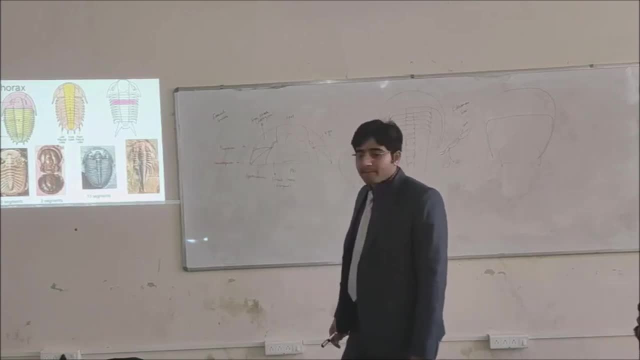 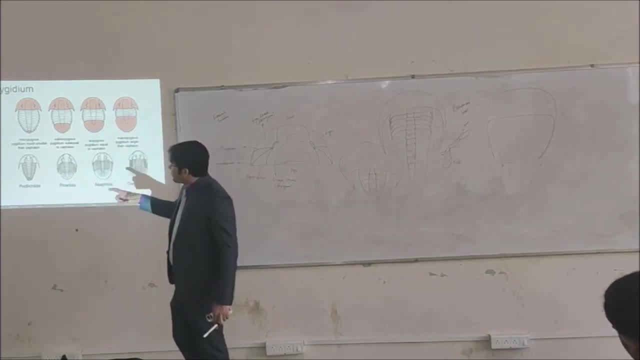 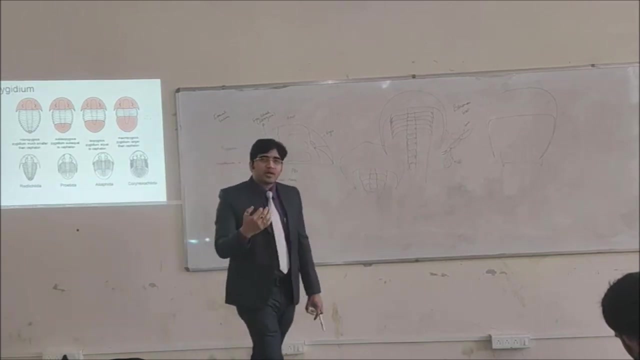 I don't know what it is. There could be some wrong body. Okay, Pigeleum. You can see here. Pigeleum could be separated into segments, or it could be made up of fused segments. Okay, Fused segments. 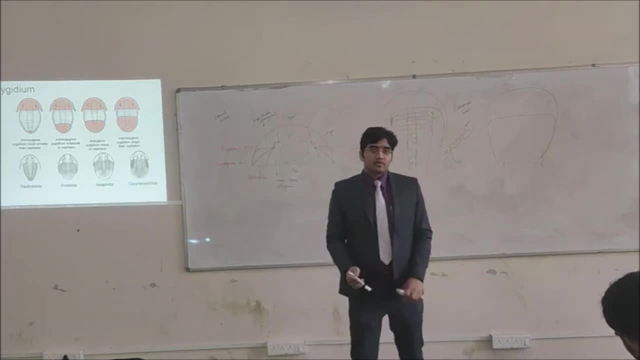 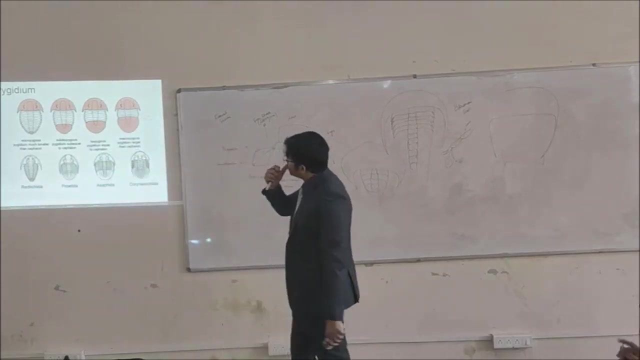 Pigeleum was made up of fused segments. So this is the basic morphology about the trilobites. Let us now discuss it here. Yes, it is a very small one, See, don't confuse with some isofagous, mysofagous. 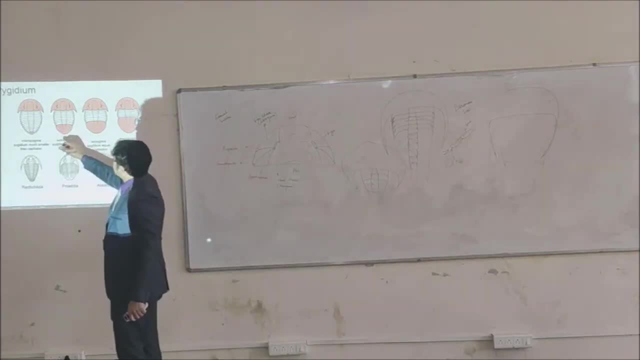 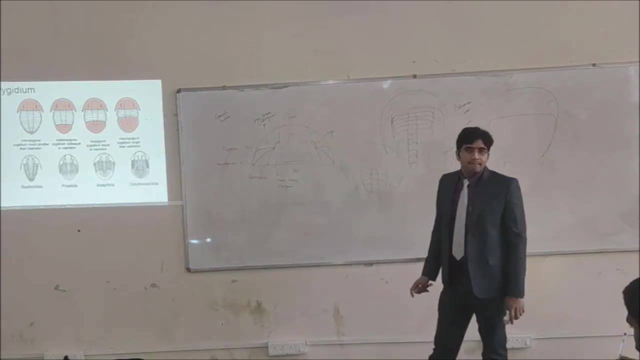 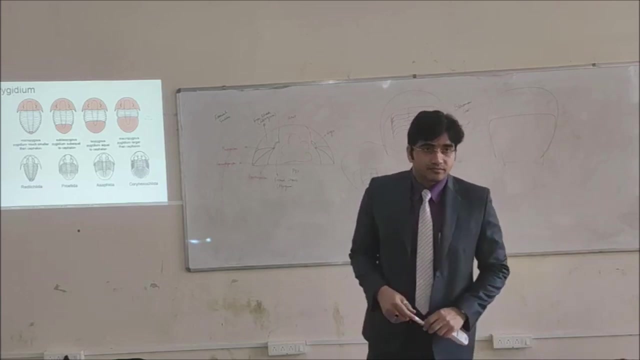 Don't confuse, Don't be confused. Okay, Any confusion. still now, Sir, what does a glabella do? What it does is it is a part of the ceplon below which is a hypostome. It was a covering for the hypostome. 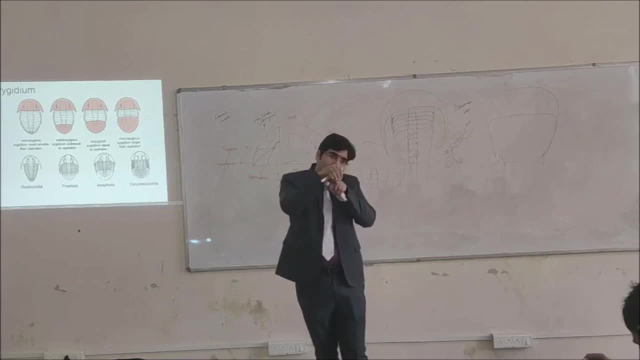 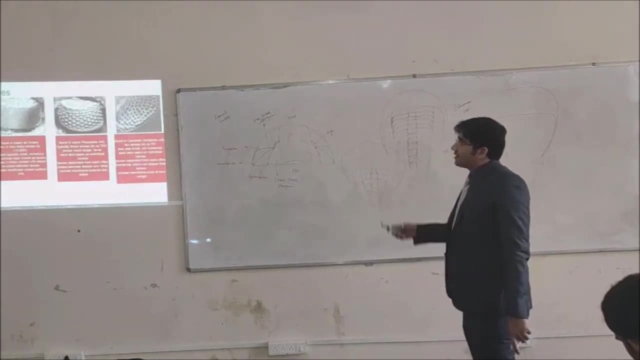 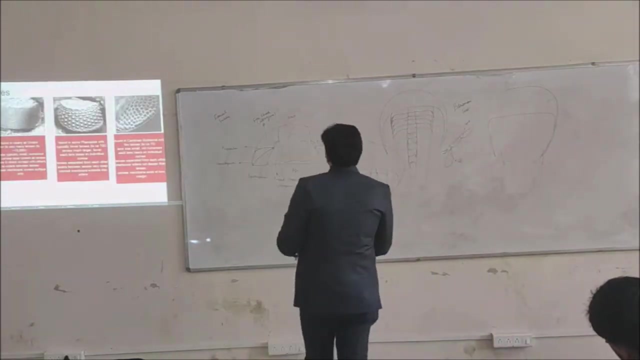 Most of the plates below are made up of glabella. Shall we move ahead? Yes, sir. Now let us come to this very important part: Eyes. The trilobites. they had eyes, And if eyes are present, it means that 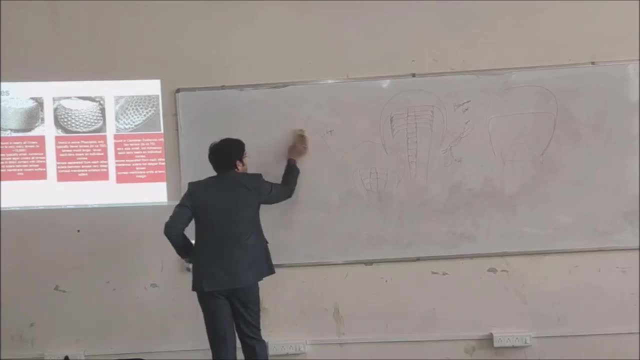 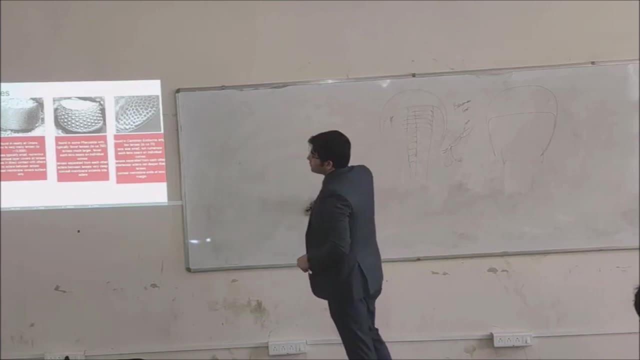 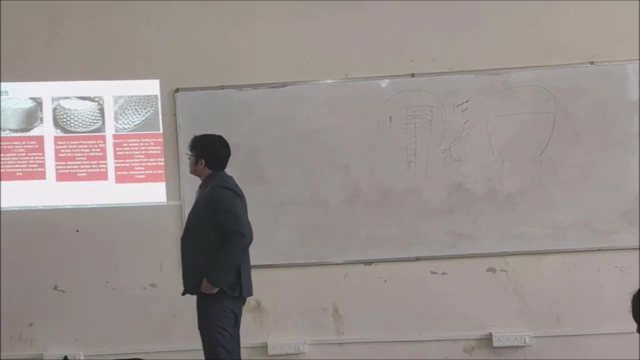 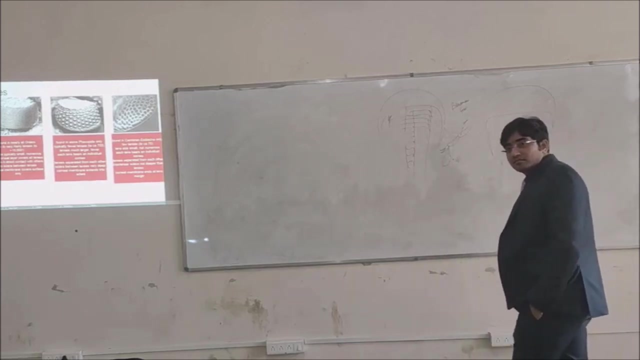 they could see. So it was an intelligent group of invertebrates which had their vision And the eyes. they were of three types: The aqua with eyes and trilobites. You have seen trilobites in PC, right. 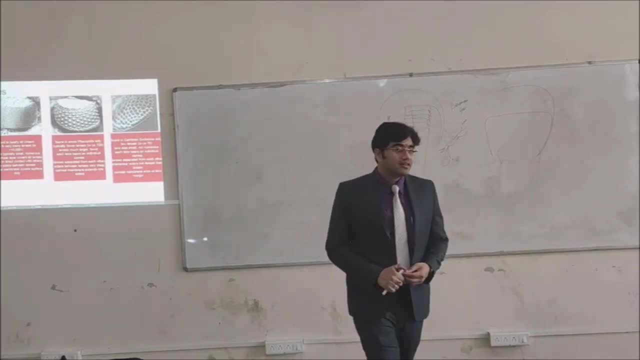 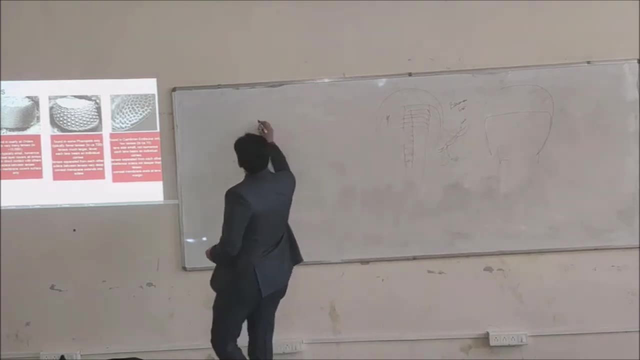 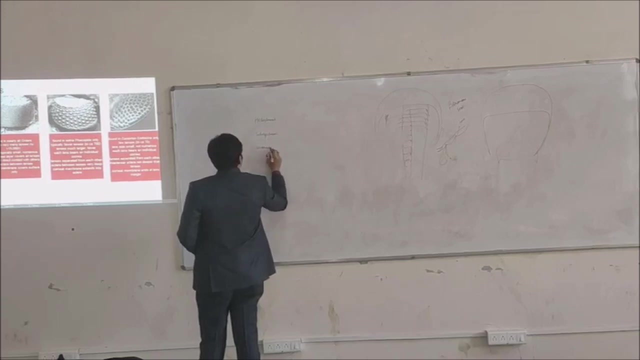 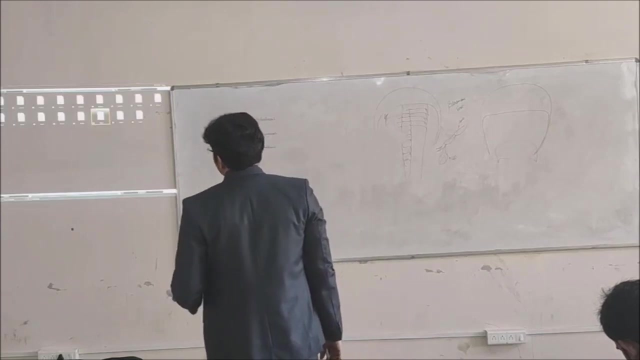 Do you know what kind of eyes they had? Any idea? It had three types of eyes: Polochrome, schizochrome and abacochrome. Polochrome, schizochrome and abacochrome. All right, Now if we look at, 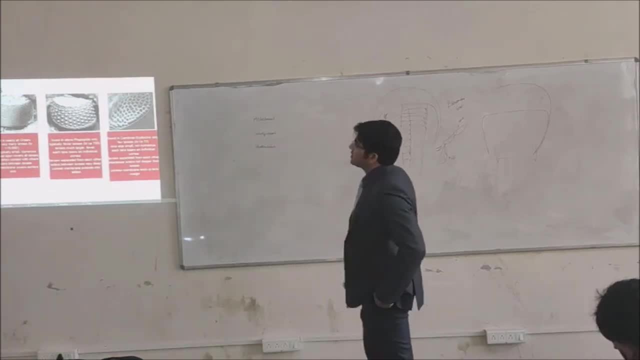 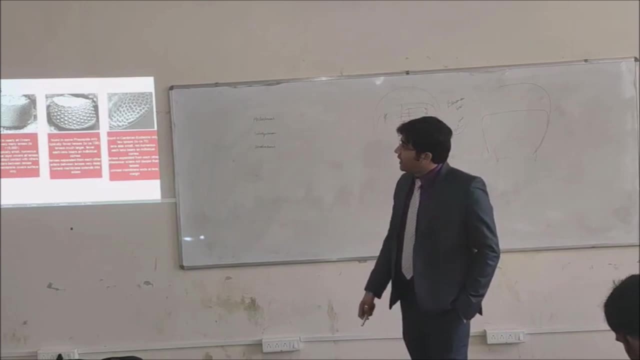 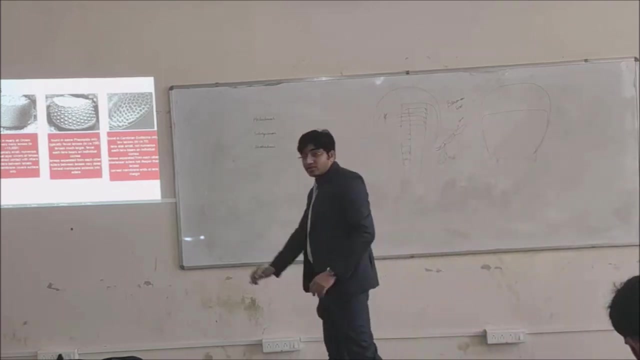 these three types. we can see here that the most common type of eyes were the holocobal eyes. It had several lenses, more than 15,000 lenses. And let me tell you one more thing: that the eyes of trilobites were raised from the surface. 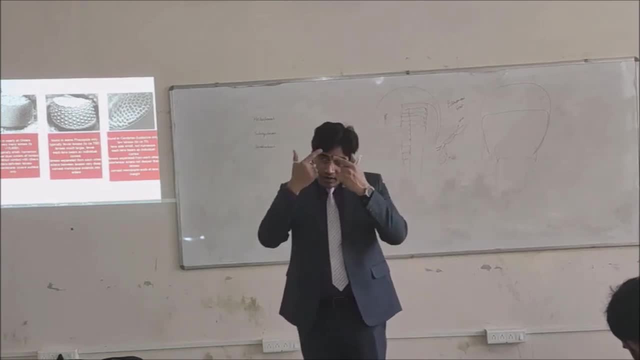 Our eyes have been pushed inwards, Our eyes are in this depression. The trilobite eyes were on the ocular platform. It was raised like this on the surface. So if you see that the trilobite is sitting on, this suppose and this is the facial suture. 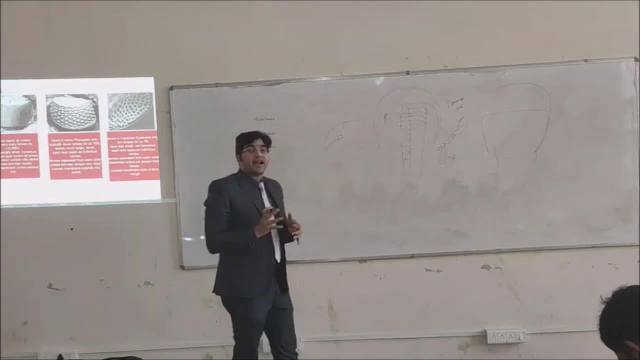 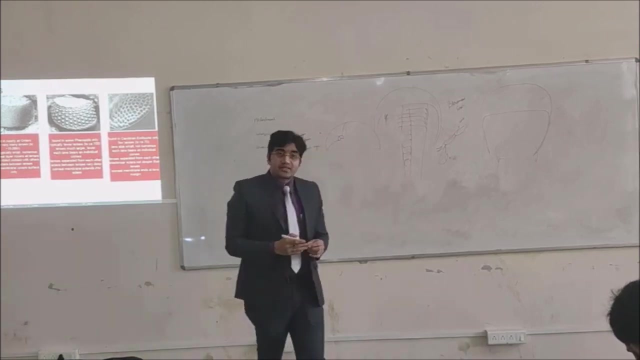 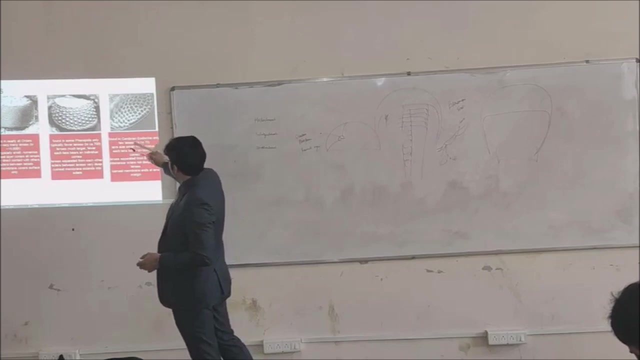 So if you see this, this is called as ocular platform, Ocular platform, which had raised eyes. They had several lenses. The main of number of lenses was there here, The holococcal eyes you can see here It had this. 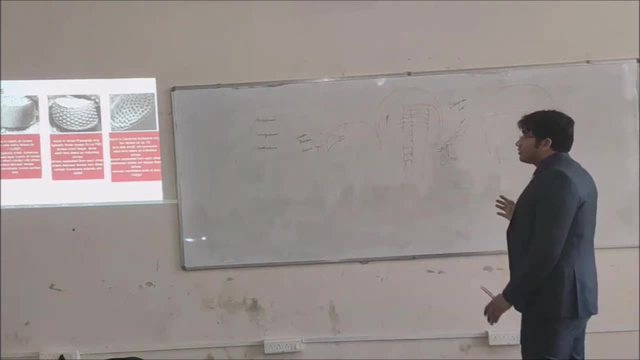 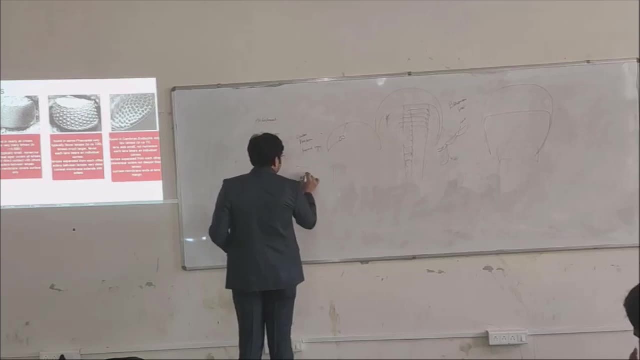 It had smaller lenses And one corneal layer. One layer used to cover all the lenses, So there was one layer which used to cover this all Corneal layer. That was the holococcal eyes- Very common eye which was found in almost all the others. 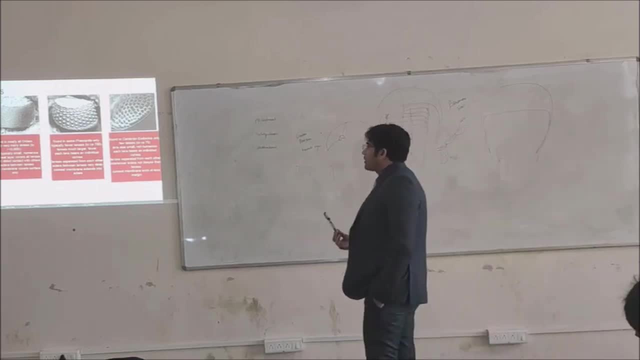 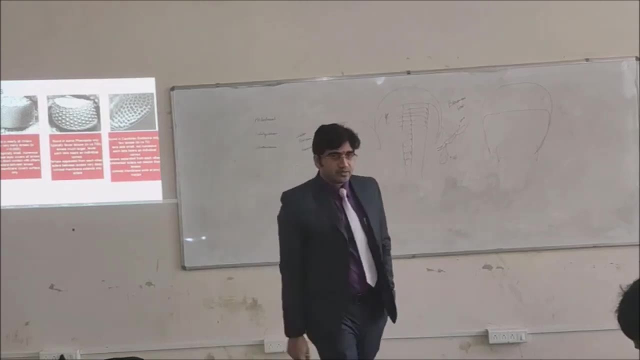 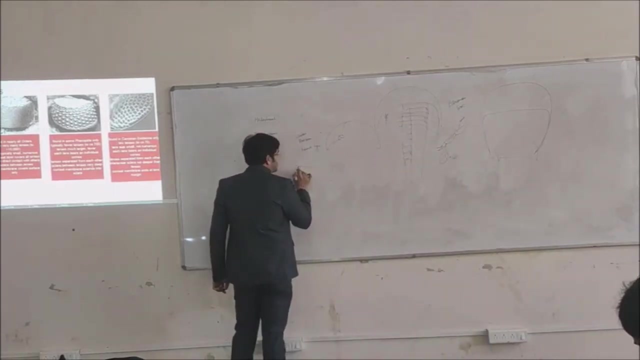 In some phagops only phagopida, not phagops, phagopida order, where the lens number had reduced and size had increased, The schizophor And each lens. Each lens had its separate corneal layer. 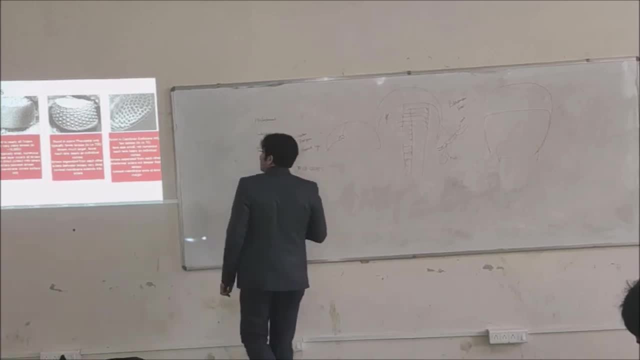 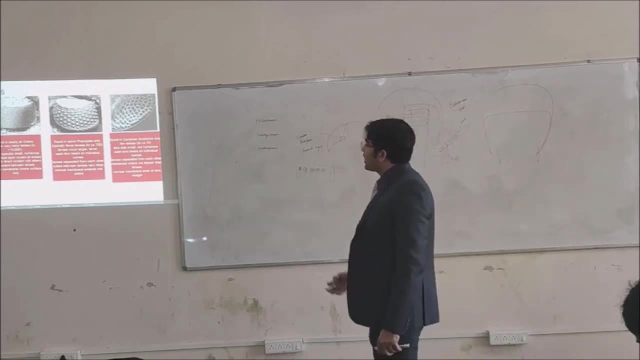 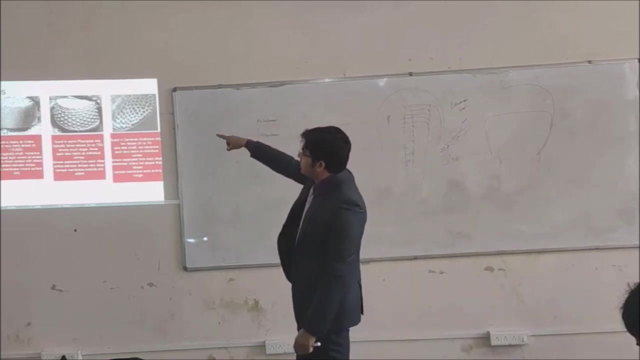 Each lens And then the eodystina. They had this, Where, then again, the number of the lenses were further reduced. The size was slightly smaller than the schizophor And each lens had its own corneal layer. Okay, 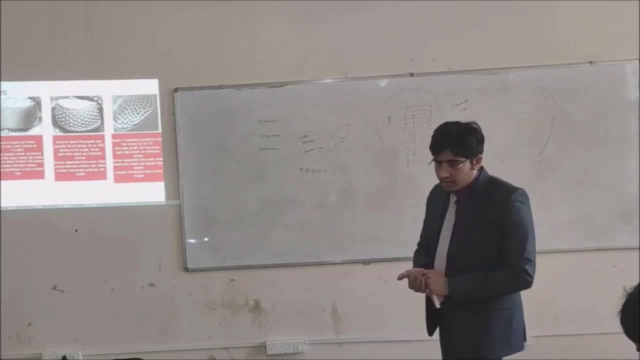 Each lens had its own corneal layer. Now These are the three types which were used in the GSI. If you go here, you will find a lot of problems. Give an example of this: That holococcal was found in almost all the others. 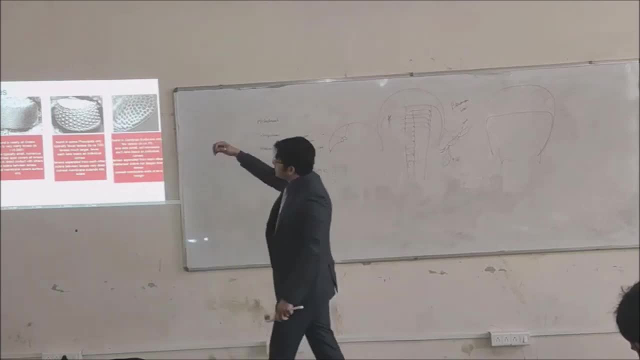 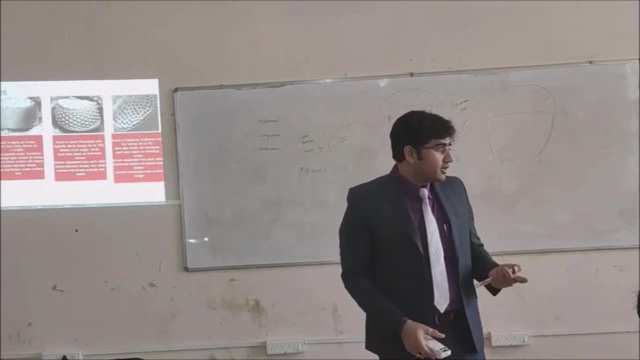 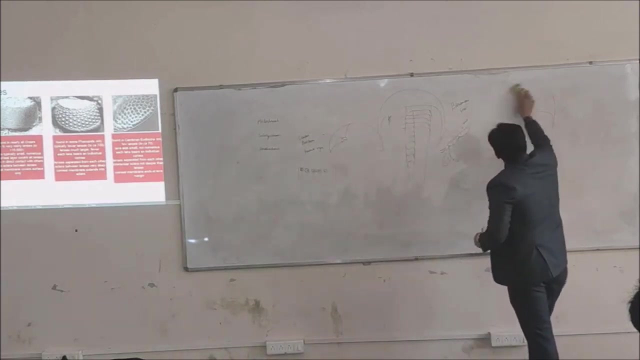 Schizophor, in some phagopida only Hathor corneal, in some eodystina only. What is important is the composition of the lenses of trilobites, The lenses of trilobites, So the trilobite lenses. they were essentially made up of cancite. 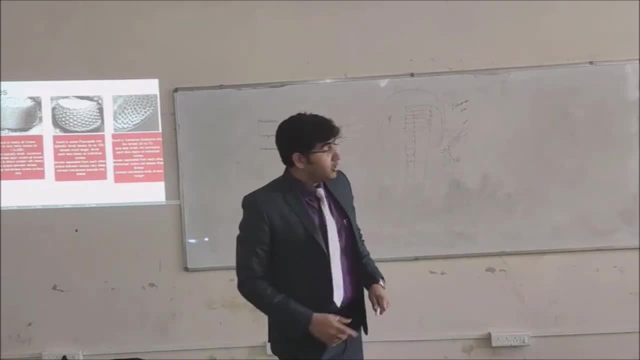 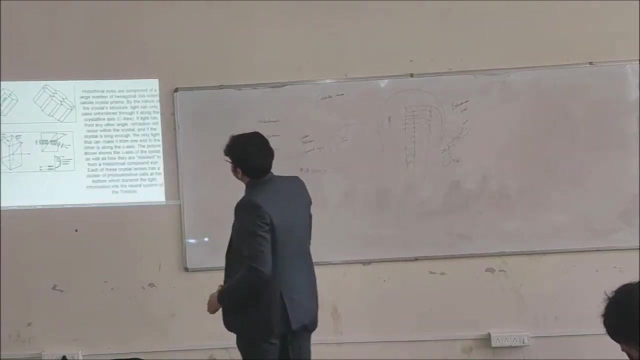 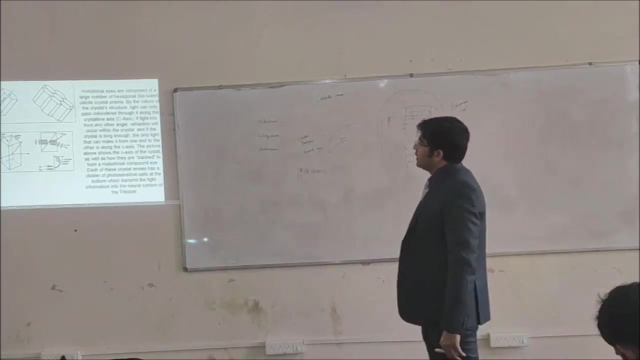 The hexagonal prisms. The lenses were cancite, Cancitic lenses And if we look at this picture, If you see here, Holococcal is composed of a large number of hexagonal calcite prisms. We all know that the optic axis in calcite is the c-axis. 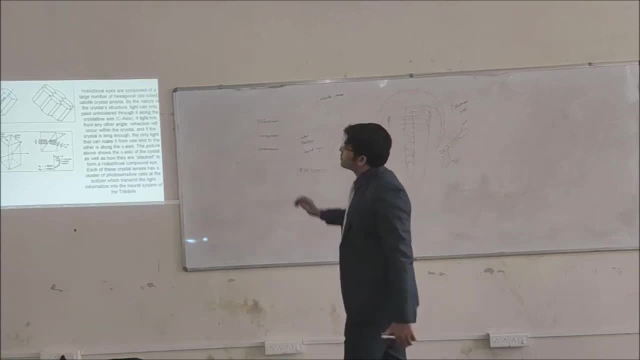 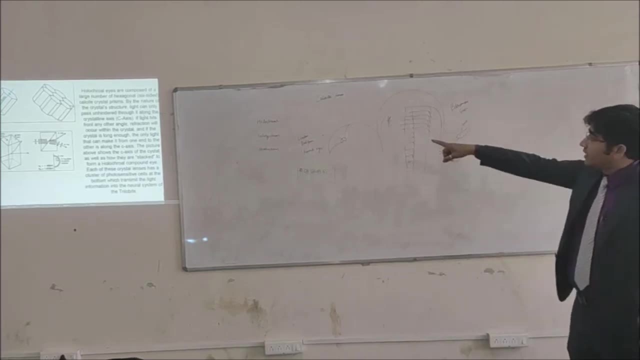 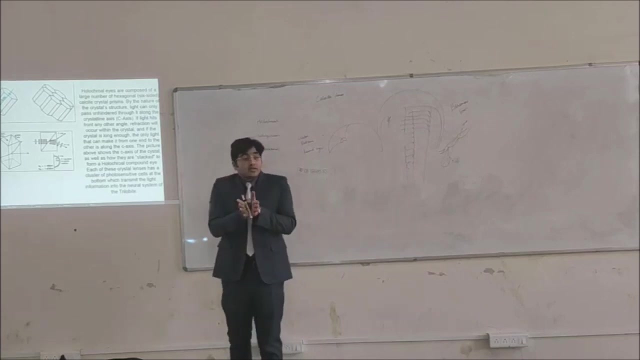 So if you look at that diagram That by the nature of the crystal structure light can only pass unhindered through it along the crystalline c-axis. If that light passes through the c-axis Then it would give it a wide field of vision. 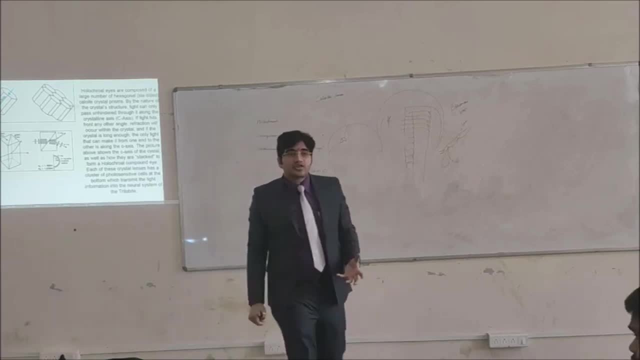 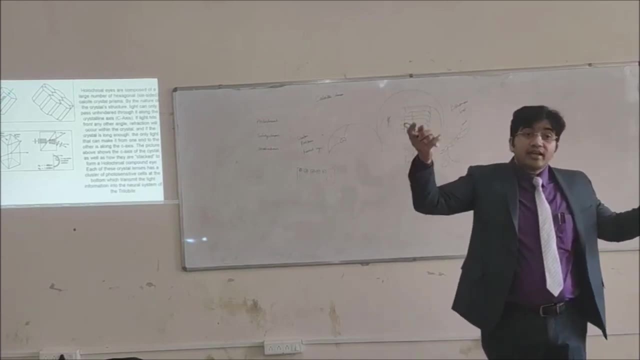 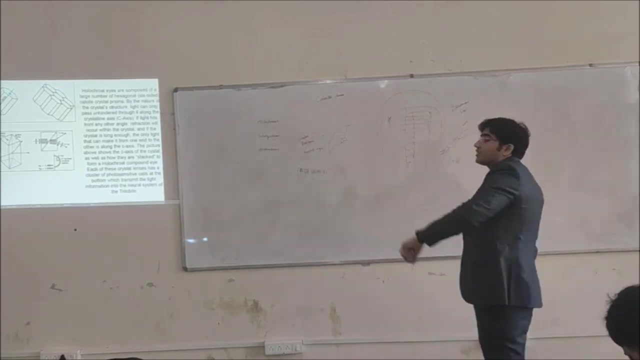 Therefore, even in the dimly lit conditions, Where the lights are very dim, Dim light conditions, When this wide field of vision was there, It was due to the calcite lens, Even if one ray of light is passing along, that Hitting along the c-axis. 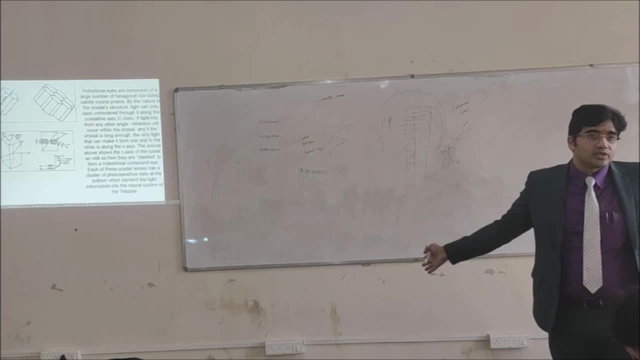 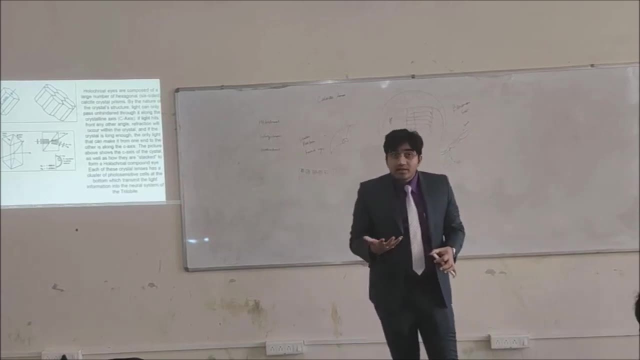 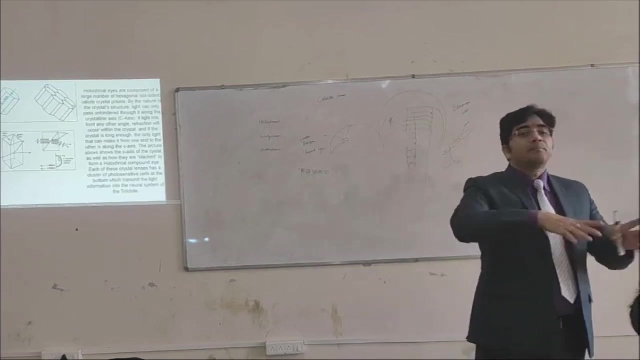 It would give a wide range of vision And since these lenses were many, There was not even one lens. Light would pass through either of the lenses If one of the lenses, The ray of light hits the c-axis, And it would give a wide field of vision. 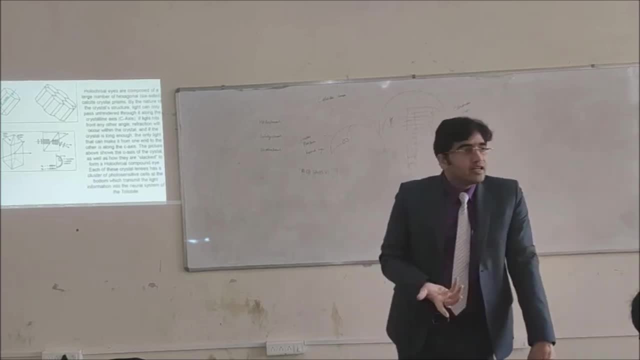 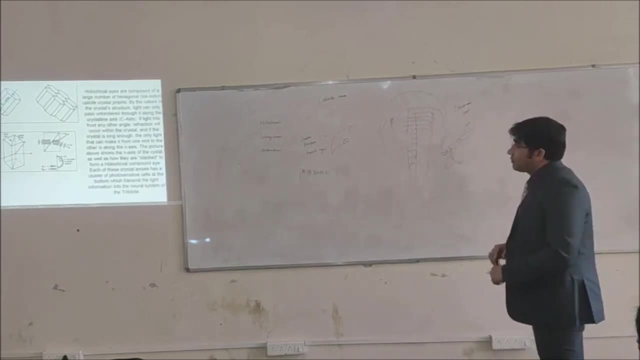 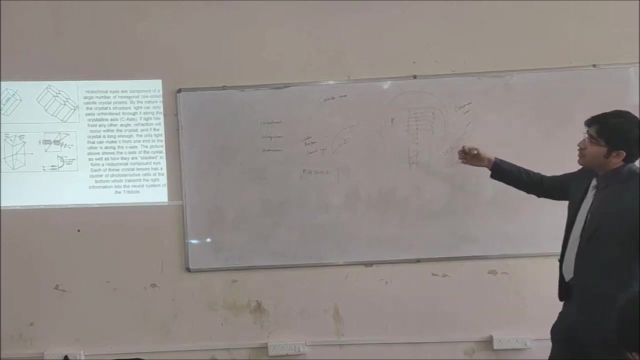 It was enough for this type of light, Because they were, And even if they were in dimly lit conditions, In water, the light will be less, Isn't it? So the calcitic lenses Which were stacked: See the first picture. 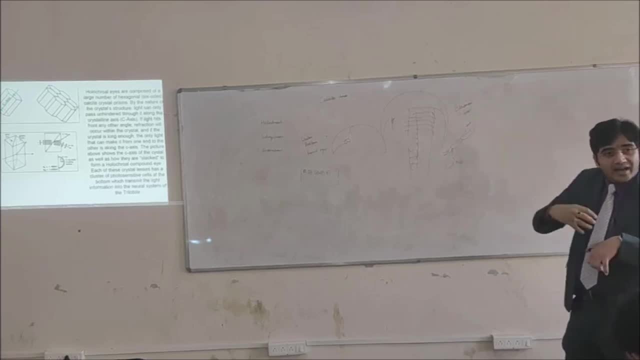 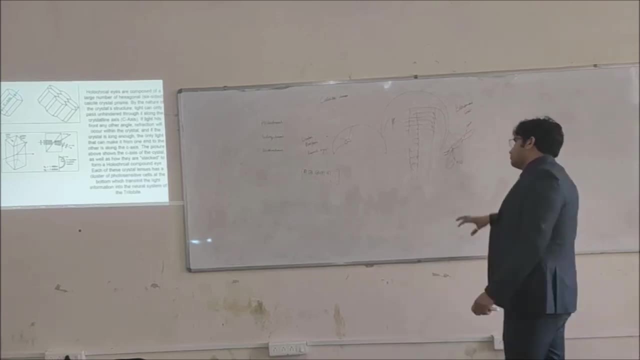 This was how the hexagonal prisms were stacked In the dilogite axis. Is it okay? This is very important You should know. Okay, Dilogite has three types of bodies, But they have lenses of calcite. The optic axis is c-axis. 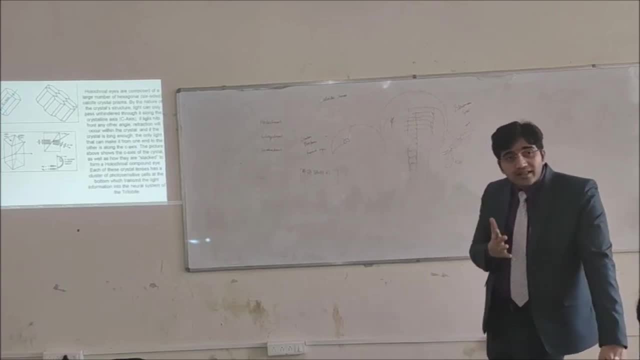 Through which the light would pass unhindered. But if it hit that It would give a wide field of vision. You all have read about the nickel prism. Which mineral is made of the nickel prism From the inside? If we cut it from the inside? 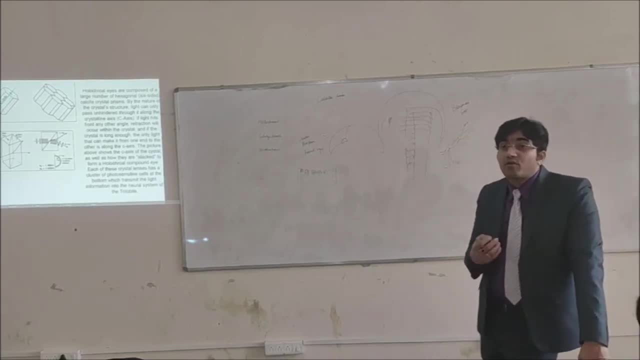 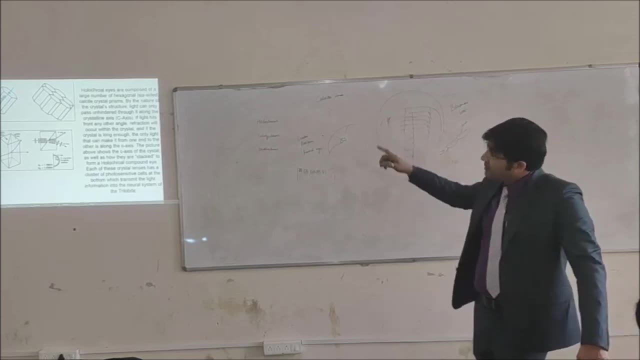 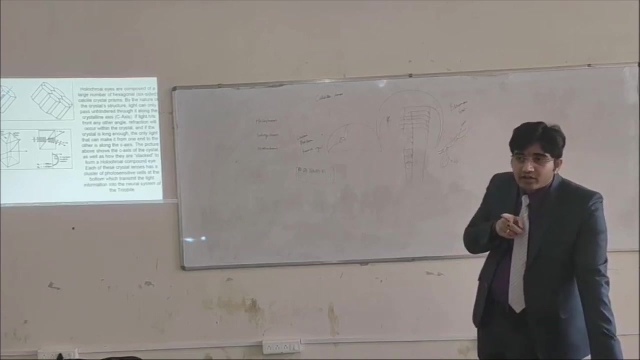 If we join it, So its RI would change. That is how You do the Petrographic microscope Right Same thing over here That the optic axis Was the one If a ray of light Used to pass through it. 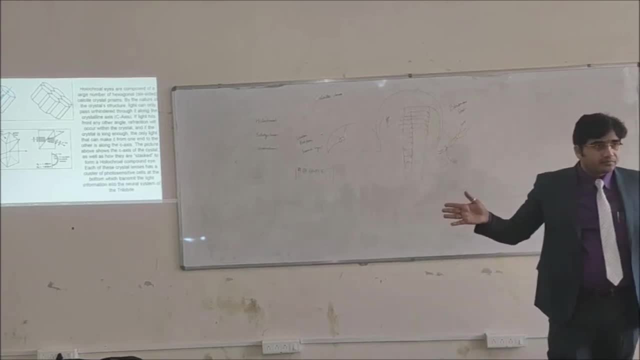 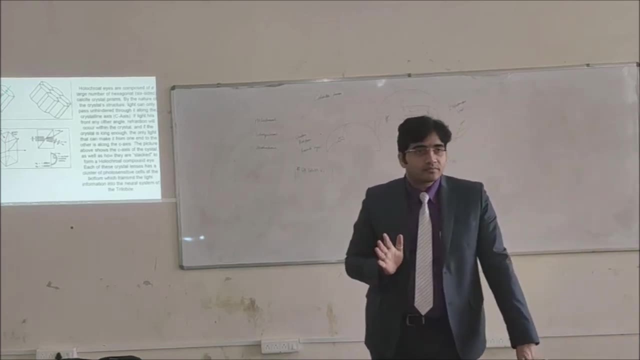 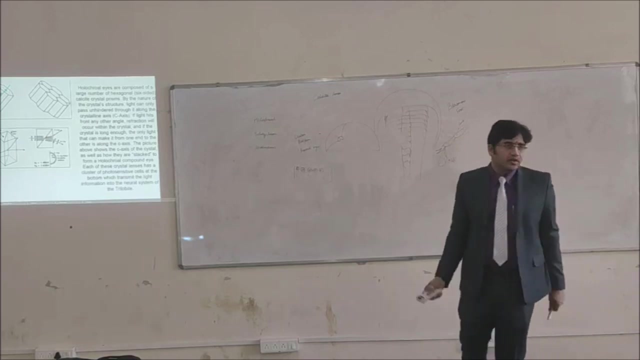 Then it would increase the vision field And, since there were several calcite lenses, It would give a improved vision. Okay, Is it okay? Okay, I will give you this, These pictures. Don't worry, If you wish to draw. 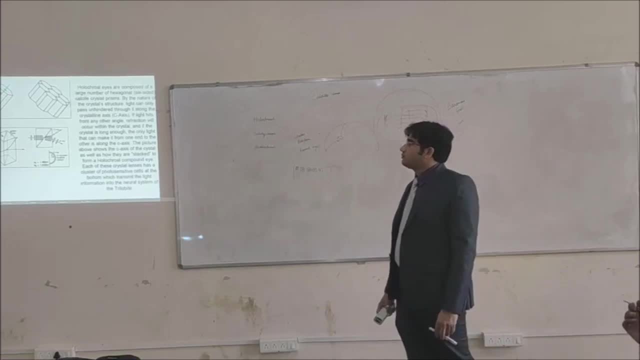 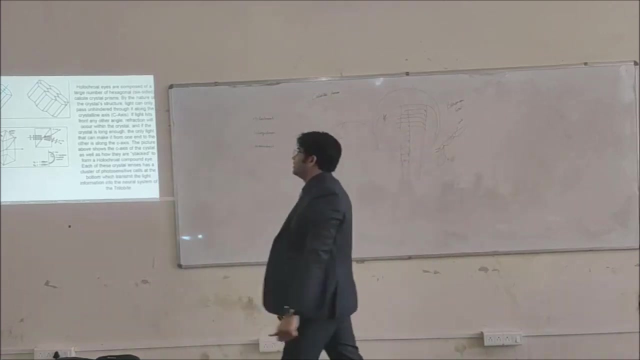 You can draw it. I will give you a picture, But after this You need to draw To see. To see. Okay, By the way, This is called. This is called. By the way This is called, Sir. 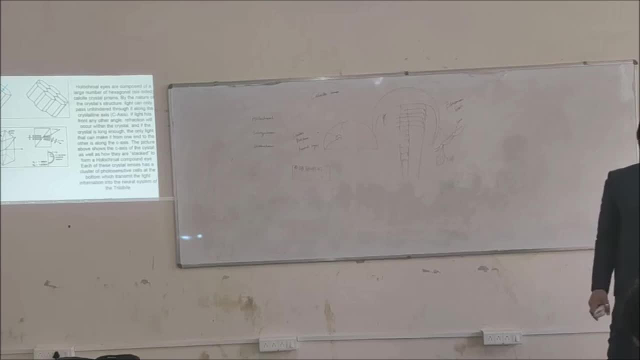 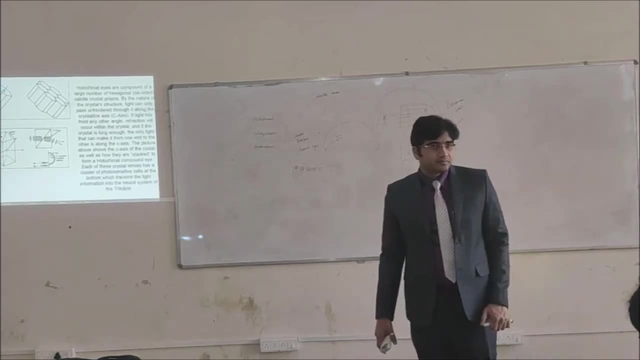 These eyes are quarter, Yes, Kind of quarter. Yeah, They are rays from the surface Because they are on the oculon platforms. They are not in depression Following it. This is a picture of the mirror. Okay, Yes. 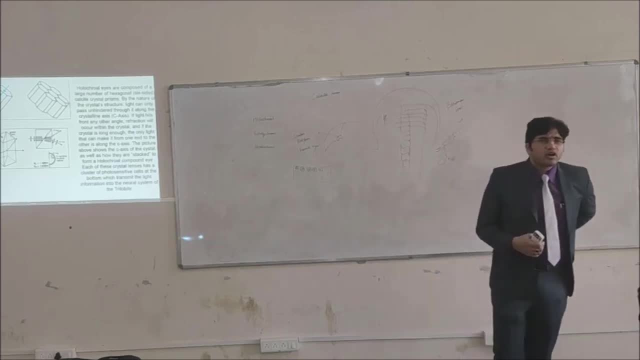 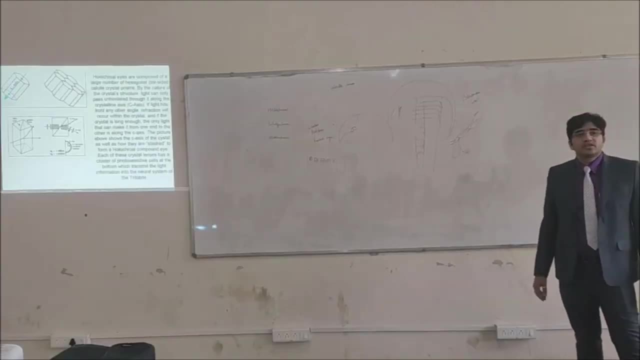 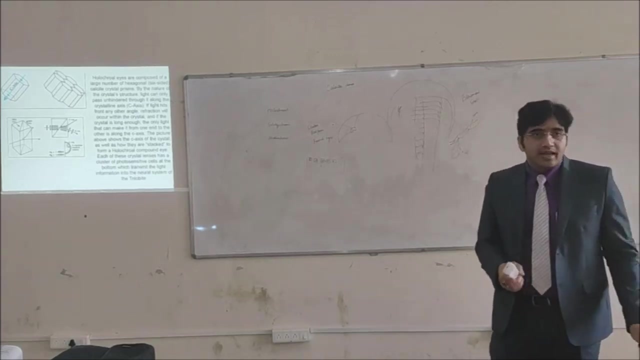 These are the interesting things about it. Draw the diagram of eye. write the name of the eye. The whole idea of functional morphology is to divide, derive or reduce the life habits of the possible group by looking at them. That makes phallicology interesting. I could have asked you to learn 10 names of phallovirus, but that is not going to help. 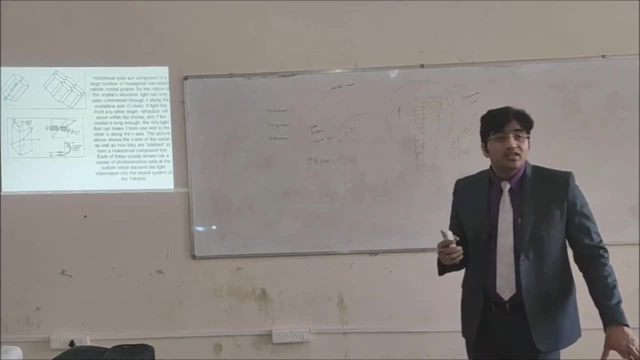 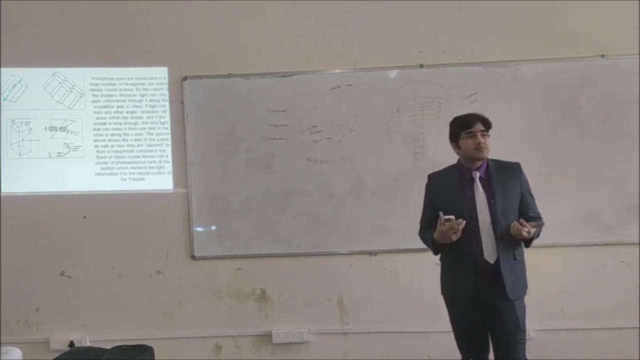 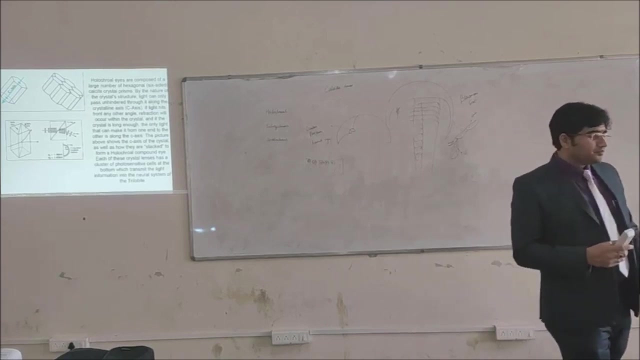 So we will be focusing more on the functional morphology. If the number of phallosis segments increases, then the shape of the body will be random: wide, bulbous, etc. These are the things which you should think. Any confusion till now. 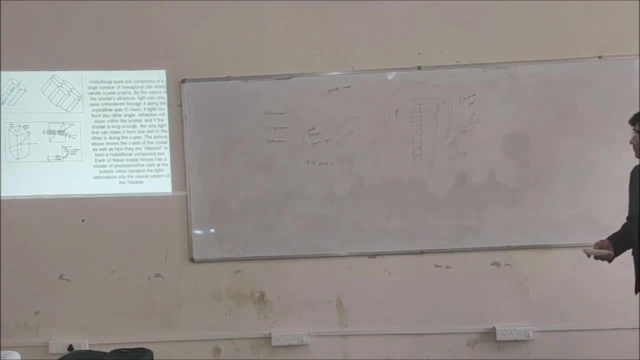 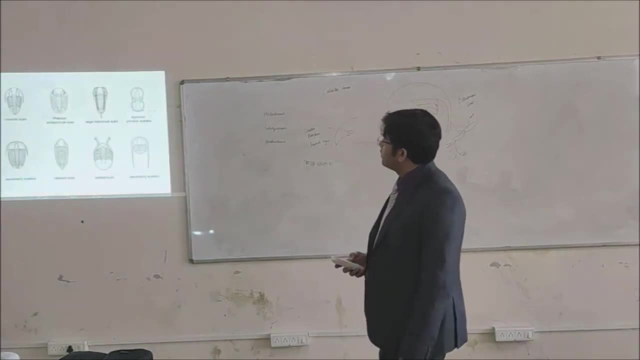 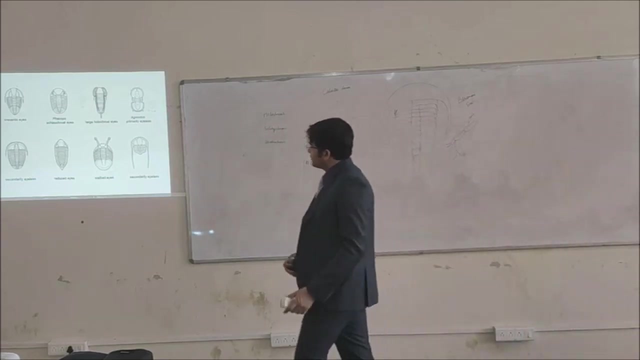 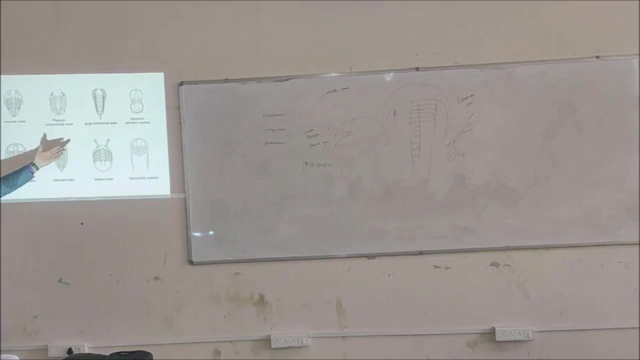 Everyone understood. Give it here. These are the different shapes of the phalloid eyes, where you can see here Chrysanthic eyes, then you know schizoproval eyes, large voloproval eyes. You can see here how the eyes are changing. They are kind of compound eyes. 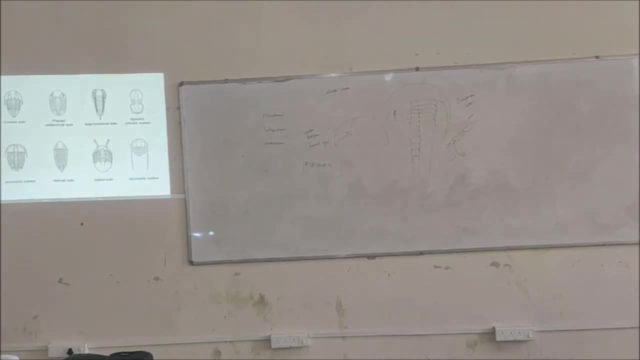 How slight they are. Have you seen? the eye of the house flies. It has got a compound eye, So these also have Now primary eyes. You can see no traces of eyes. Diagnostics: Secondary eye has phallophobe. 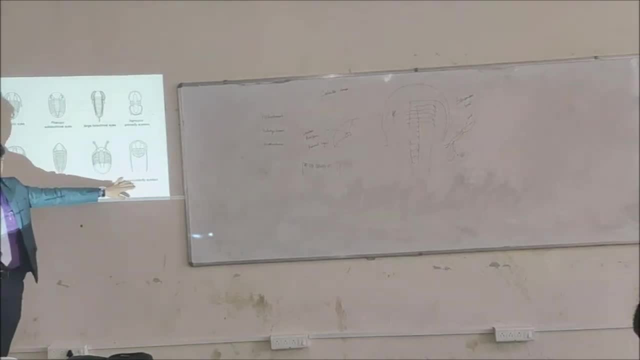 Secondary eye has phallophobe. Secondary eye has phallophobe, Stacked eyes. There are phallophobes which have eyes of ancient age, Stacked eyes, Reduced eyes. So all these changes that have taken place in the evolution of phallophobes, they have important changes. 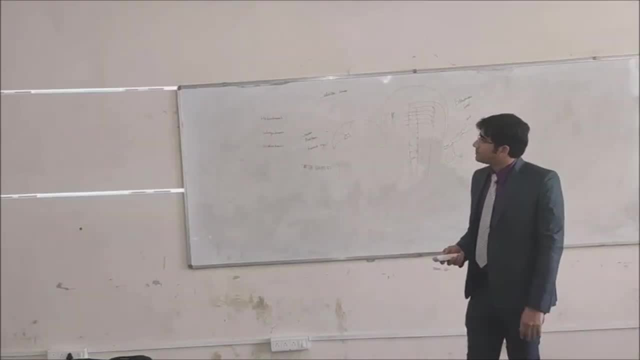 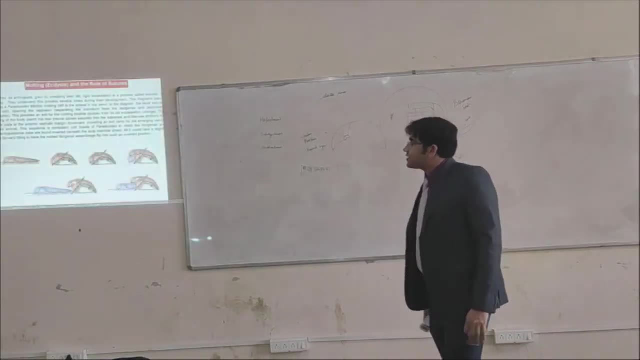 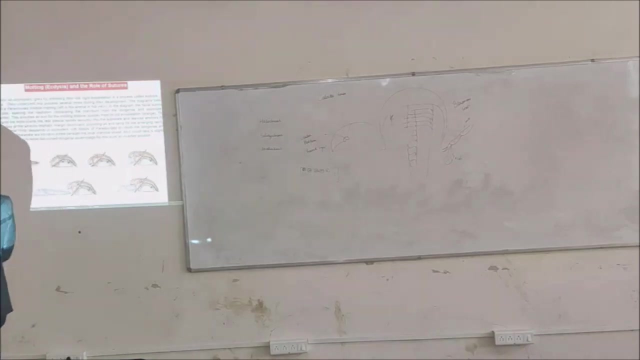 Okay, All right. Now let us come to ectasis, or mold. Look at this: Phallophobes develop several mechanisms, So, for example, enrollment. Have you seen a phallophobe which has enrolled itself, which is completely rounded? 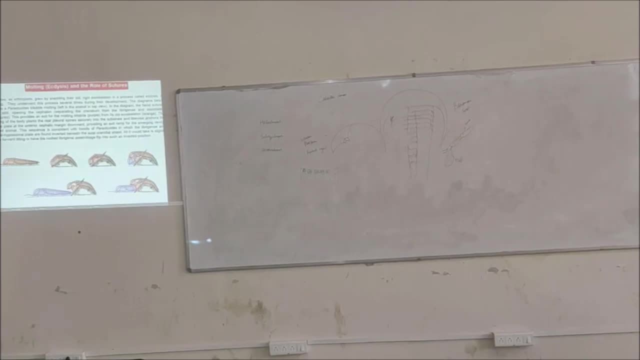 The very common diagram of phallophobes you see in books like Amol Das Gupta, you know, even in Moonlighting of Fisher of Clarkson, is enrollment of phallophobes where phallophobe has been totally enrolled. 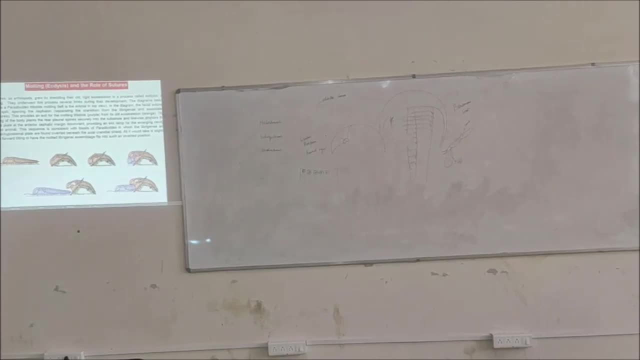 Any of those mechanisms if they could enroll their body, probably a productive mechanism. So see the facial suture. This is the facial suture. The red color How The liverigena is opening up. along that The animal is coming out and a new mold or a new carapace has been made. 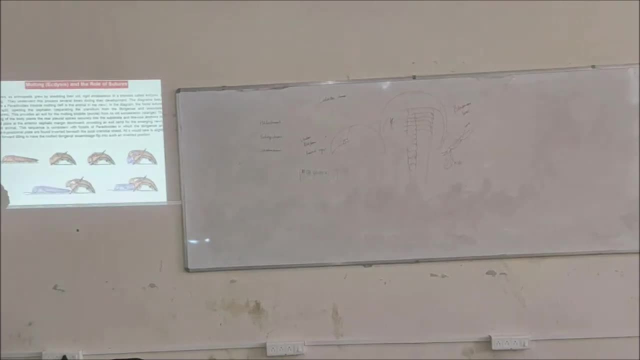 This has been described. This was an important life process for the phallophobe to continue on, But then this was also the reason for maximum deaths of phallophobes. Probably when they were opening up, they were eaten by some phallophobe. 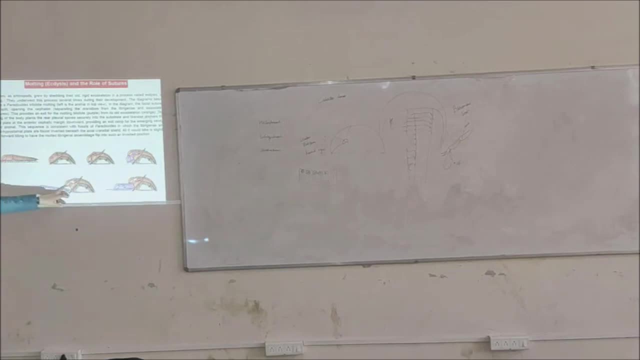 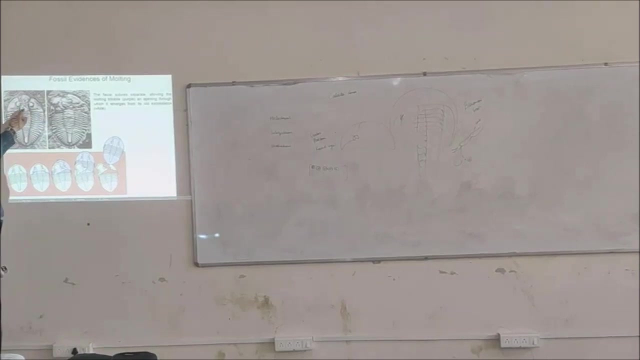 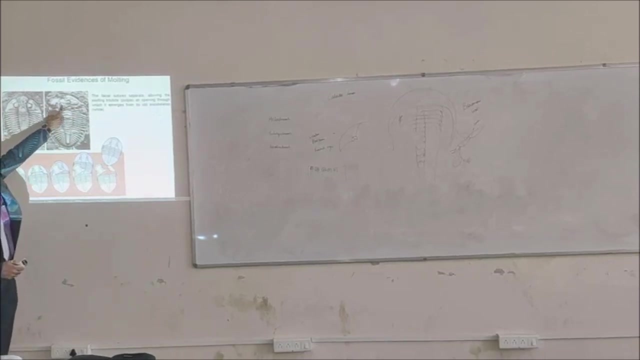 Or they could not have come out properly. I will show you a diagram. See this. Can you see that? This is the original fossil, How it has opened up? You can see the liverigena opening up and then this portion has been displaced. 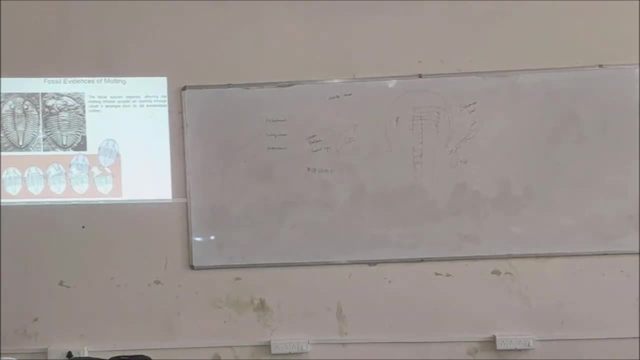 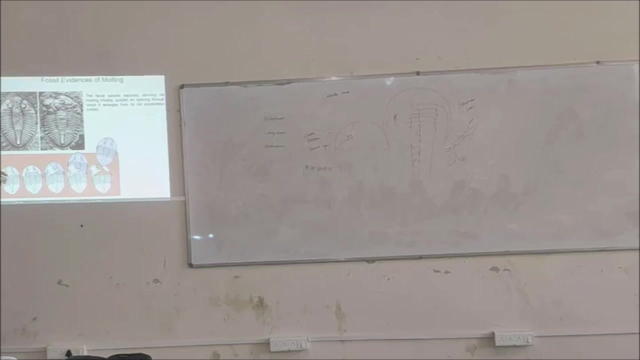 Following it. See this. This is the importance of those facial sutures. Now imagine if the facial suture was. this is an Otoscoparion suture. If the suture was still here, only this side will have been swallowed. 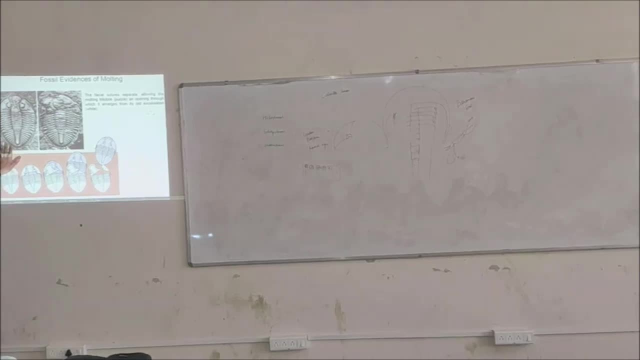 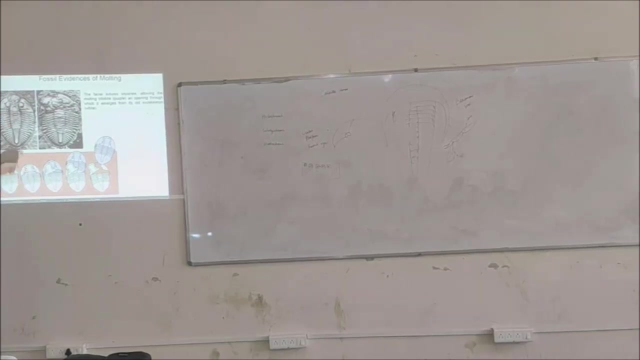 The answer to this comes from this side, Then if it was Donatocarion Vigar Prostocarion, the entire cephalon has been opened up. Okay, Did you understand this? So molding and diuresis was an important process. 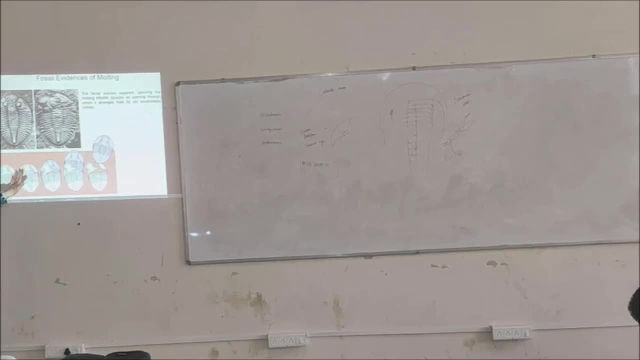 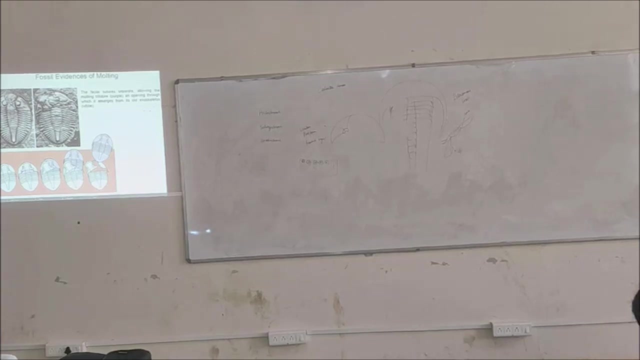 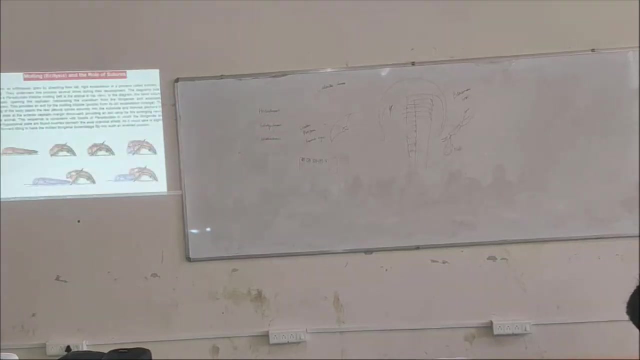 But also it was the reason for maximum deaths of these phallophobes. Probably they could get stuck in this or they were eaten up by the predators while they were going out. Okay, Any more questions? Alright, This is the molding of Paradoxide. 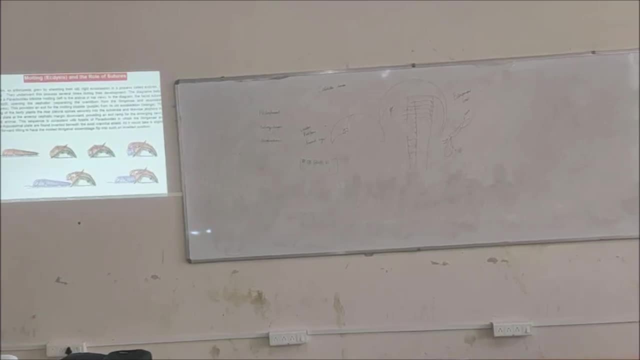 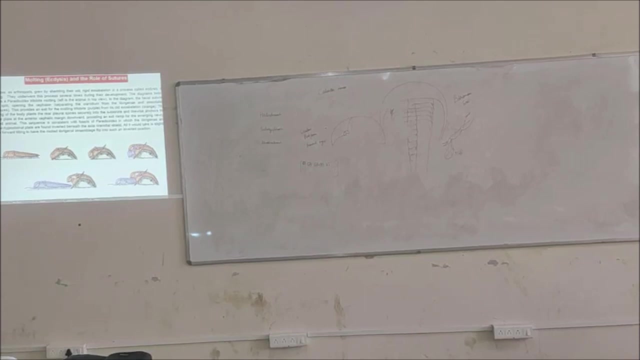 So you could go through this right up What is written in that. Okay, What questions can be answered in this? What is molding? Molding is nothing, but it is simply the change of the carapace by a phallophobe. 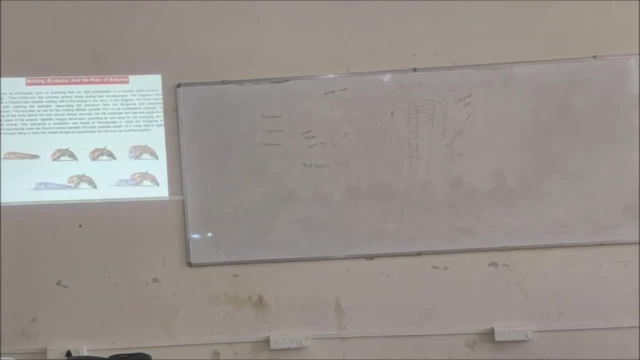 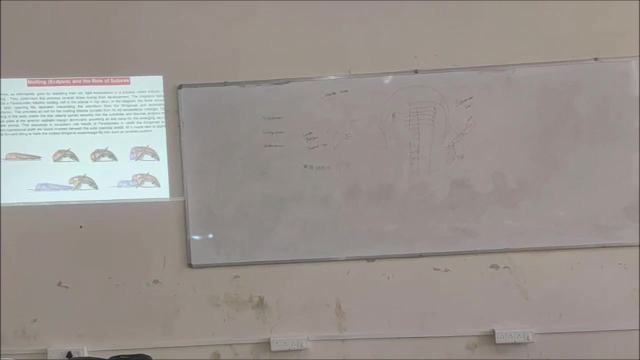 What is the most important feature that helps in molding The facial suture of the cephalon. And then what happens in there? The cephalon is opened up by displacing the libidina and the organism would come out making a niche. 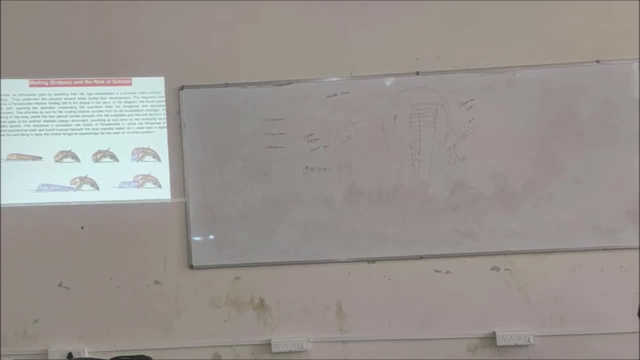 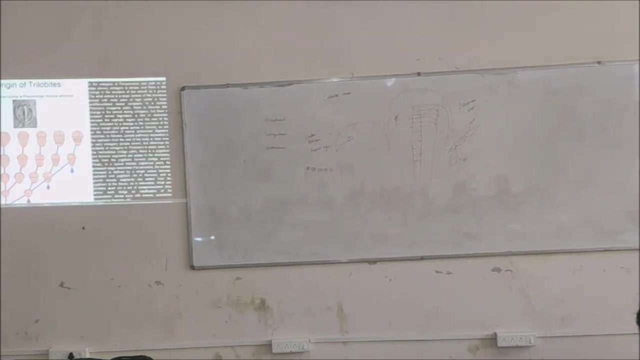 Alright, Alright. Okay, Let us now look at the origin of phallophobes. Sir, can this molding be done to give a taste to the predators? No, It changes the plastic. Why does it do that? Because it has to be tested. 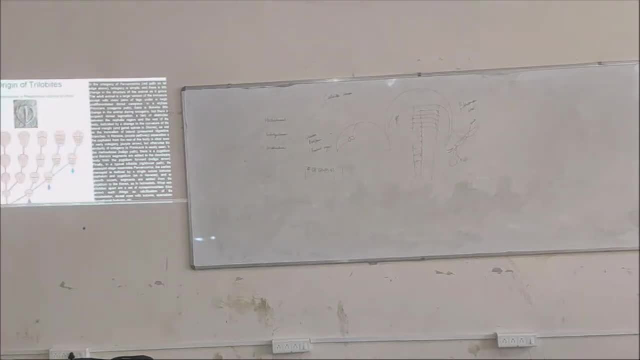 But it needs its body. For example, let us say that you are locked in a shell And you are told that this is your home And this is your part of your body. You will grow inside it. As soon as the shell grows, it will remain small. 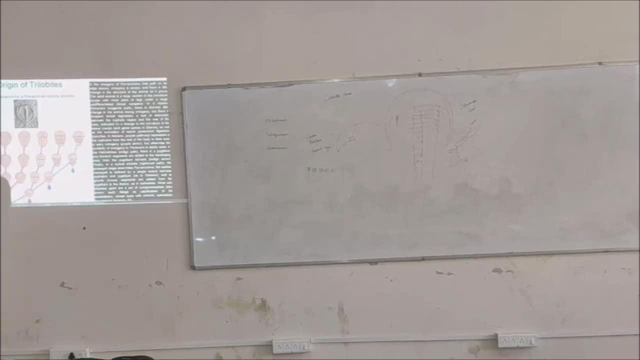 You will not be able to grow inside it. In this case, during its lifetime, when the carapace used to grow, it needs another exoskeleton. We have exoskeleton. Our bones grow with the body, But imagine that we were living in an exoskeleton. 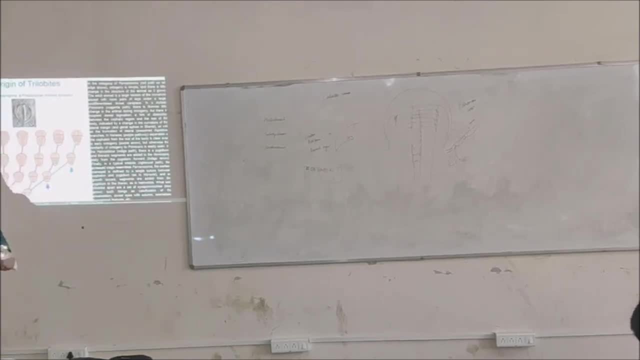 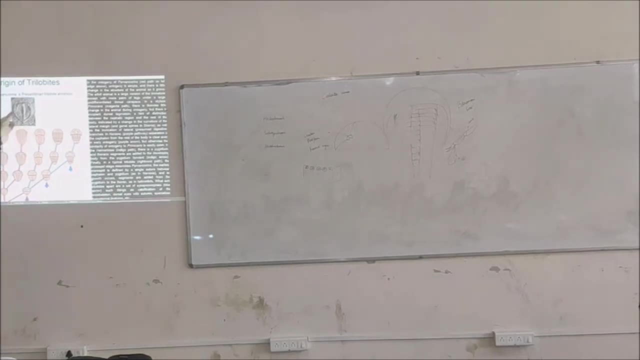 As the exoskeleton remains smaller and the body used to grow. then what will happen? Alright, This is paravankohe, which I have studied. Doesn't it look like trilobite? This is the ancestor of paravankohe. 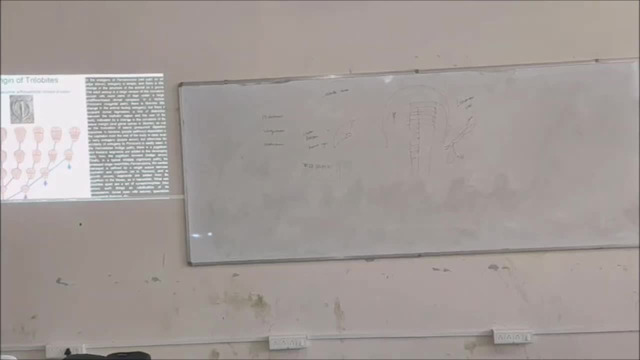 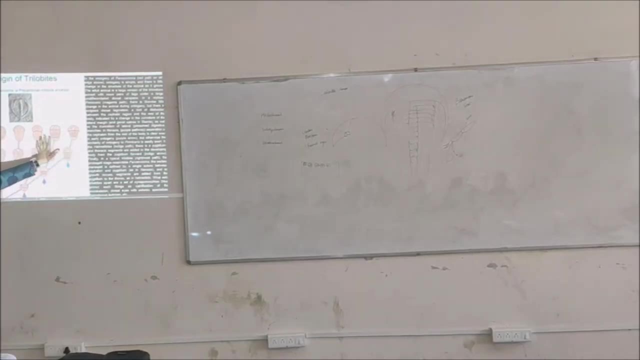 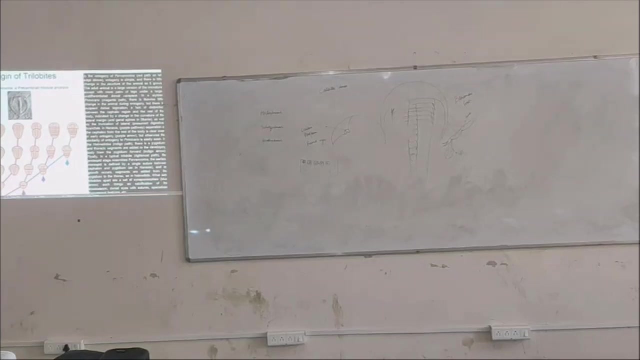 Paravankohe: Alright. From paravankohe the body starts to get segmented and then give rise to several such groups. We will come to it So. origin of thylobites: This was the pre-canon thylobite ancestor. 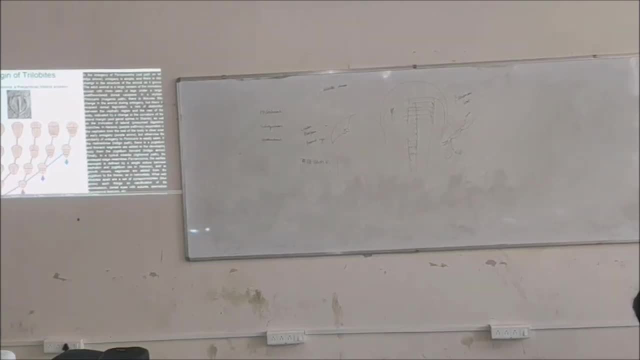 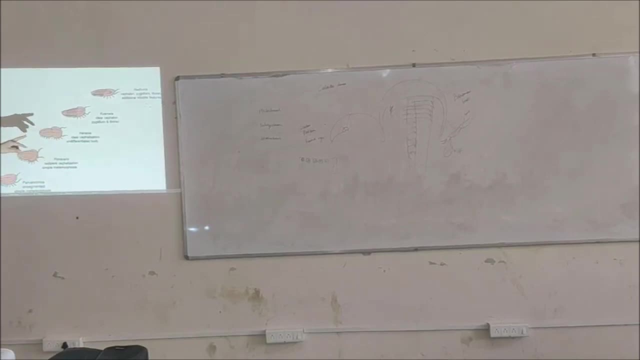 Arian thylophauna, Which gave rise to different groups. So paravankohe gave rise to primi-caris, paravansu-meroia, paravansu-tumaiya and then red lichia. 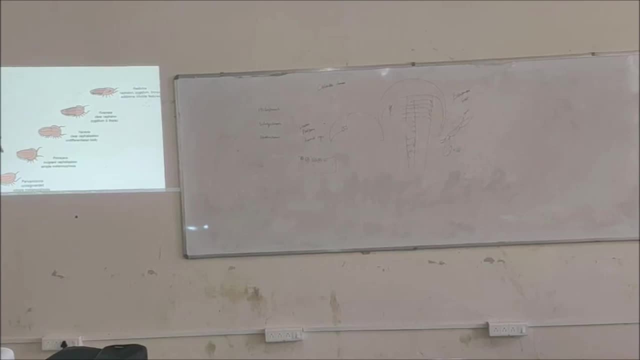 So that was the first proper phthalo. These are the different stages. You can see these stages over here. Can you see that Which is pre-explained over here? Even if you don't do this, if this name gets twisted. 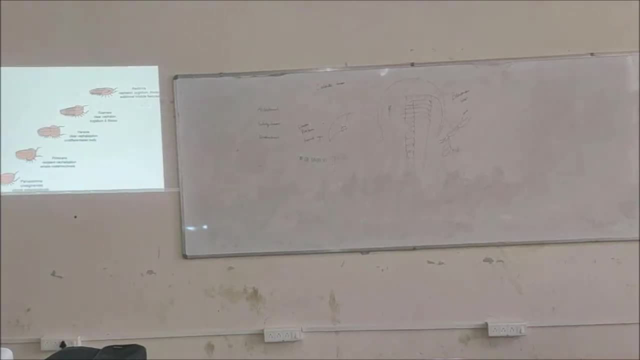 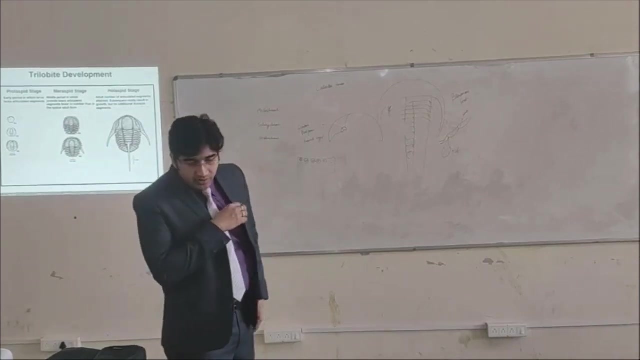 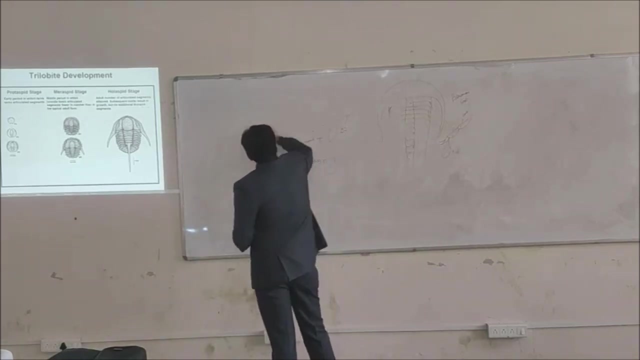 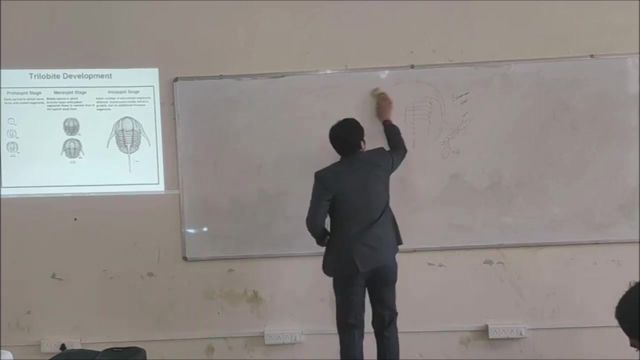 you will get red lichia from paravankohe. Okay, Follow it. Trilobite development. When we look at the growth of trilobites, the trilobites, they show three stages. The three stages in the growth of trilobites. 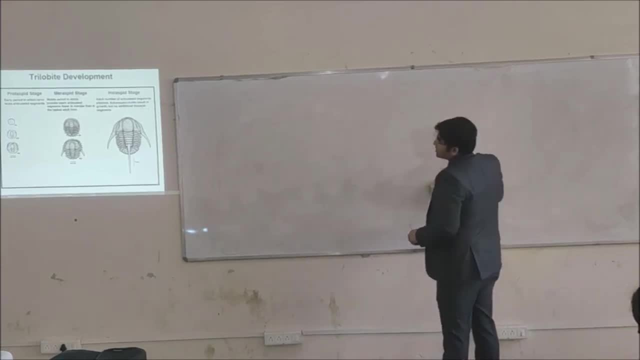 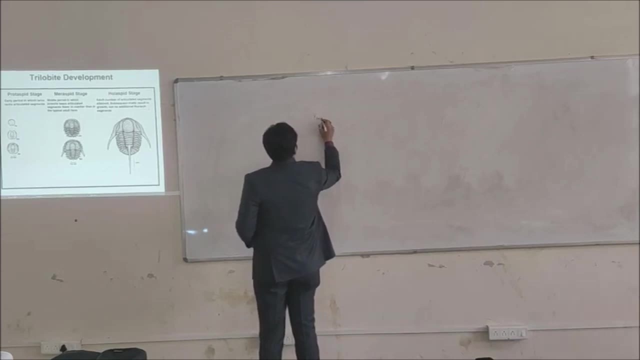 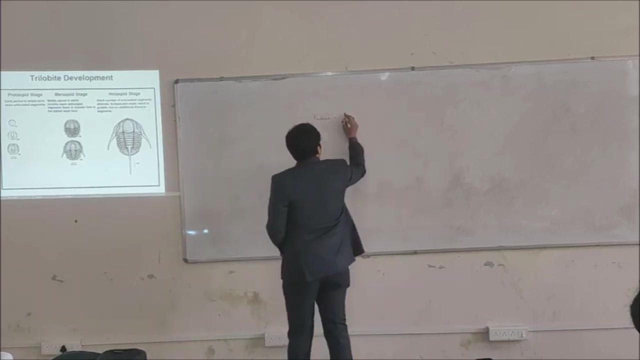 they are the protasperous stage, the verasperous stage and the collasperous stage. Protasperous- In this, what is formed is called protasperous. Okay, Protasperous, The larval stage. Then we have the verasperous stage. 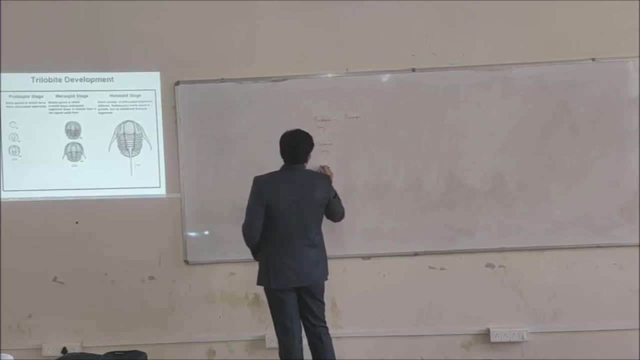 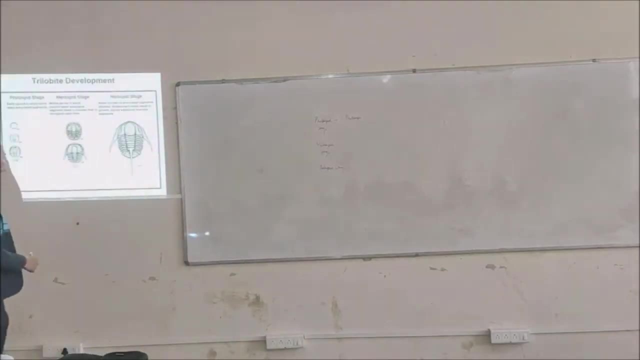 And then we have the volasperous stage. The adult stage is called as the volasperous stage. So here the larval form which shows the differentiation of the body in three groups, Followed by the juvenile form and then followed by the adult form. 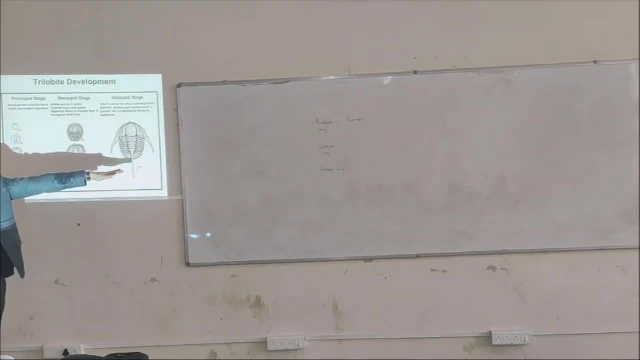 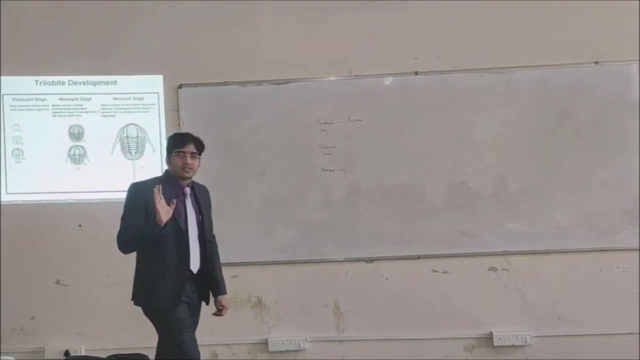 Volasperous, Verasperous Collasperous. Okay, This larval form of what is the larval First form, First form of what? In the evolution of any organism, the first stage is the larval stage. Okay, 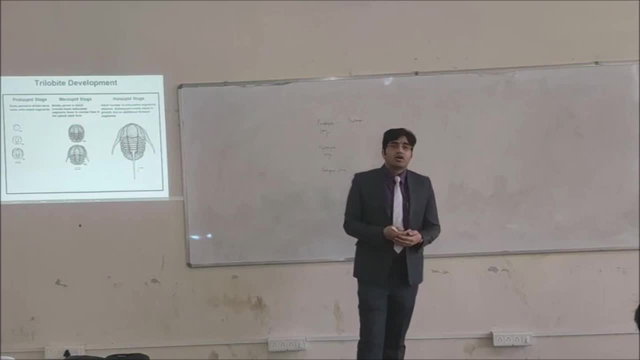 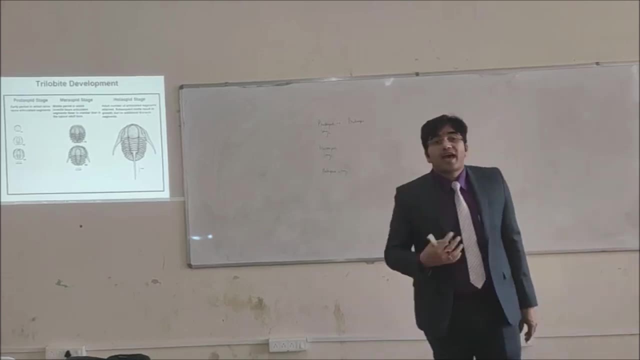 This larval could be belliger larval, or lecitotrophic larval or lactotrophic larval, You know There are. depending on the food habits or the way they are living, they have these different names. So again, 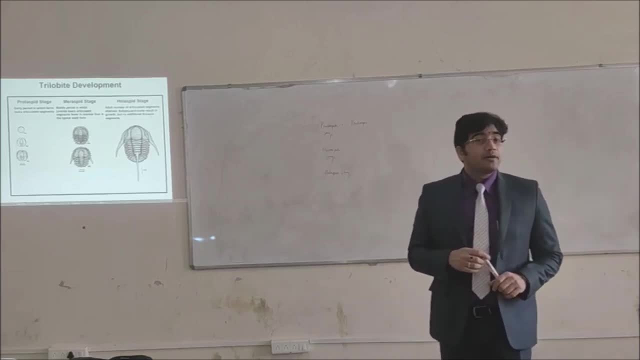 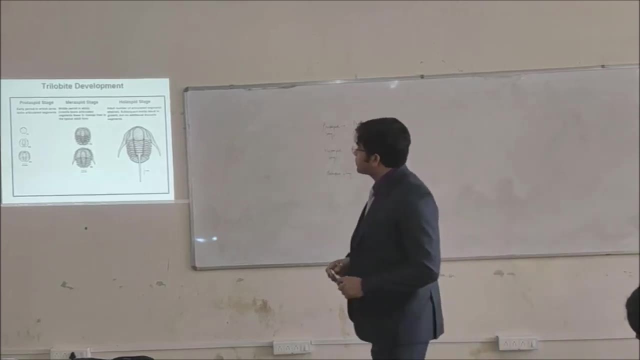 a small assignment to you: Try to find out the different types of larval stages, What are their names, And you will tell it to people, Alright. So when we look at the different stages, in case of the protestant stage, 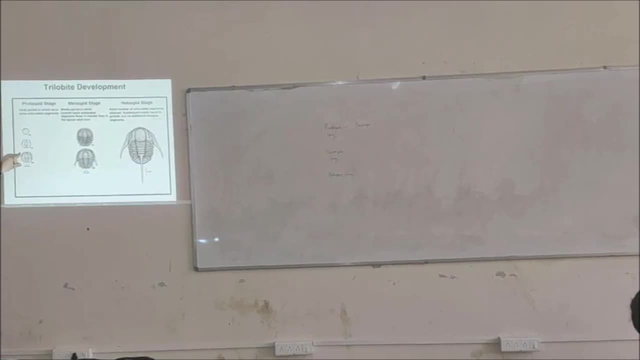 where it was the larval phase, they lacked these articulated segments. That is, the proper differentiation of segments is not there, But they are starting to show the three lobes. Can you see that? The formation of the axial lobe and the 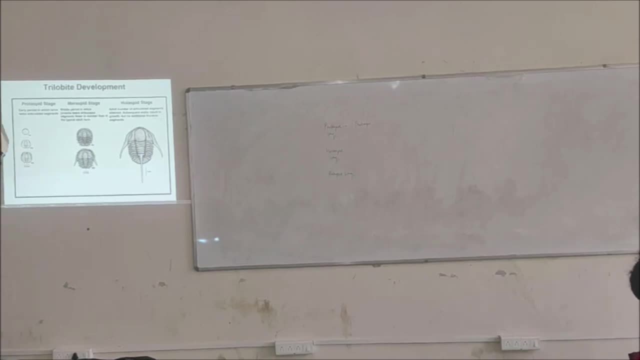 gluteal lobe. As we go to the merastic stage, the juvenile now, the differentiation in these segments, the segmentation of the body has started. The segmentation of the body has started And the segmentation of the body has started. 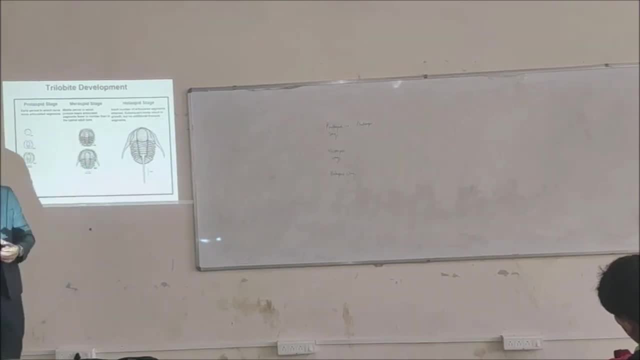 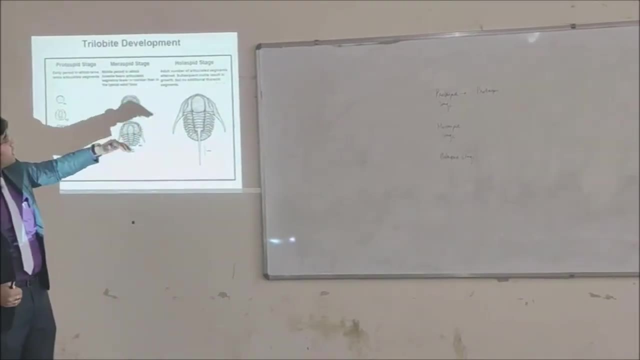 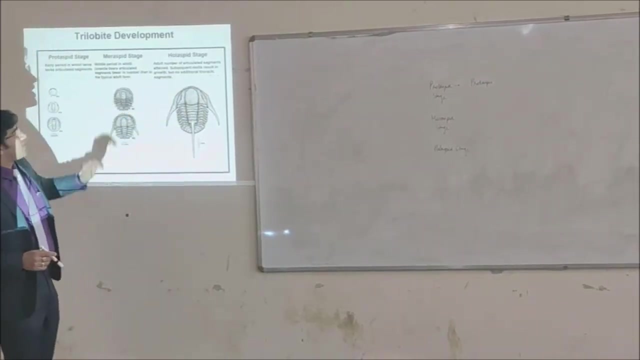 Is it okay, But still the number of segments will be fewer or lesser than the adult. That is called as the juvenile phase. It goes to the adult phase, well down to the 40. And then here subsequent modes result in the growth. 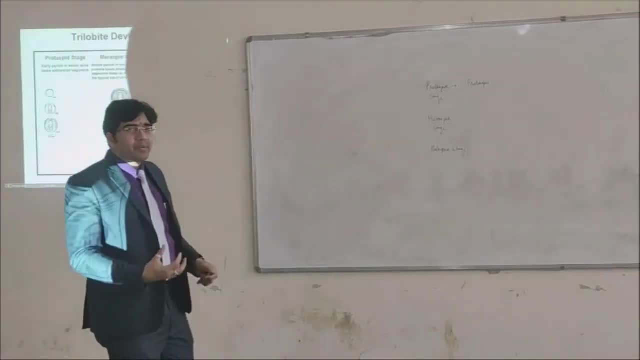 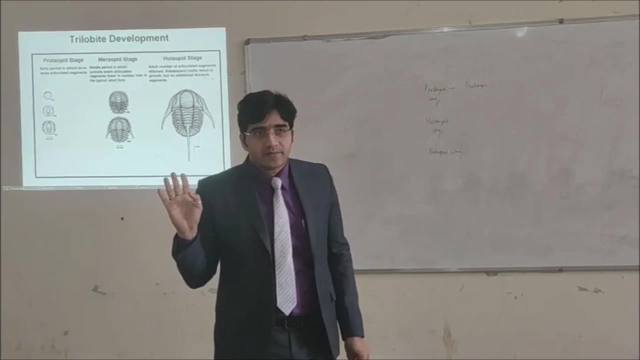 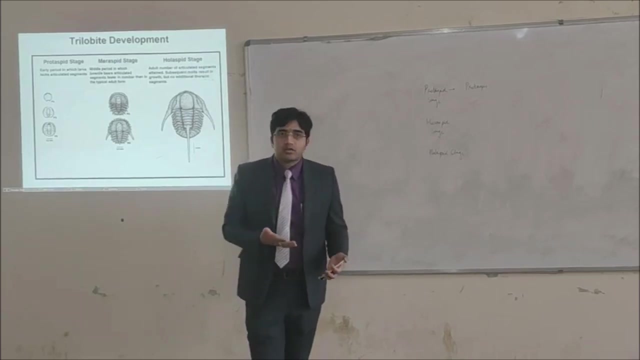 But no additional plastic segments. So once the number of the plastic segments has been decided, no matter how many segments are there, the number of segments won't change. So if, let us say, you have seen the agnostic segment, 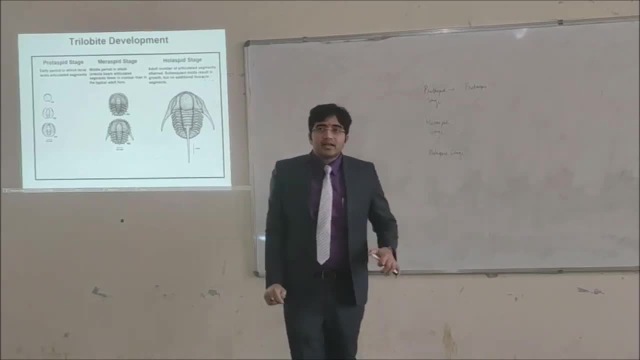 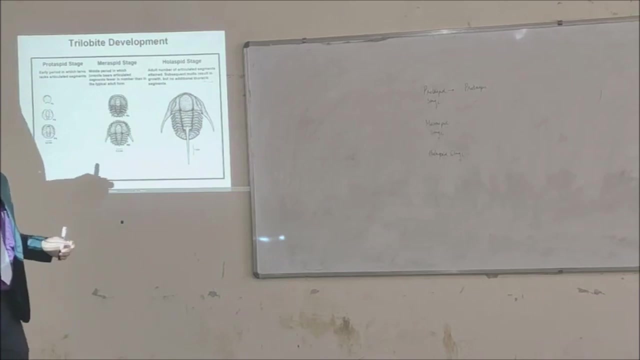 won't the agnostic do the moulding Definitely, but those segments remain true. Are you following me That if the number of segments have been decided in the to show its growth in size, but then the number of segments will change? 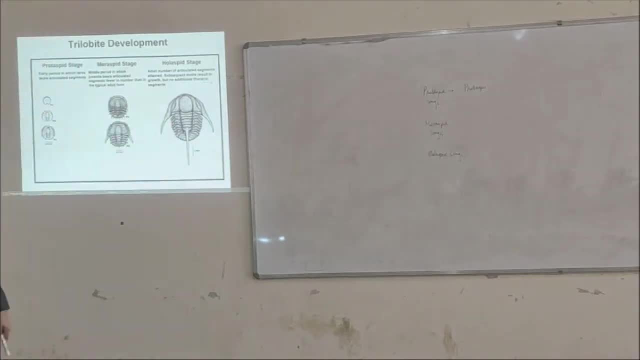 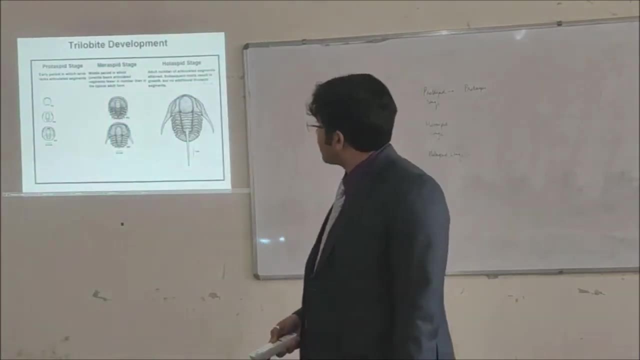 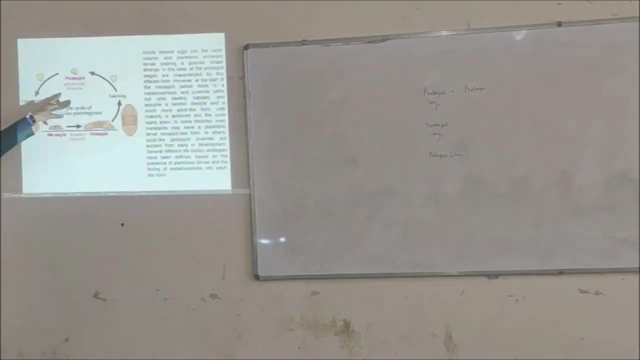 Sir moulding is absolutely Yes, Here. moulding is here. Okay, Is it okay? See this Protaspis sp, which is a plant tawny. that is covered. The larva is included in the plotter Now. 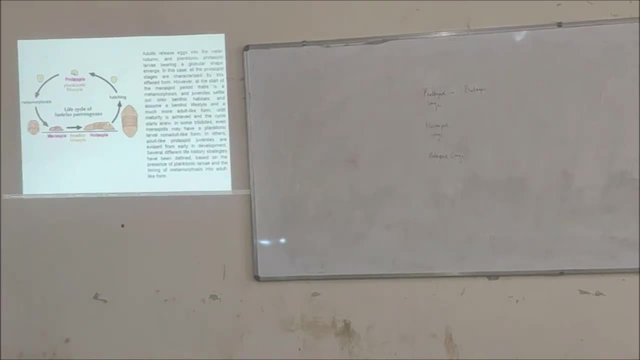 what is the plotter? Metamorphosis means it is changing its form. Metamorphosis comes up, say metamorphic roxyneon. Any change in the shape is called metamorphosis. Now, with metamorphosis, the protaspis. 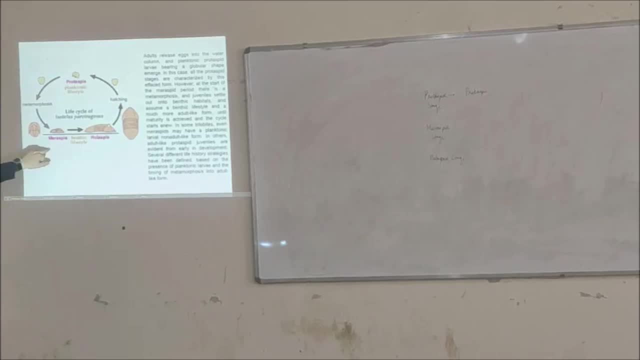 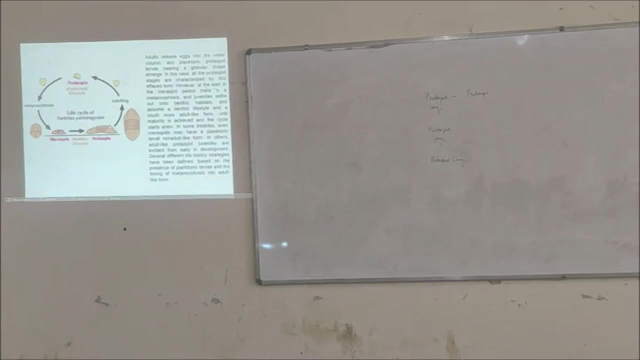 comes to the meraspis state or meraspid state, Then it goes to. So you can see here the large one stage is the plantic stage, plantony stage, the plotter, But once it becomes body, larger, 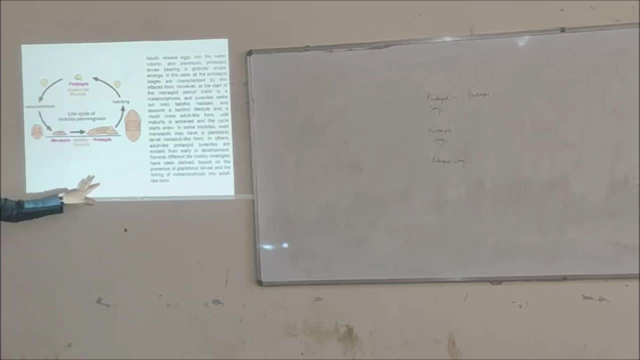 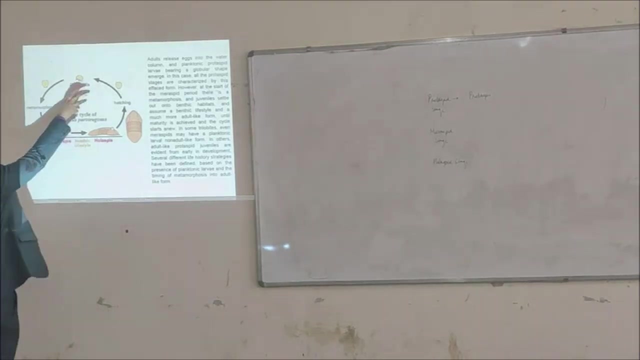 body, the and the head stages they are. They have changed from to, So these three stages they are. So when it was a, it used to eat. it was a one which, But when it became it had to. 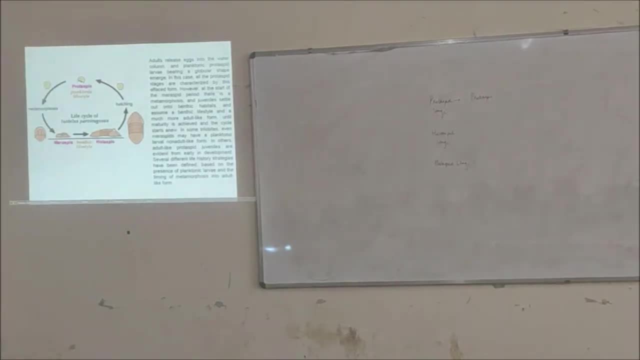 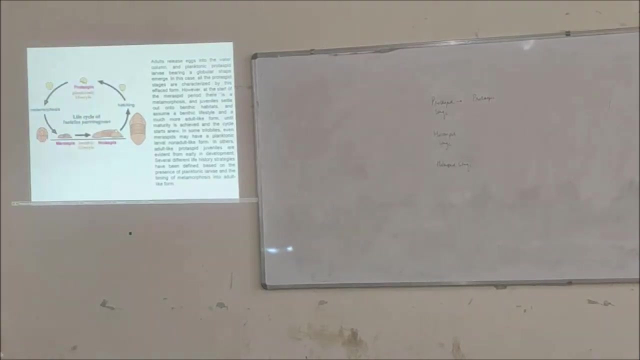 feed on the material which is there on the It's If something is floating in water. If you eat the particles floating in the water, But where it can go it will have to out the Then was the that used to. 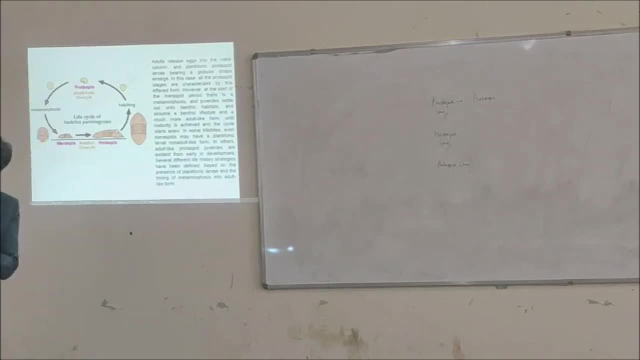 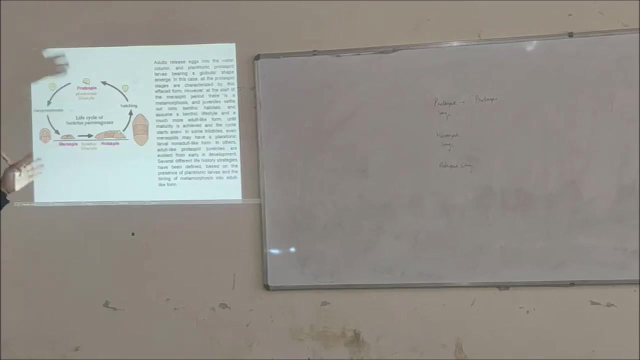 come in. Then it was: This is the part, The is all, But it is moving. 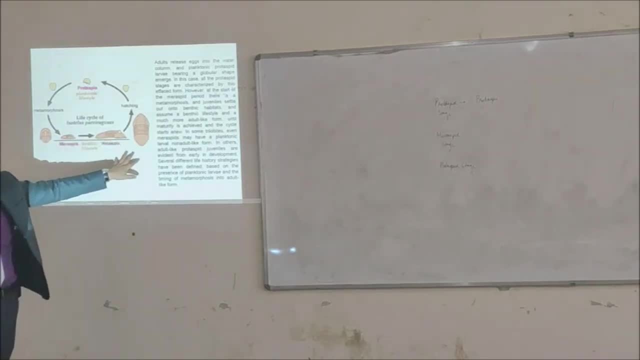 So importantly here. the dry mobile could not hedge in the menace principle. They would hedge only when they become addicts. They would produce gametes only when they become addicts. So this gametes, they were fused together, gave life cycle. 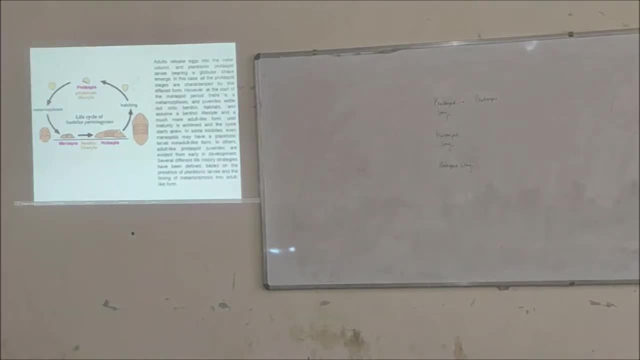 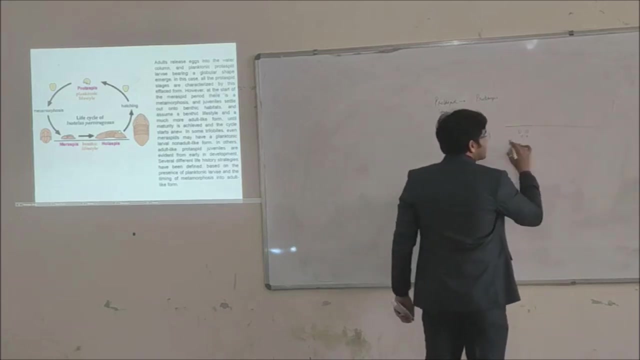 The mawaar has same life cycle. Life cycle, can you, Is it okay, Sir? there is three causes for water. What are they? Something which floats in the water. This is the water, And these are those larval stages. 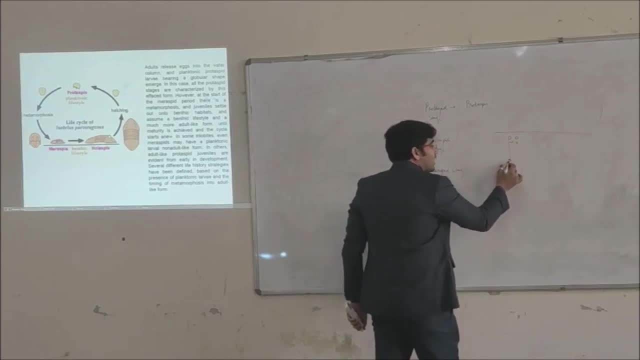 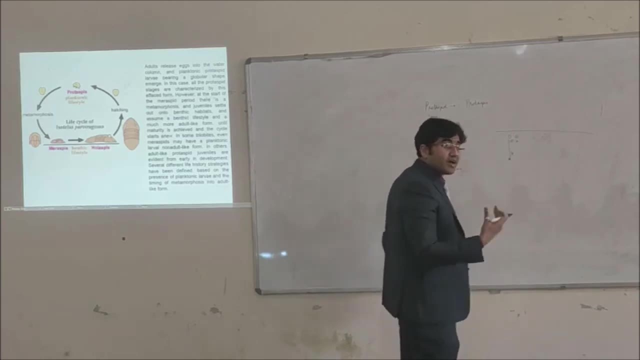 These are the particles which are floating in water. They cannot go down because they are planktonic. They are planktonic, So what could they feed upon? They need food for growth, for survival, So they could feed upon these particles floating in the water. 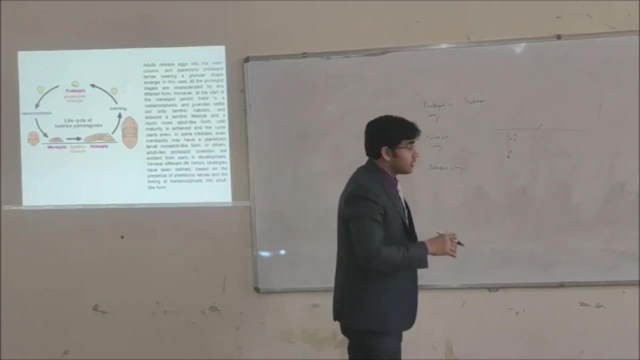 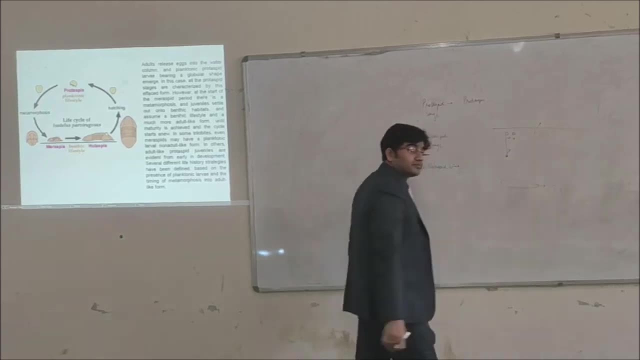 Tyrosols, or those food particles, soids, which are there, But once they become benthic creatures and they start to move, they will eat the material which is here on the sea floor. Okay, The detritus feeders. 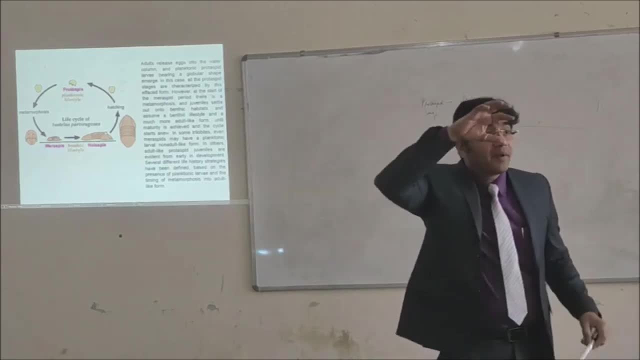 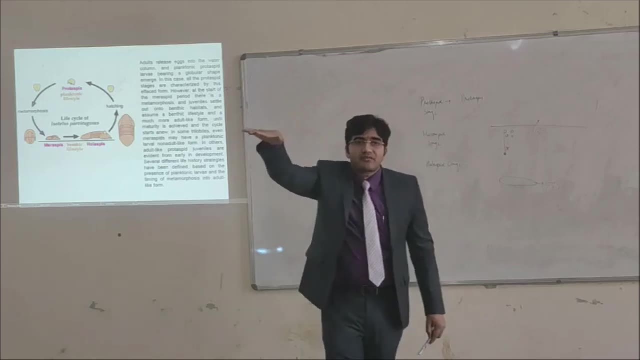 What is it? Detritus feeders, Detritus feeders, So planktonic feeders, water planktonic feeders, ones which cannot go down, they have, They live in the water surface. They are the plankton planktotrophic. 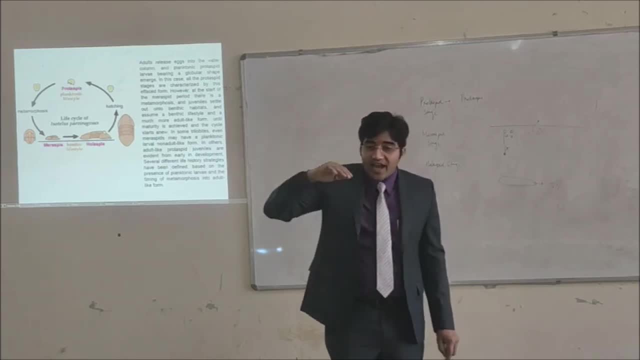 Planktotrophic, Okay, But those which have, which can walk on the sea floor, they are detritus feeders. The detritus feeders, the detrital material left over, material which is like on the sea floor. 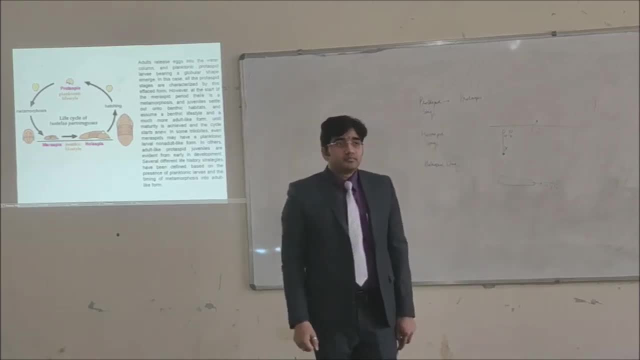 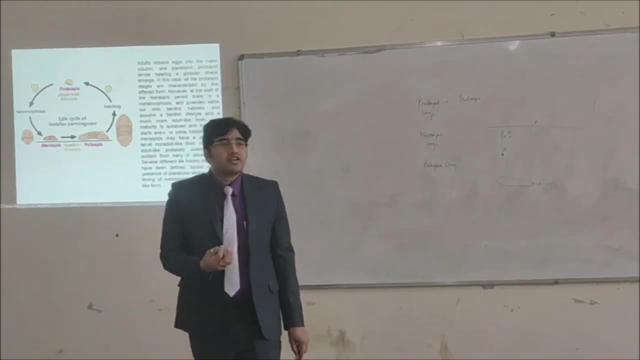 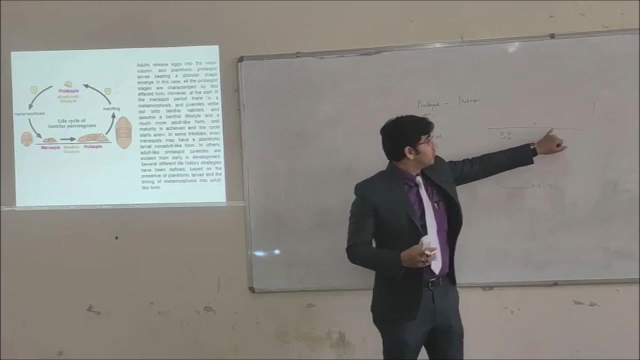 they will be eating that. Okay, Sir, it means the term from Bhagavad Gita, Karmika. No, No, Doesn't mean that. Why can't you have the vegetal material falling on the sea floor? You have the the vegetal portion here. 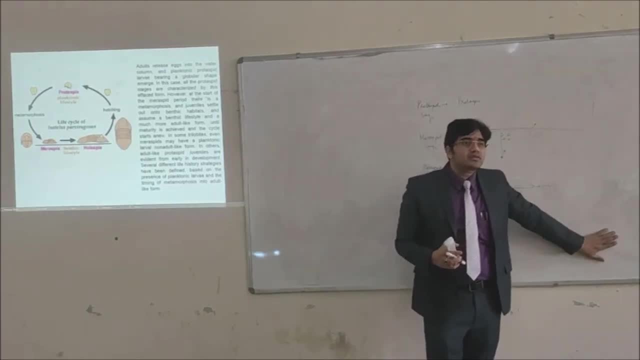 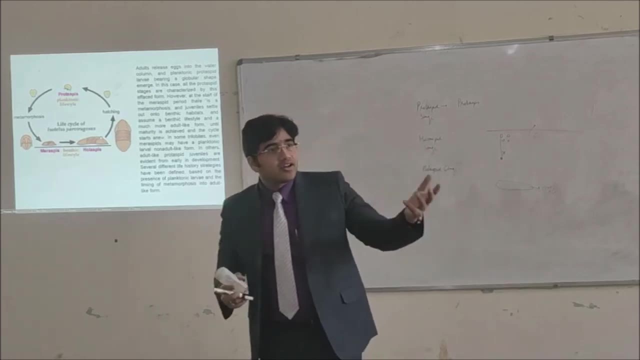 Once they die they will go on the sea floor. The detritus feeders. Okay, Planting kya? Are there not zooplankton? So organisms eating those zooplankton, are they herbivores? 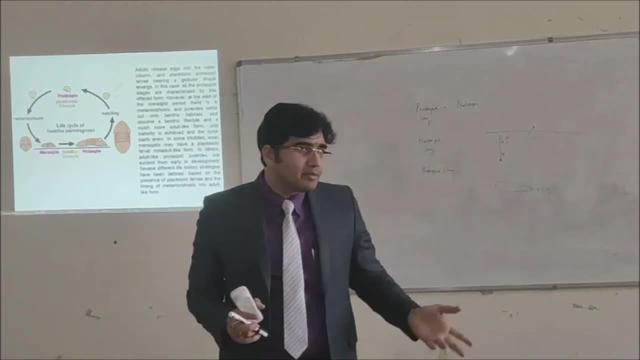 No, they are carbivores, but they are eating plankton. Then you have those vegetal portions which are falling on the sea floor as detritus, detrital material. something is eating that. If it is eating plant material, is it a carbivore? 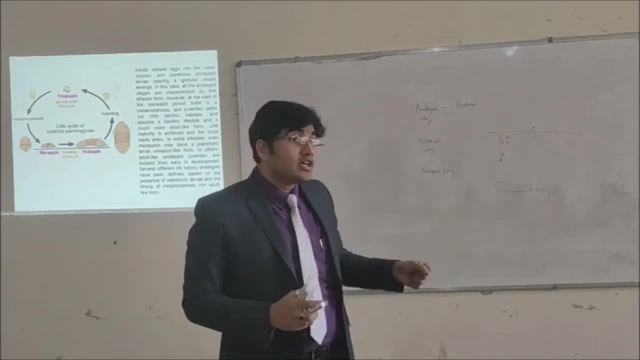 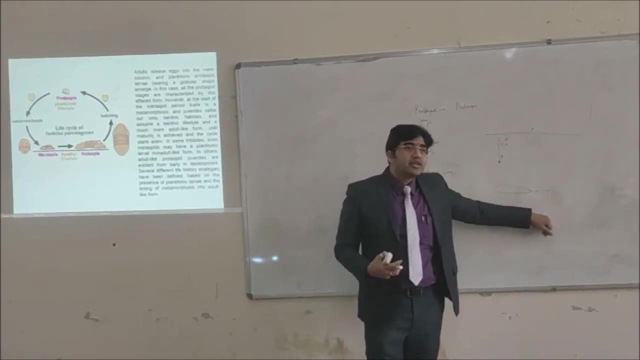 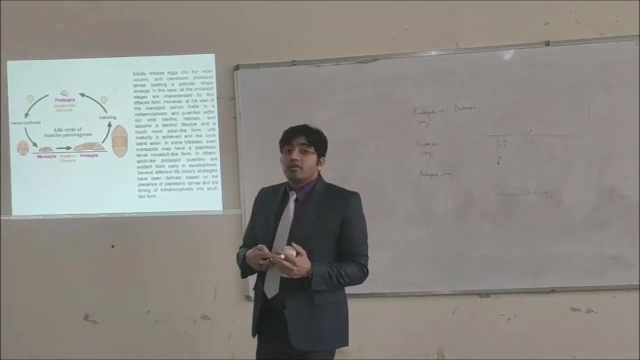 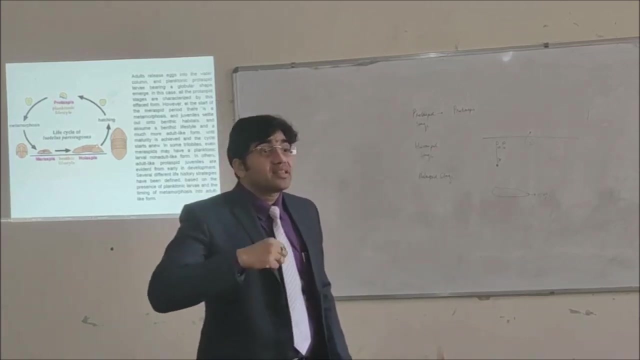 No, So detrital feeder, filter feeder, planktotrophic, all these are terms which are defined on the basis of plant material. Okay, They have defined out the basis of the method by which they intake their food. okay, Chale aage. 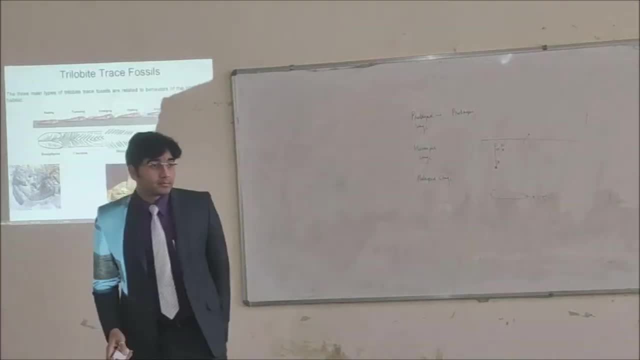 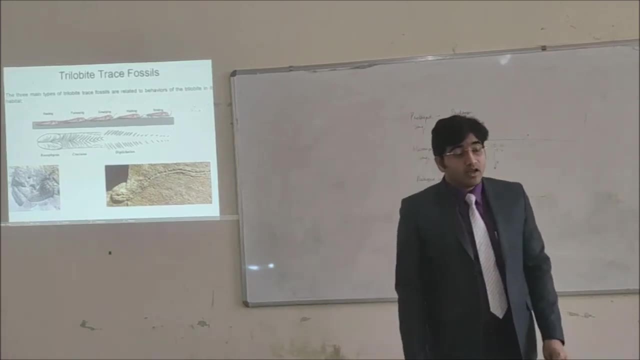 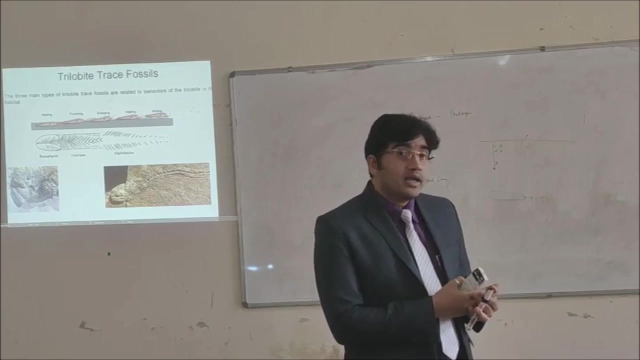 Sir, The basis of food. The basis of food. They probably show both. Yes, Once the gametes fuse. once the gametes fuse, you will never have asexual sex. Remember: evolution can never take place by asexual reproduction. 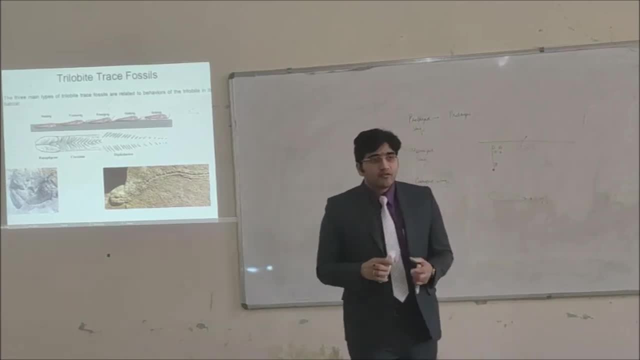 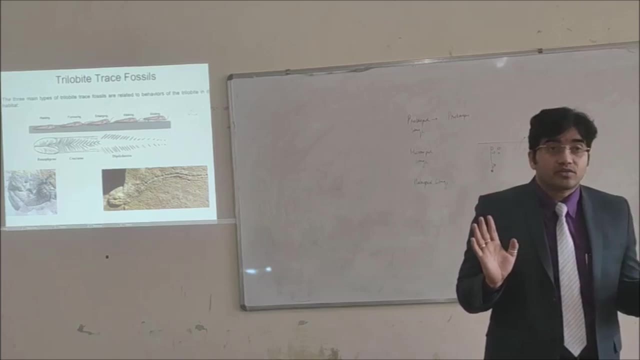 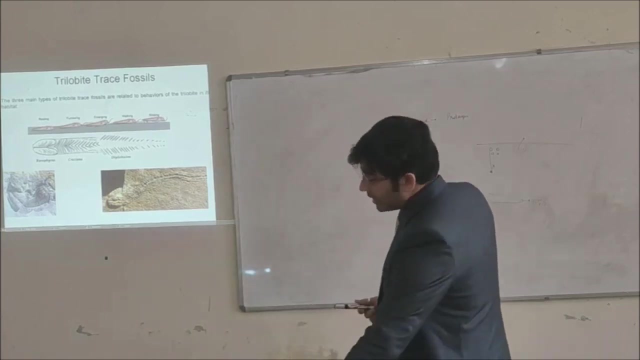 It has to be sexual reproduction. Keep this in mind. Fusing of the gametes is either in-situ or ex-situ. is a sexual reproduction. Okay, Alright, Now. depending on the lifestyles of these biobites, there are different trace fossils. 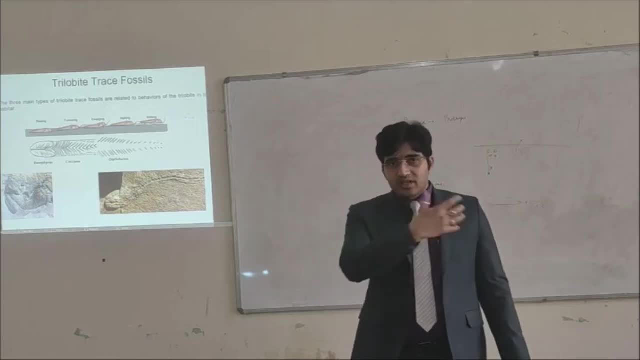 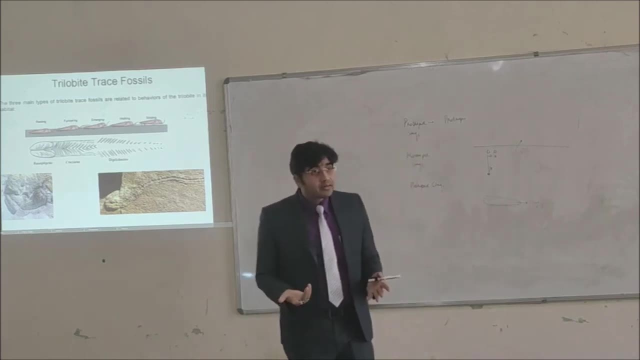 that have been seen. We have seen till now by the morphology, that chalobites had legs. It means they could walk, They could run And they could sit at some place. So how is trace fossil defined By the definition of fossil in people? 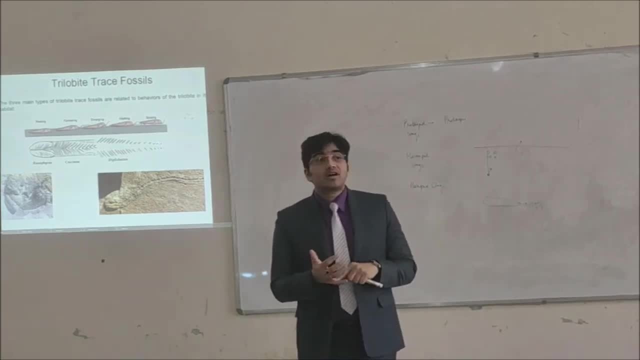 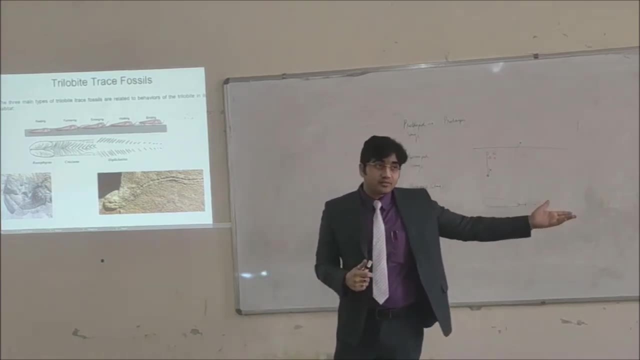 What is the definition of fossil? It is a naturally preserved remain of the body parts of organisms or their behavioral patterns. So if the behavioral pattern is preserved, which should be at least 10,000 years old, So on that basis we have derived body fossils and trace fossils. 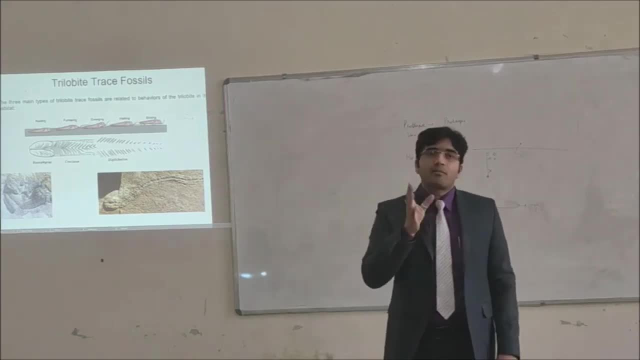 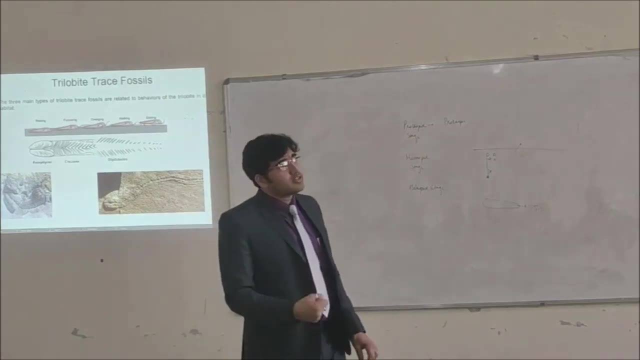 Body fossils means the remains of the body. The carapaces are the body fossils, But the remains of the behavior, they are the trace fossils or ethno fossils. The triobites: they show three types of ethno fossils, Three types. 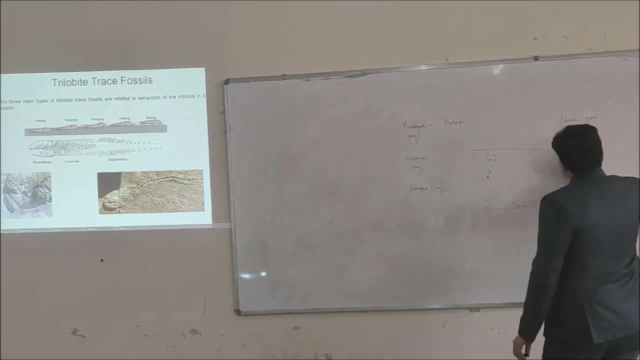 What are they? They are. if a triobite is sitting somewhere, If suppose this is a triobite, it is sitting somewhere on the soft mud And then it moves away, leaving behind a depression. Leaving behind a depression which was intruded by the sediments. 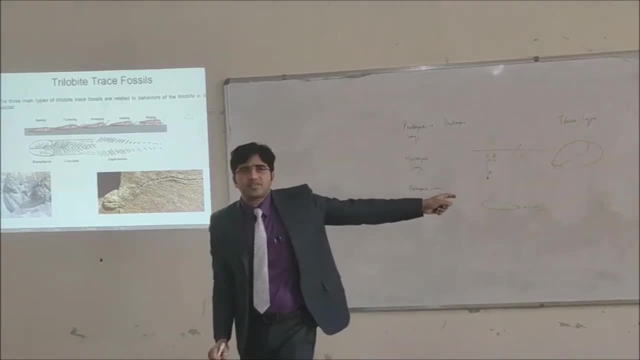 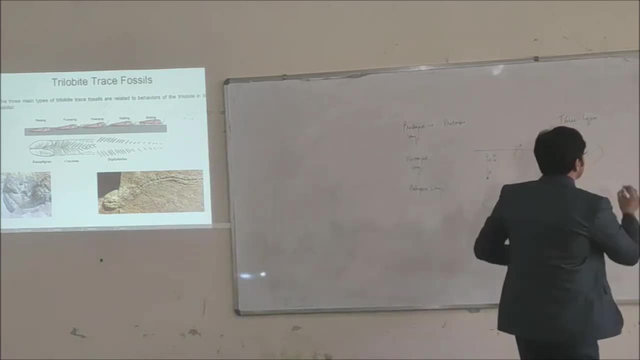 And this can be seen, that it probably is made by a triobite. This was one depression means it was the resting trace, Resting traces, Resting traces And the resting trace fossil of a triobite is called as rusophilus. 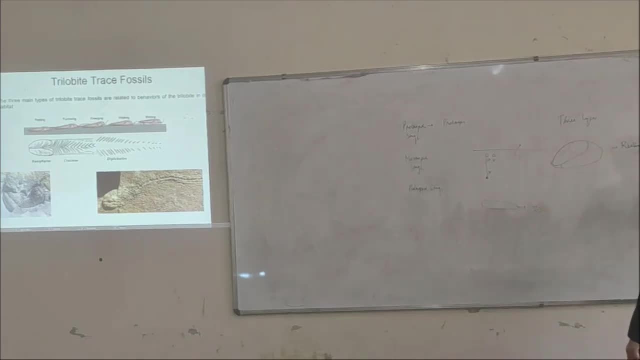 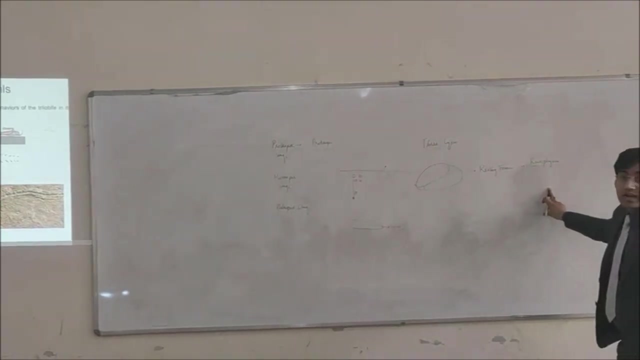 Rusophilus. This is the name of a fossil, So you will have to underline the name while writing or italicizing while typing: Rusophilus, Rusophilus. So what is a rusophilus? It is the resting traces of triobite. 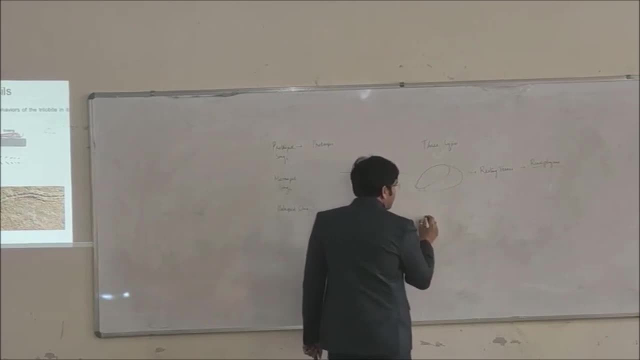 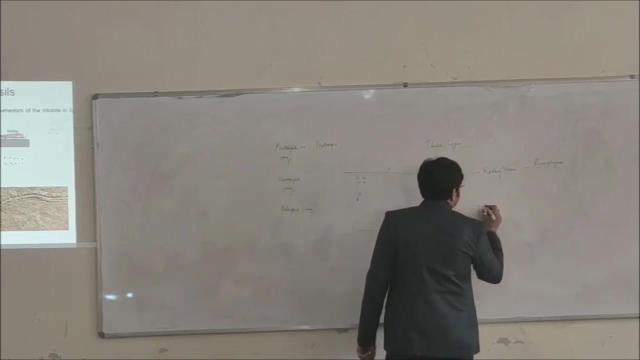 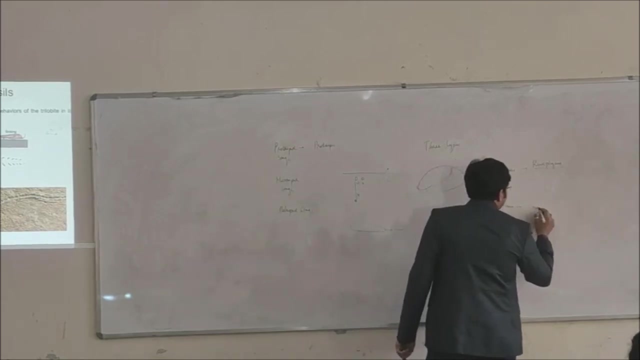 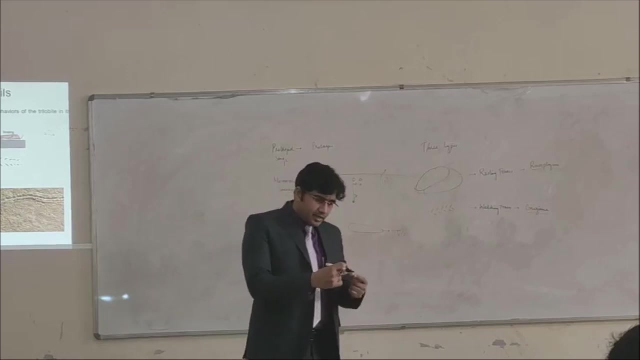 Then if the triobite was walking means it is leaving behind the footprints, The walking traces. Walking traces, We call it as cruziana, Cruziana. Cruziana, The even footprints means once you walk, you have a certain pace of walking. 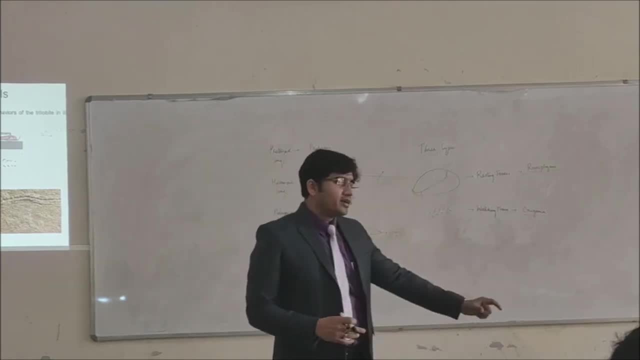 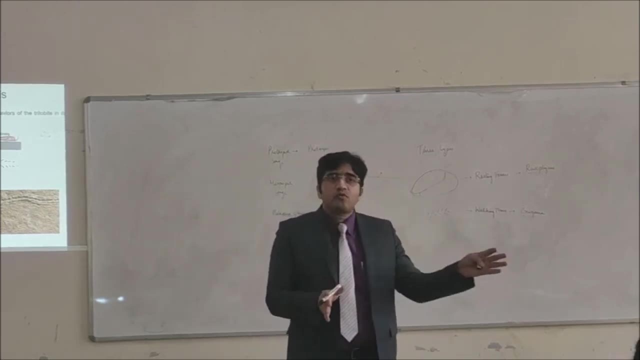 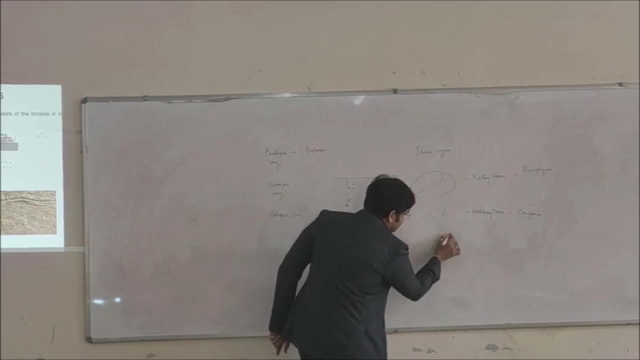 You will leave behind your footprints almost at same. you know distance equidistant, But once you start to run, the distance between two footprints increases. Okay, So the running traces. they are called as diptychnitis. 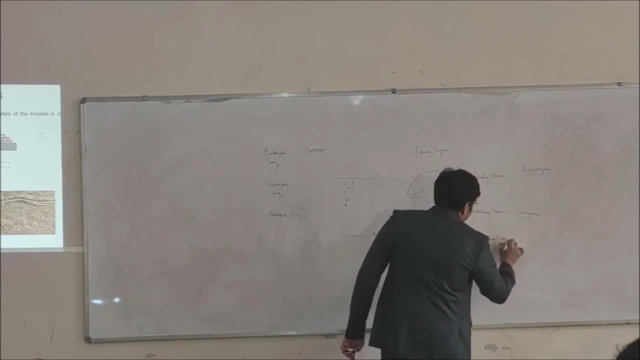 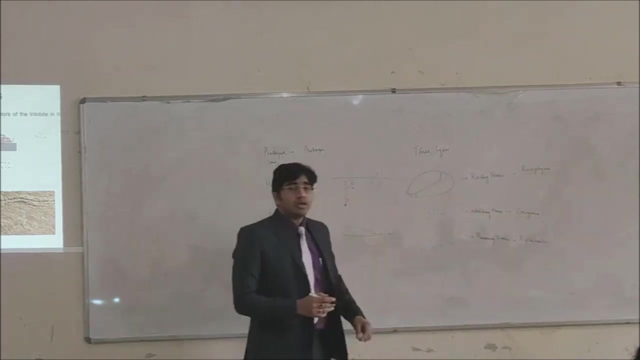 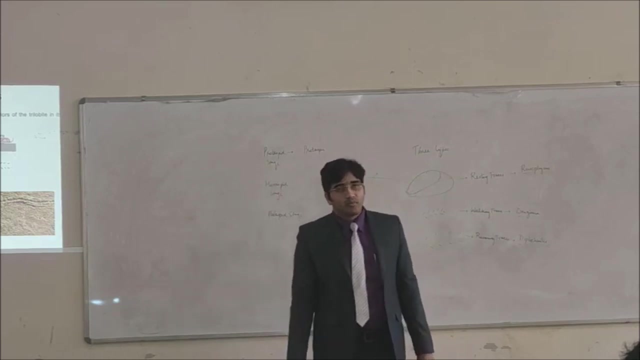 So there are these three types of trace fossils which are made by the triobites, diptychnitis, cruziana and rusophilus. Rusophilus is the resting stage or resting traces. Then walking traces are cruziana And running traces are running vehicle traces. 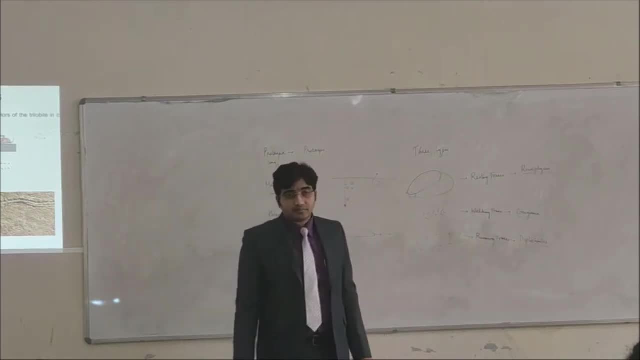 Okay, running traces are typically like this, But it is not necessary that only trilobites will make these traces. I have told you the other day that why the trace fossils cannot be used for biostatistics, Because one organism can make several trace fossils and one trace fossil. 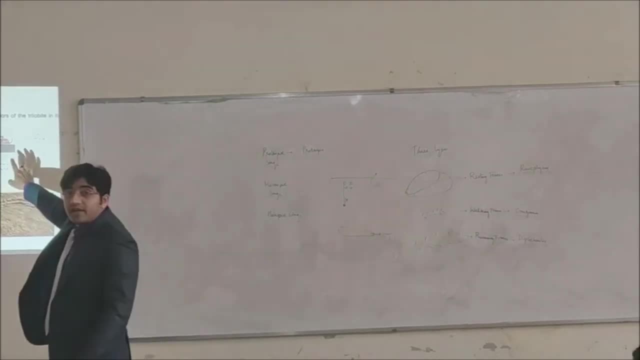 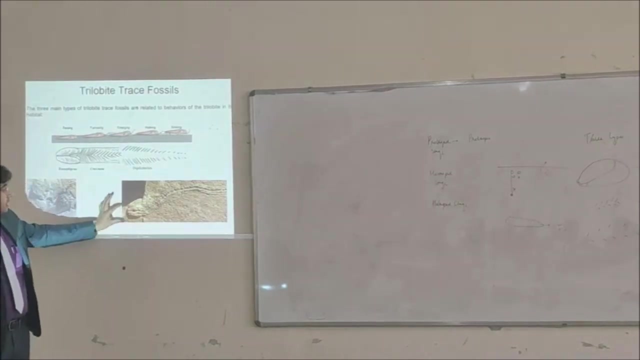 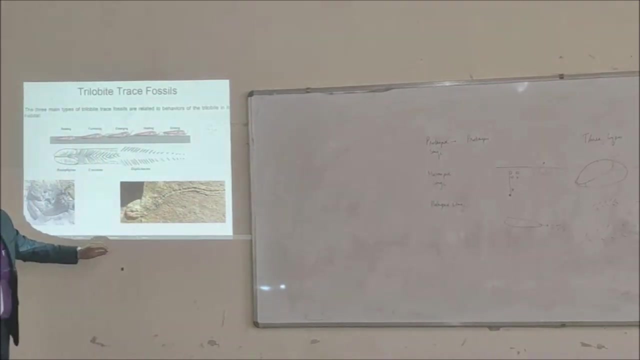 can be made by several organisms. So see here everybody that we can find this is a very good example, Very good example: Resting trace, walking trace, and this is a running trace. Very rare is it, Sir? how will this be done? What? Where you will find walking traces? 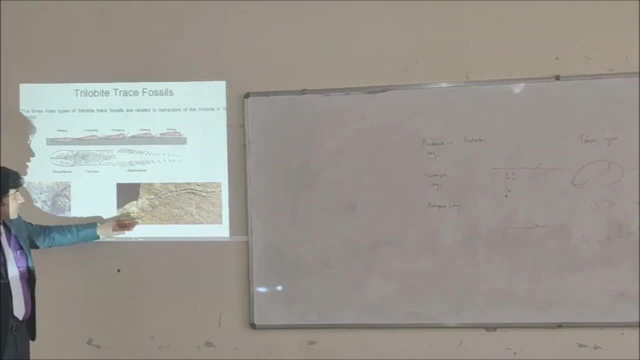 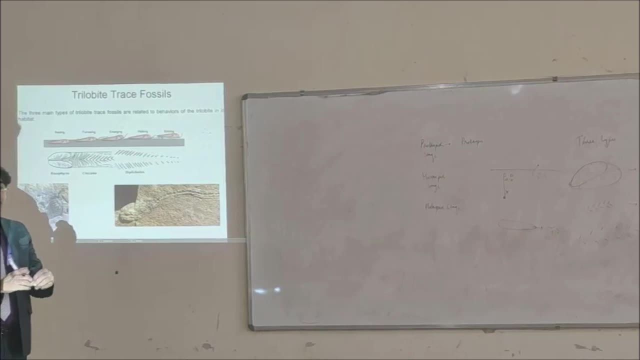 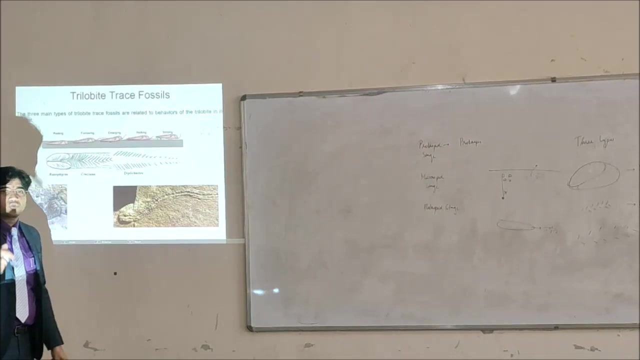 there you will find it, Even have a little bit of it. Now see this one where it is sitting. it seems to be moving, But its running traces we cannot differentiate, Unless somebody is an expert of technology of fossils, you can guess. Now, Rishabh, all of you who go to the beach, you have seen. 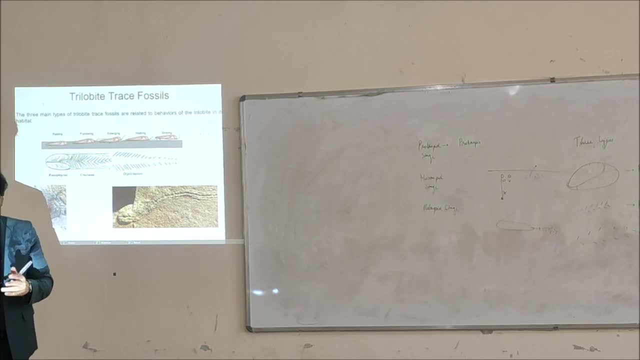 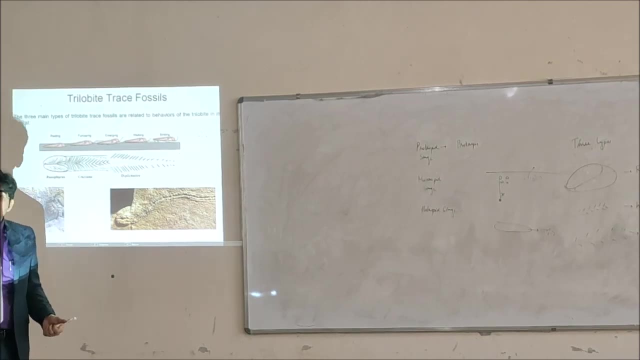 crabs. Have you seen those crabs Once they run and hide inside? where you have seen those bugs? they are different. In fact, it is only running traces. That is what I was telling you: That one trace fossil can be made by several organisms and one organism can make. 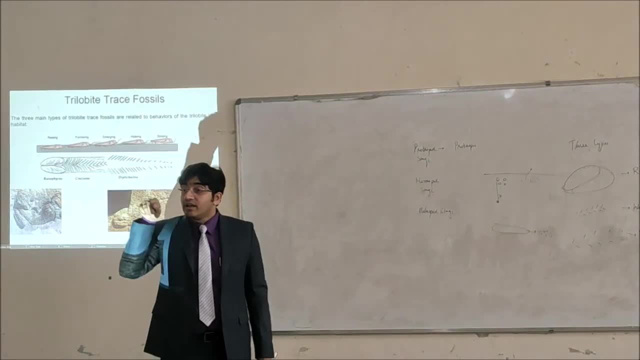 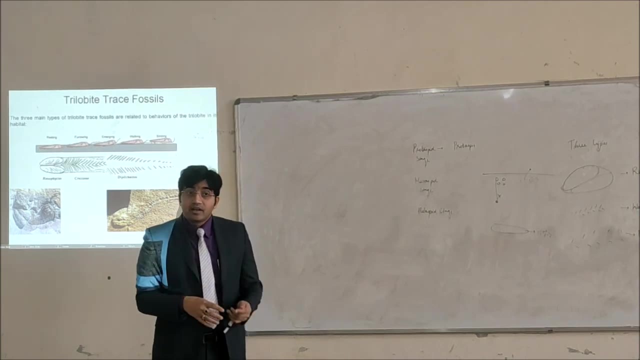 several traces. So it is very, very difficult to know this trace fossil was made by which organism. Therefore we cannot use trace fossil for various reasons. But for paleo environmental analysis, trace fossils are very good. Therefore they are one of the important tools used in the petrochemical 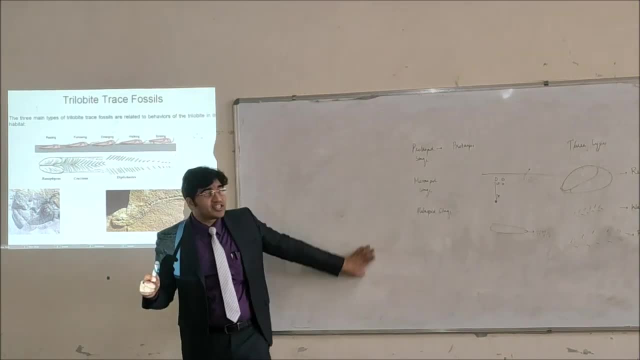 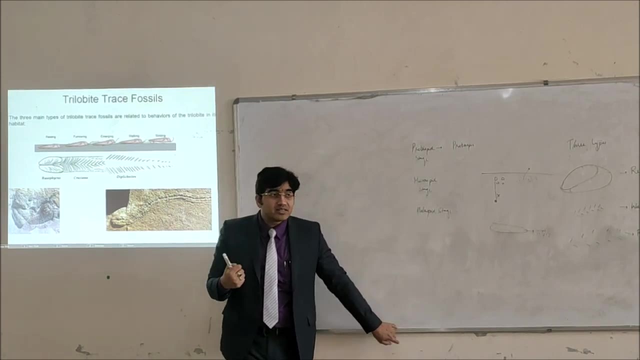 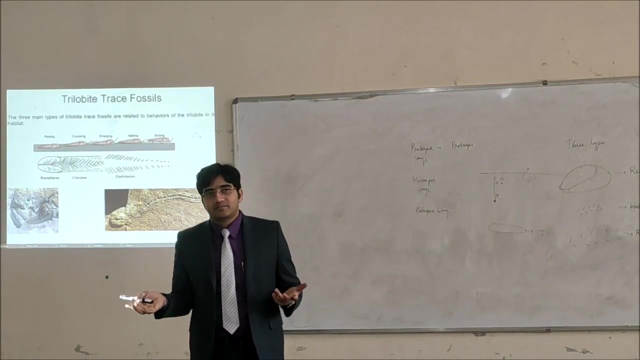 industry. So now, in the case of trilobites, if the question is asked, what are the various trace fossils made by trilobites Three? The resting traces are on the lusophilus, walking traces are on the cyana and the running traces are on the cyana. Is it ok? I mean, there is no. 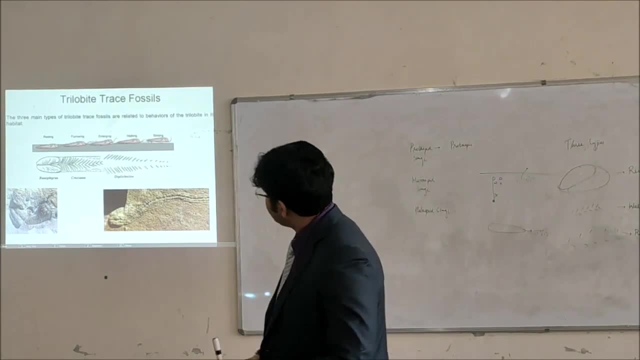 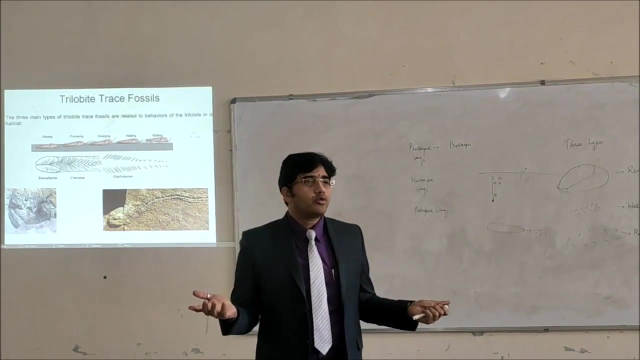 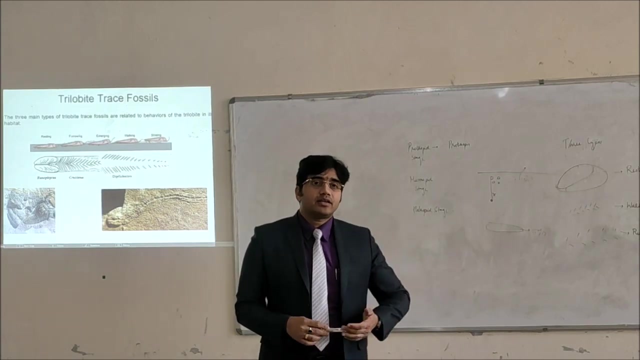 doubt, no confusion. All right, Sir, trilobites have less rate of logging or rate of running? I don't know. I don't know. There is a very good paper in Nature by Alexander, 1970. He has calculated the speed of walking of dinosaurs. 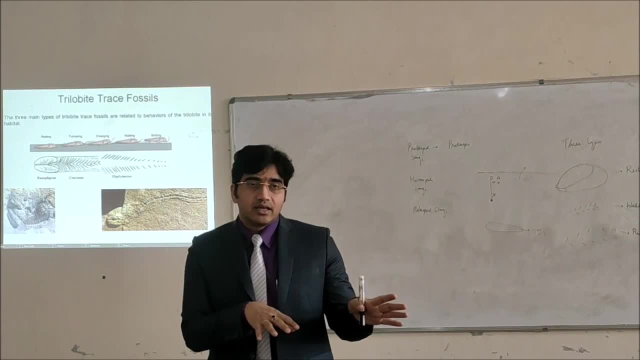 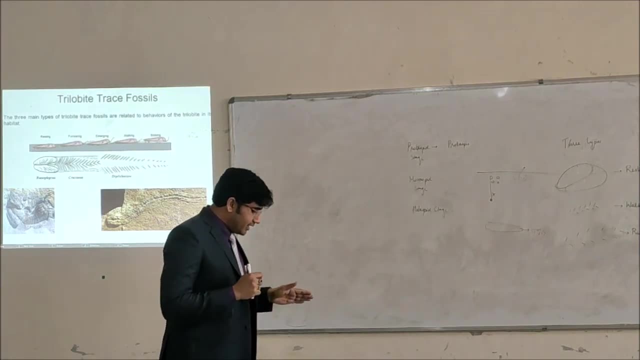 The speed of walking of dinosaurs on the traces of the footprints? Because I think that would have been because he would measure this. What did he do? He measured the stride. What is one stride? You know what is a stride? This is supposed that this is one footprint. 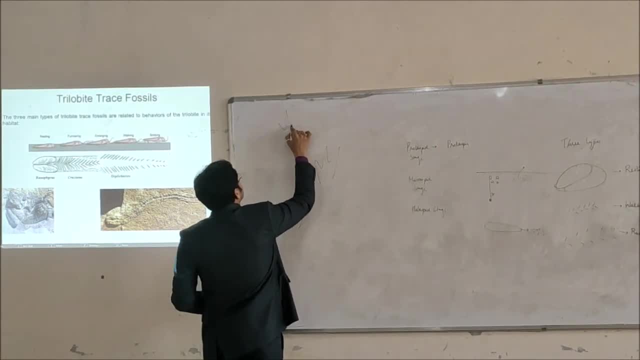 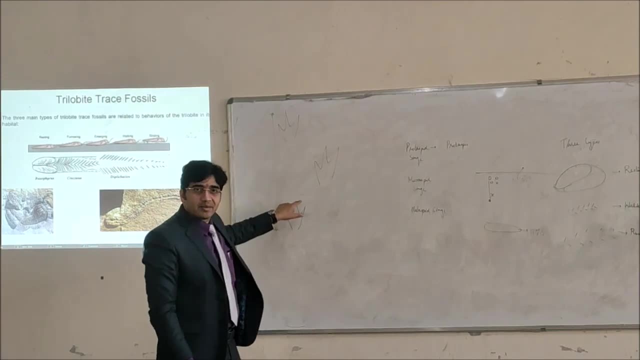 this is another footprint. this is another footprint. So what did he do? He measured the distance between the same footprints of the same species, Footprints of the same foot, same length. This is called as one stride. And then he 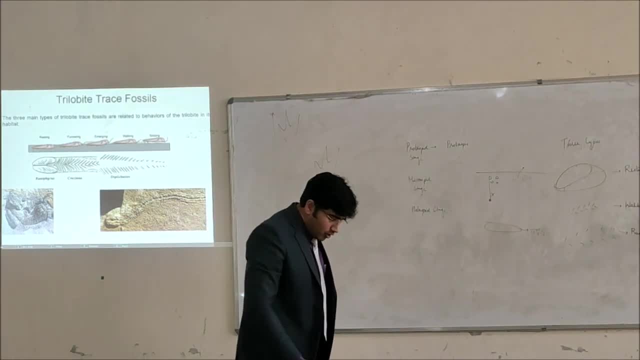 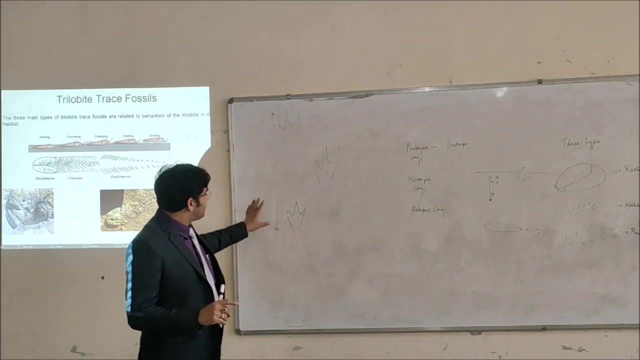 assumed. if you look at your hip height, the hip is at four times the length of your footprint approximately. So with that he derived a formula. go out with different trace fossil models that he could measure the walking speed which came out with that formula Three. 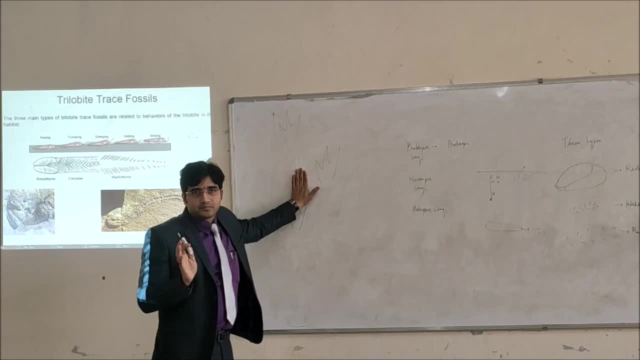 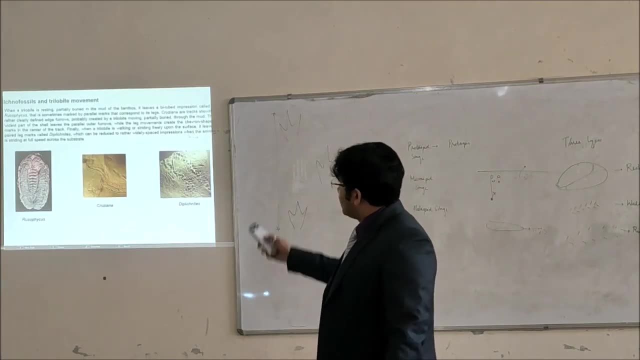 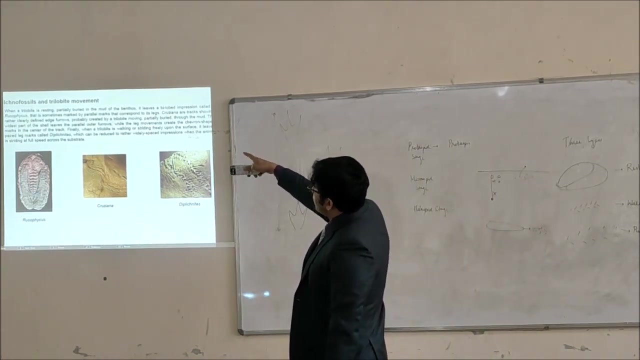 But try to find the PCD here. I am not aware of it, But yes, such exercises have been done. Alright, Equi-fossils and trilobite movements. So this is very important. By road impression. 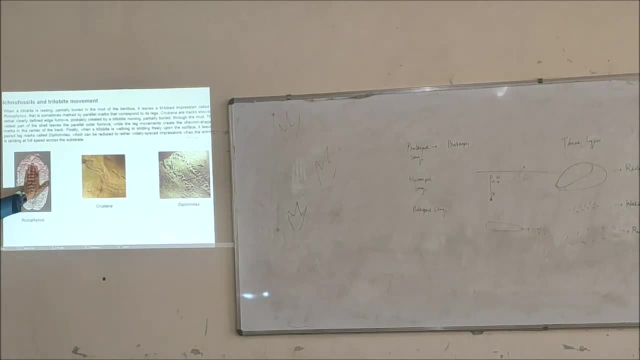 of the fighters, marked by the parallel mass corresponding to its size: Parallel mass. And then cruziana. it is the tracks we are showing, these sparrows walking. and then we have the big knight list, which is chevron chevron. you know chevron chevron. so if a trilobite 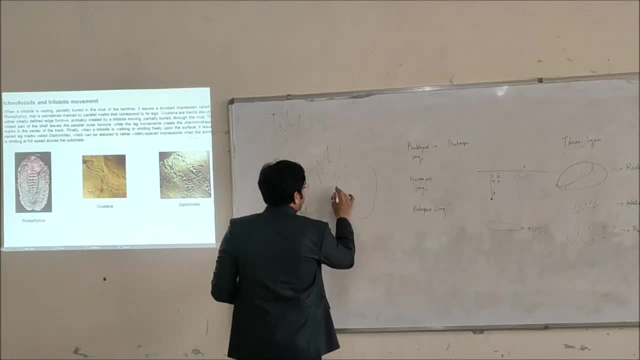 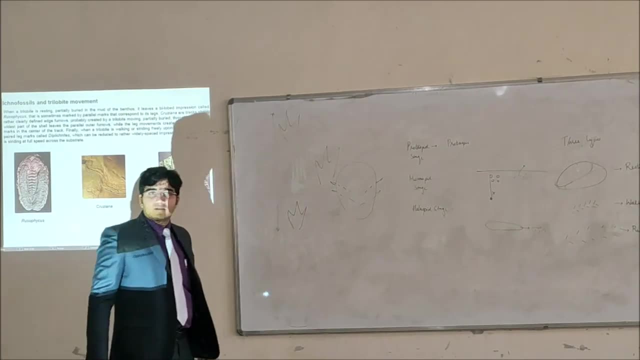 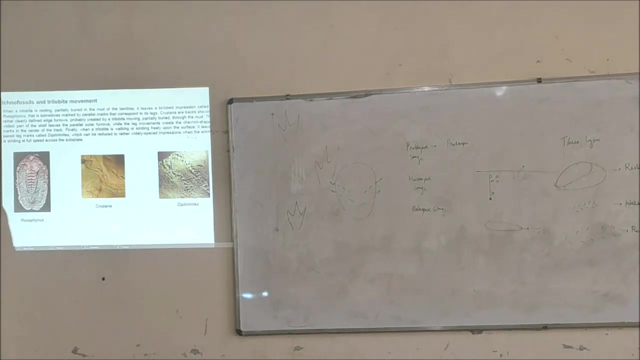 is having. let us say, this is a trilobite and its this foot is here, this is here, this is here and if it is walking, it will leave behind a mark like this, a chevron mark. ok, so, talking of these trilobites, these traces only tell us that trilobite would walk and 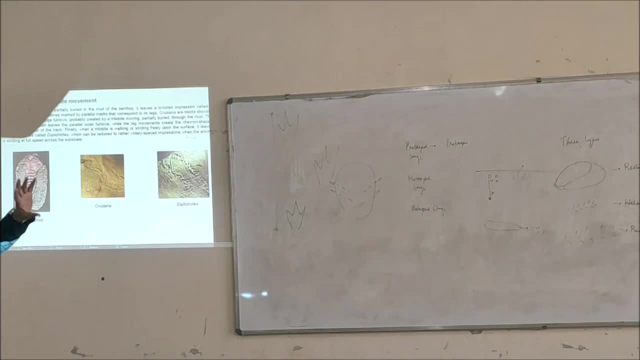 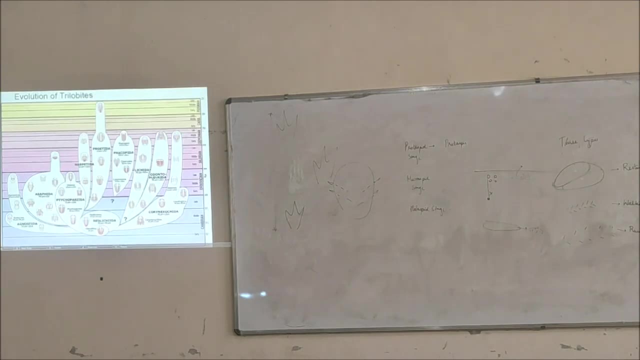 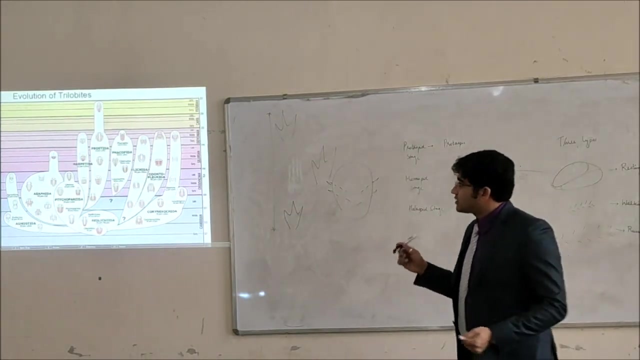 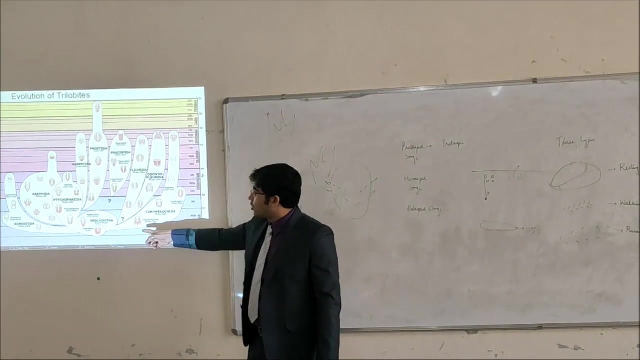 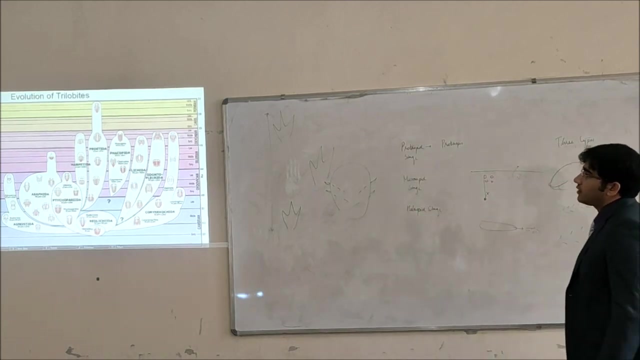 which is very, very correlated with the shape of their puddle, looks alright. ok, so we can read this, the last part: evolution of trilobites. you need to remember this evolution part, not by these diagrams, but by the means. simple example: they first was the order of red lichida and from that they diversified further. type of 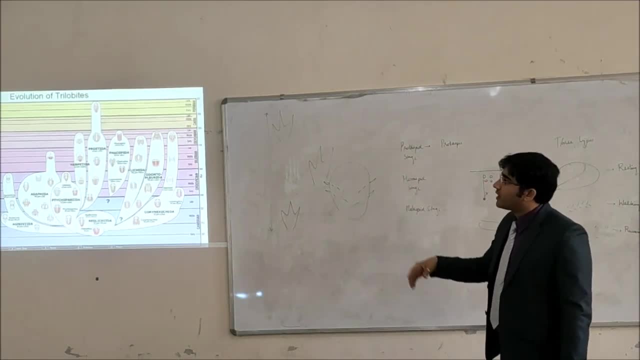 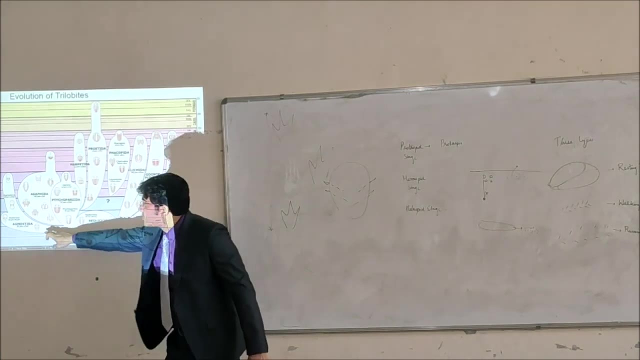 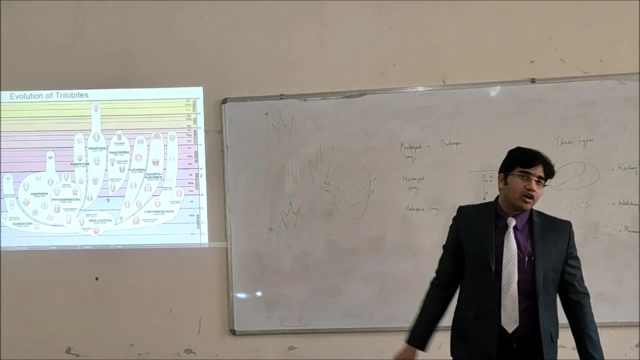 lichida. you should remember two, three things. first order, red lichida. first, blind trilobites, agnostida. last order: proetida, proetida. that was the last order of red lichida and the last order of red lichida. 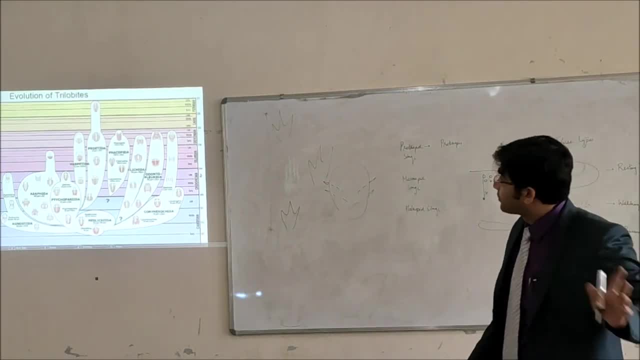 So you can see that the second order of red lichida was a trilobites which got extinct at the P-D boundary Exactly Now when we saw bioconversion. so we saw agbe zone. So they were the agbe zone. let us say that if these are the ones, so they have the most. 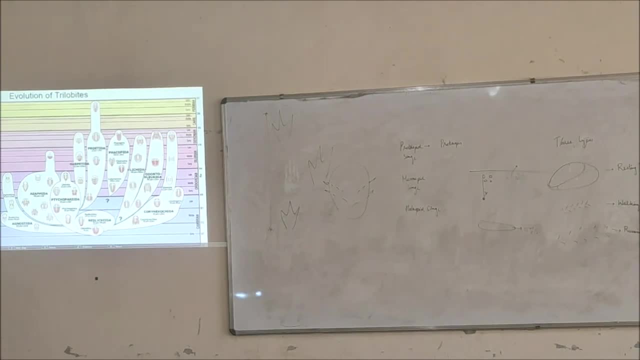 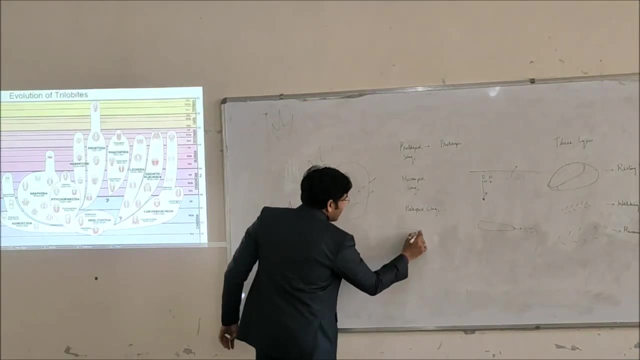 evolution or evolution. in it there is diverse education. so they started at the Agbe capri n, but from the order of the trilobites, and then they started the evolution. Now, if you see here, this is the red lichida. so this red lichida is the red lichida, and 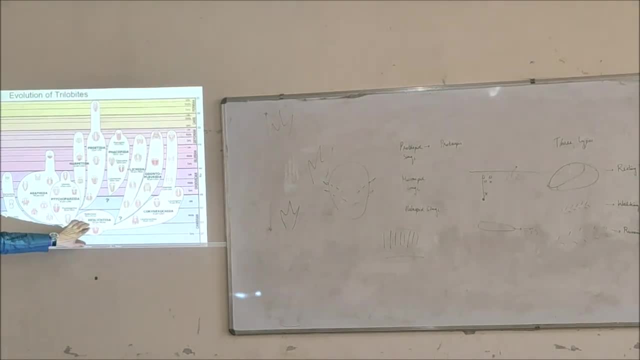 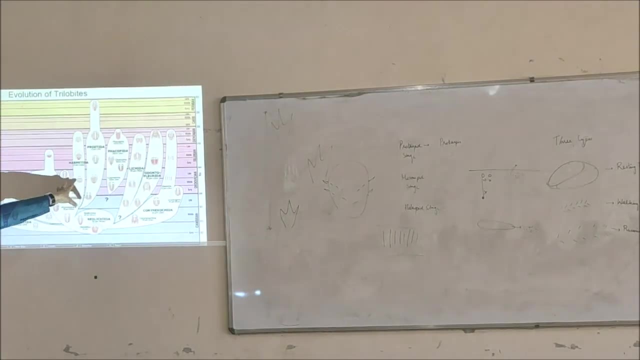 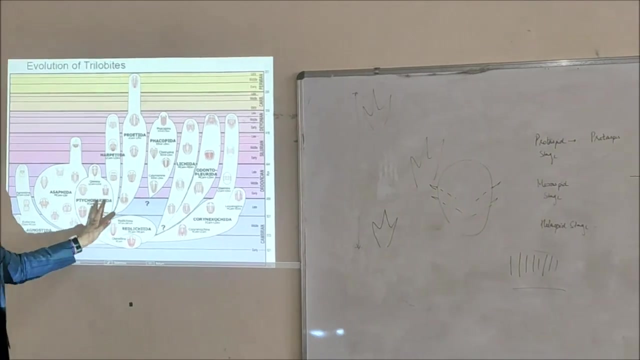 this red lichida is the red lichida, But from Ordovician to Devonian we could see that there were several orders of these thalobites living together. So this was the part. this was the portion where the evolution in the thalobites was maximum, and maximum speciation and diversification. 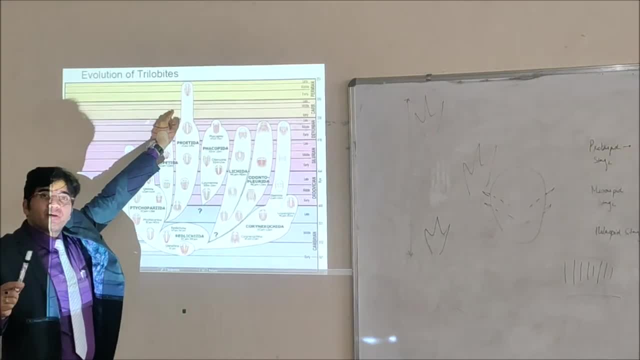 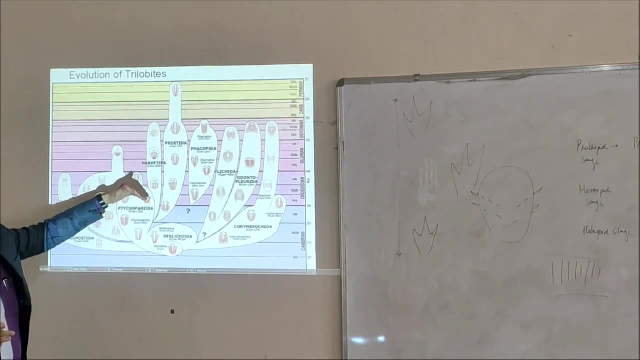 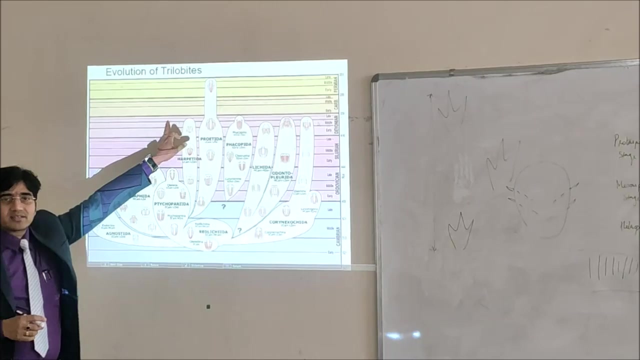 Beyond Devonian, Karni, Chakshin, Parviyana, Devizanthi, Pai had only one order. It means that the thalobites had started to decline by Devonian And these all orders. they got extinct by Devonian except the Taurida. 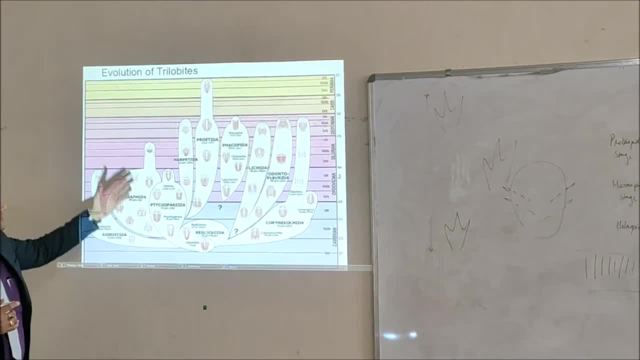 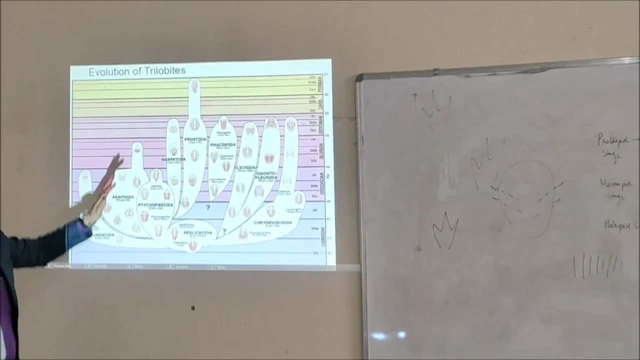 How have we known this? By looking at the rocks of these ages. these orders were not found in these rocks. Okay, So the order Taurida. it represents the last order of thalobites which survived till again and got extinct. 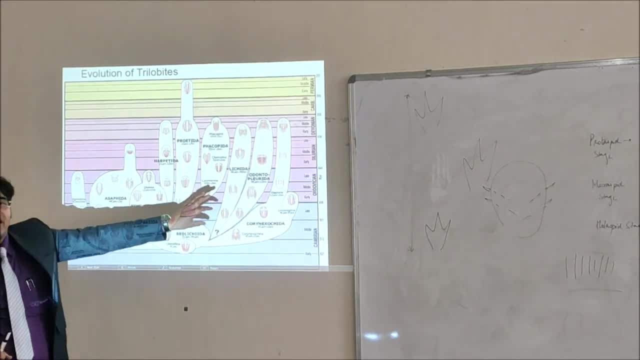 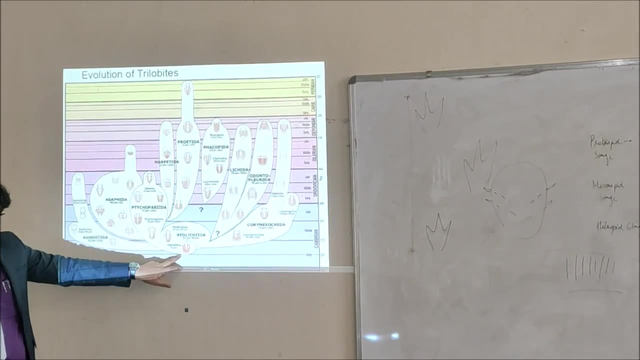 Understood. This is what makes these thalobites extinct in the next process of palaeozoic. Look at the red digita. We have it waiting As a very, very small study. I have it waiting. Agni Camelid to Manila. It got extinct. 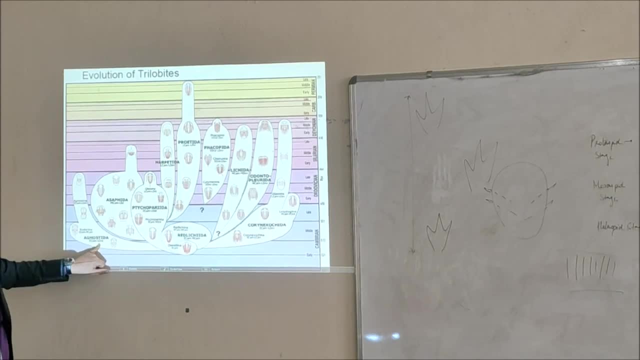 Then Agnosida. Agni Camelid to lower Ordovician, But then Agnosida. We have Agnosida. It had a branching of it. Okay, Then Esarhida Tychocaida. These were the ones which had maximum number of groups in them. orders: 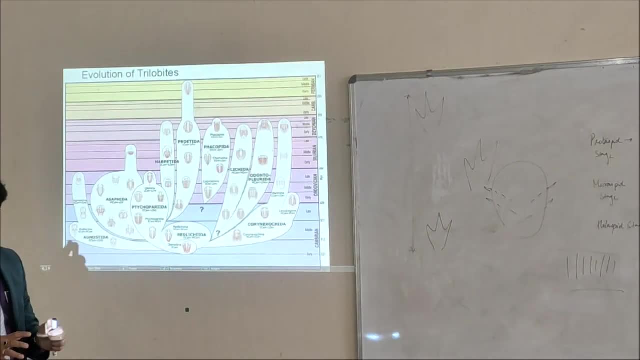 And then Phacopita Toedida. They were the ones having quite diversified, But they came later. Look at Phacopita. When did it come? It came in Agni Ordovician. Okay, So this diagram is important. 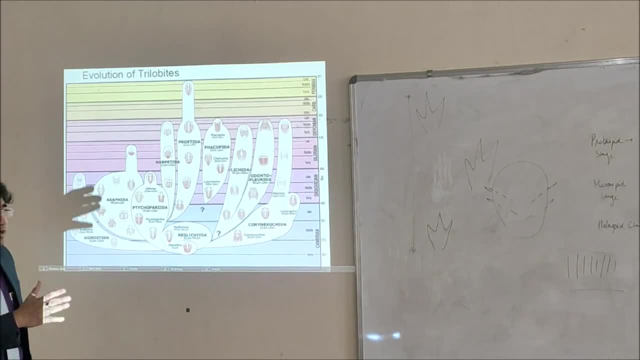 So what you will be doing in practical is also that after the completion of each group, you will take a print order of this Or you will make this diagram And attach in your practical journal So that you know continuously when you look at it. you will know what is the geography. 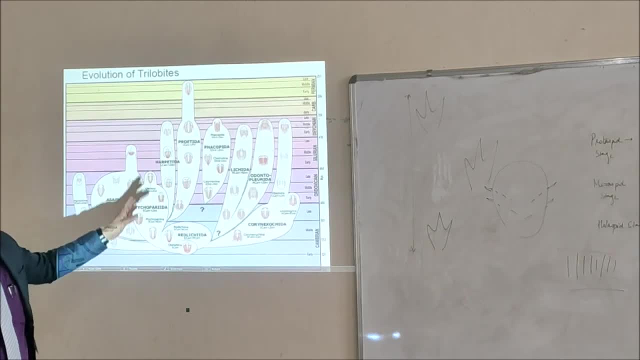 of it, Because this question is very commonly asked. This is the same thing here: the Geological History of Tural Bites. The question is: what is the geography of the fossil groups, The Geological History of the Fossil Groups? For example, that the Tural Bites, their ancestor was Salmon Covina, which was a pre-Cambrian. 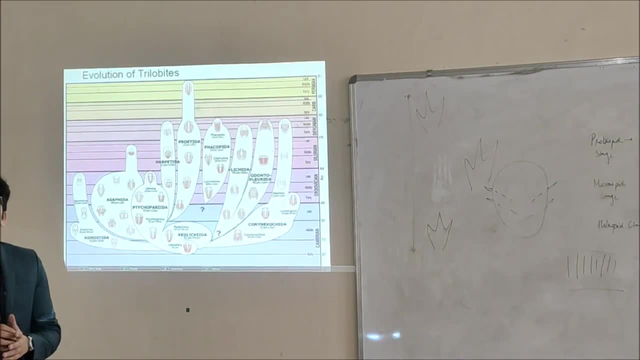 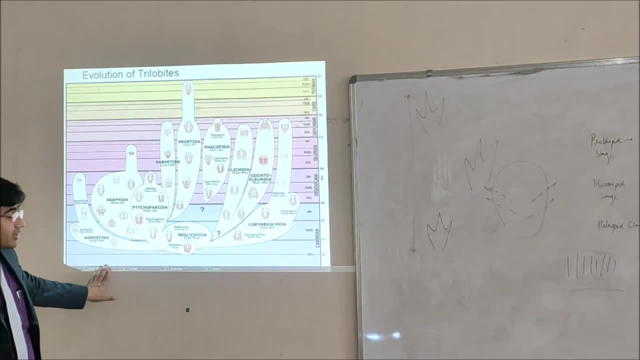 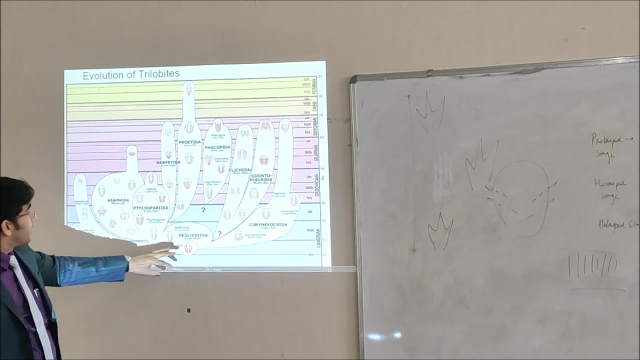 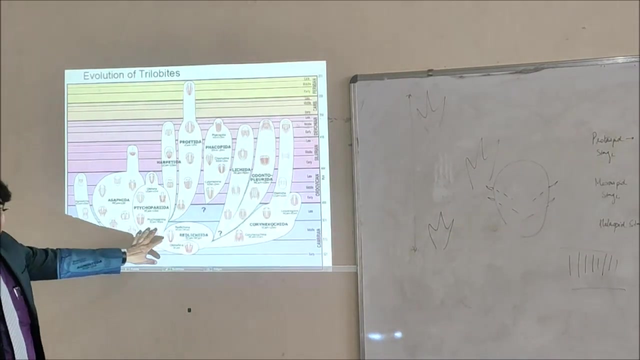 It was a soft-bodied Metazoon Which got segmented into the first order at the Abhi Kameh, which was Red-Vichita. It further gave rise to the different groups together. So if you look at Adgnostita, Corynexichida, Typhoperida, they all came at almost same. 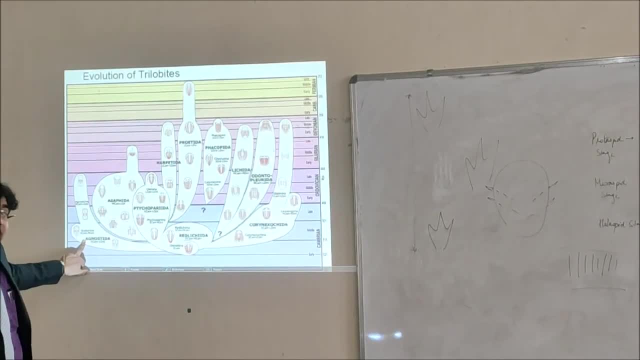 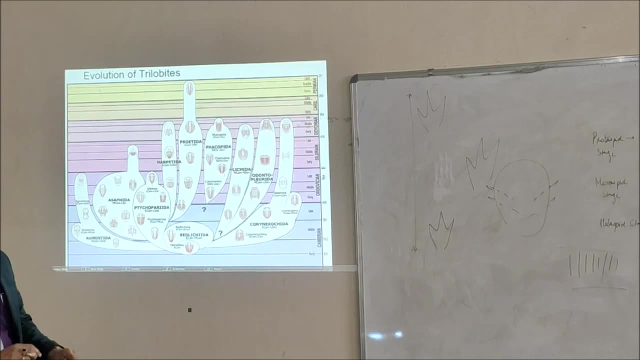 time. So in this these were the vimals primarily. So, if you look at this, they were started from the US. So it is not only the environment, but also the life habits, their genetics, their use of several organs- use or disuse. 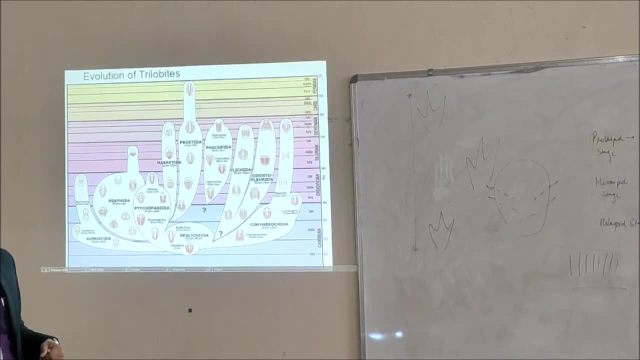 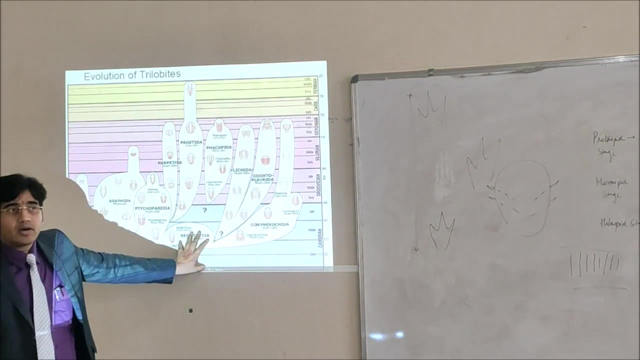 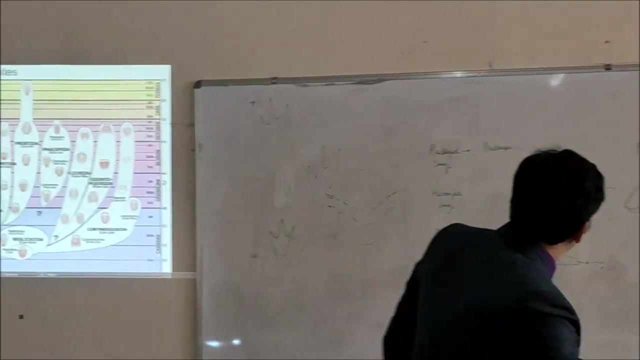 So if you do not use an organ, it will be lost in the due course of time as a part of evolution, Understood everybody. So this completes our class on the trilobites. A few more things are there. They say trilobites used to show a few features. 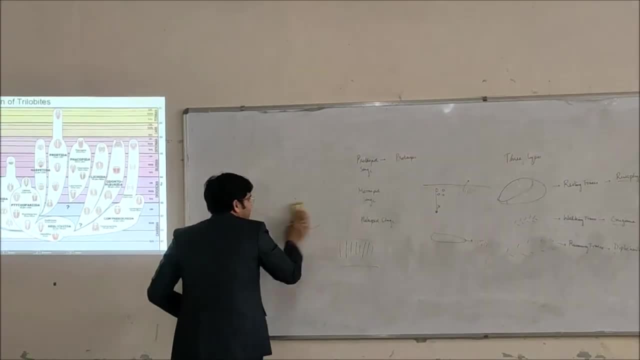 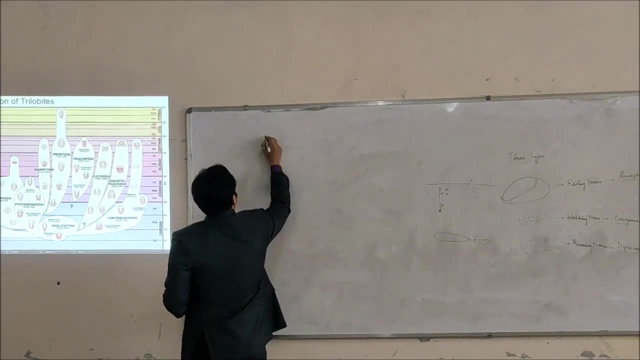 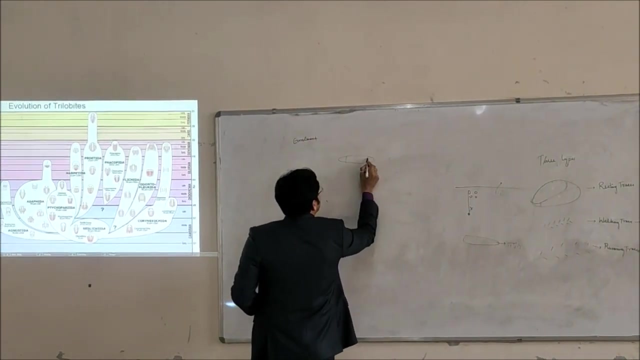 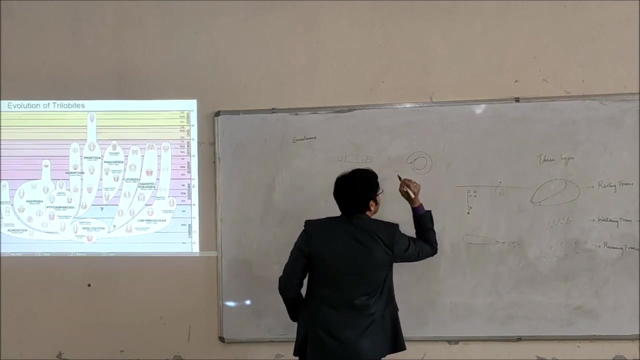 Let us discuss a few of them. There was a lot of enrolment. where these habits enrolment? What was enrolment? That if this was a trilobite, It could enrol itself, like in a spherical shape. Like this: It could enrol itself. Why did it do so? Probably to protect itself from its predators. Imagine that a fish is coming and it has its vision that I will find a wide space, I can eat it. But if you enrol yourself and cover yourself in a spherical form, 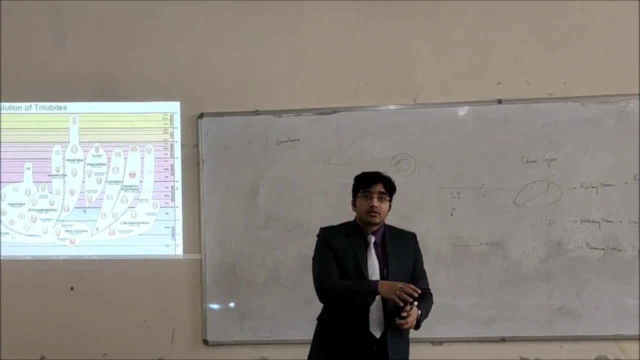 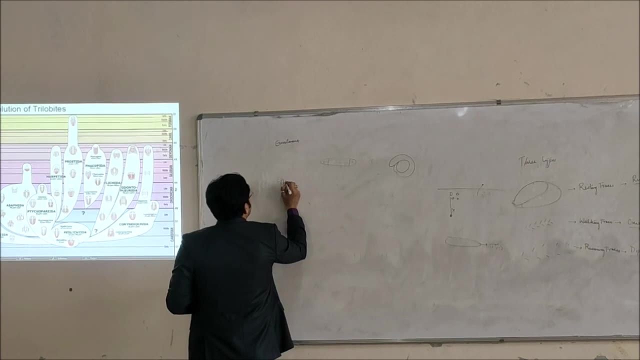 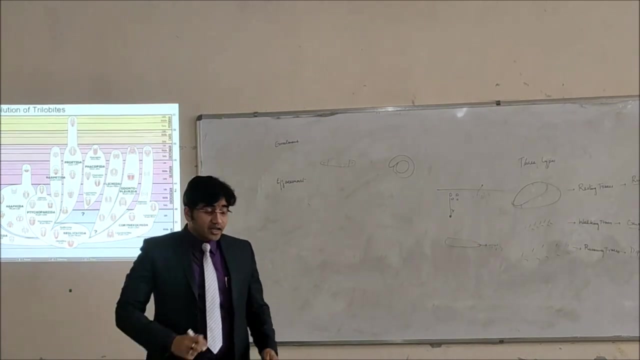 Then it is possible that It may avoid you Thinking you are quite a prey. Second, Effacement: Effacement, So another property which was shown by the trilobites. What was effacement? Effacement was a property in which all the features of Cephalon were wiped out. 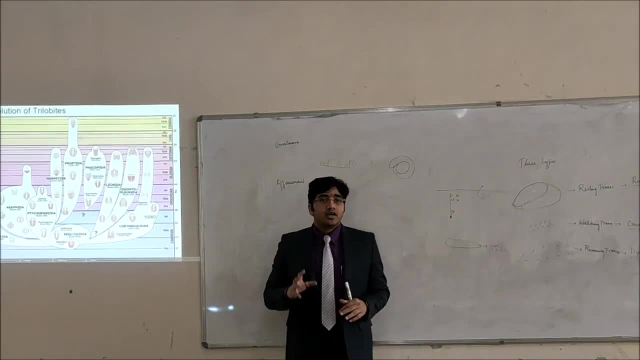 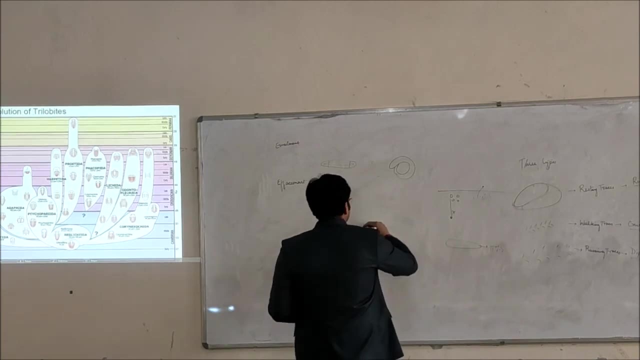 All the features of Cephalon: No facial suture, No glabellar furrows, Nothing. It was simply. It used to look like A kind of A. You know. Just this way, Sir, It looks like Kachua. 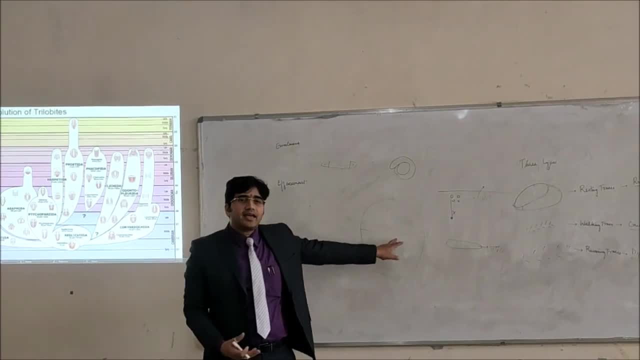 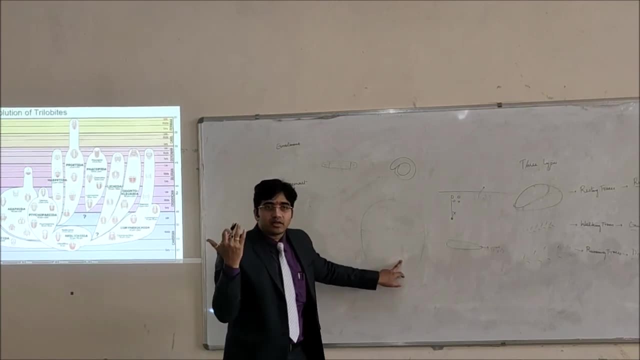 Yes, Now you will not be able to understand what this is. We also don't understand what this trilobite is. But imagine for its predators, Effacement, No features of Cephalon. This is also a property which was shown by the trilobites. 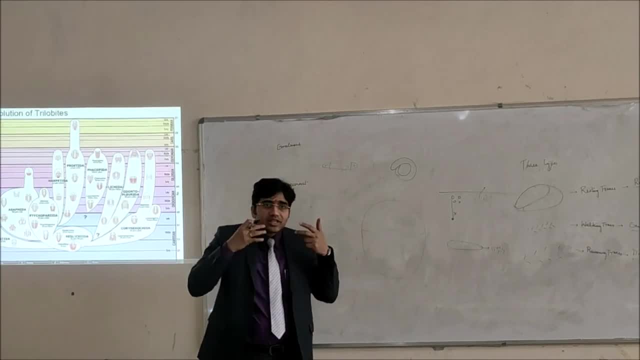 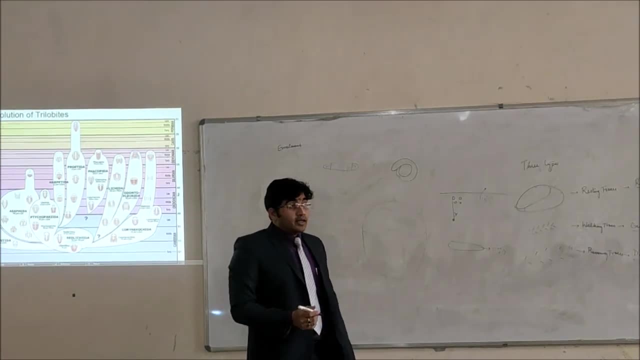 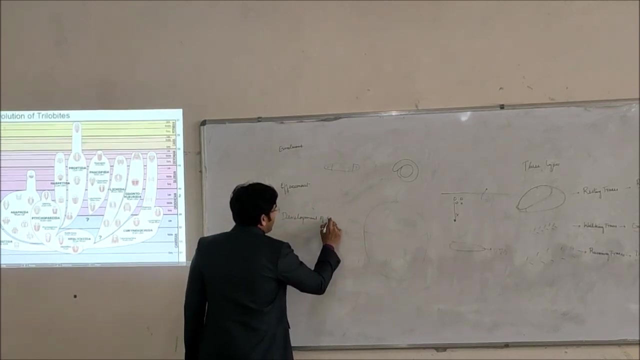 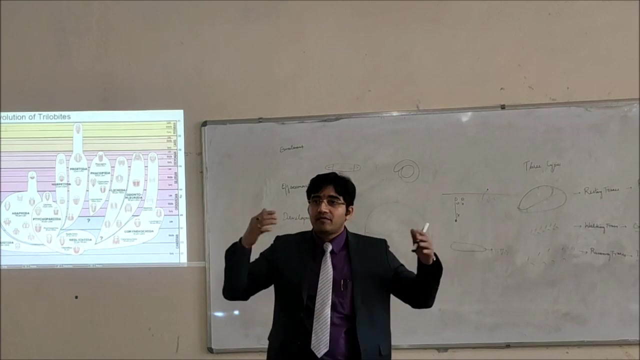 Just a little bit. inside, All the features are gone, No furrows, Nothing, No articulation. It is gone Because Then development of spines, Development of spines on whole body, Whole carapace, So suddenly you will see that trilobite carapace is having several spines on the body. 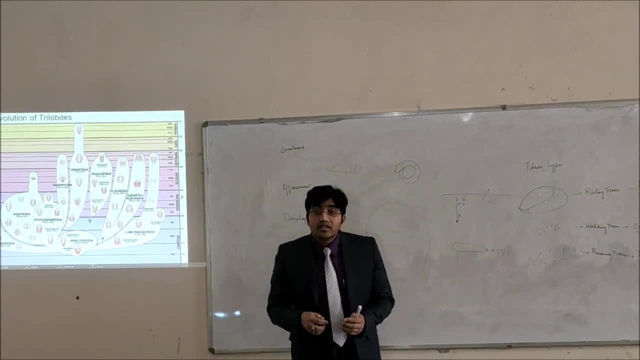 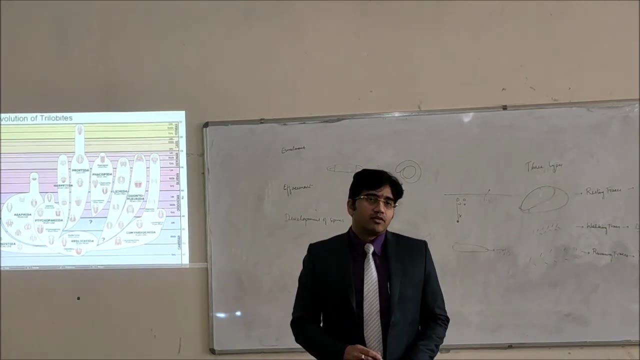 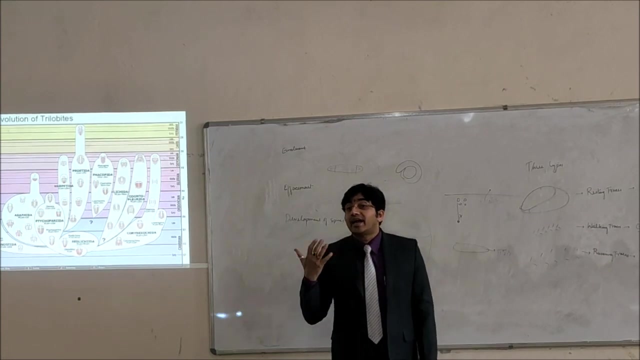 Probably to scare away its spirits. Okay, So these are all the various sustaining mechanisms shown by any organism And probably also shown by. So from today's class, what questions you can take? of course you should know how to draw the dynamics of trilobite keratosis. that is very important. 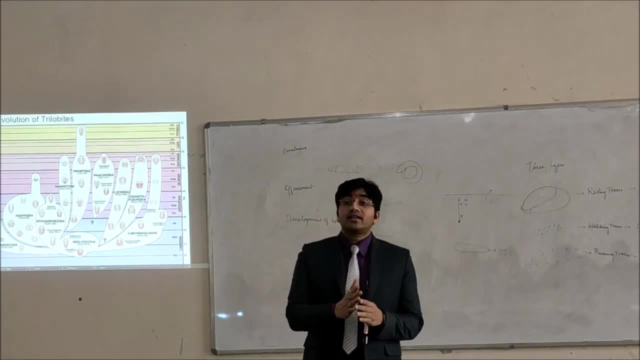 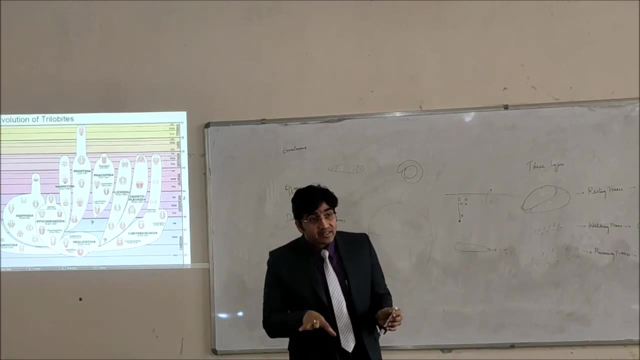 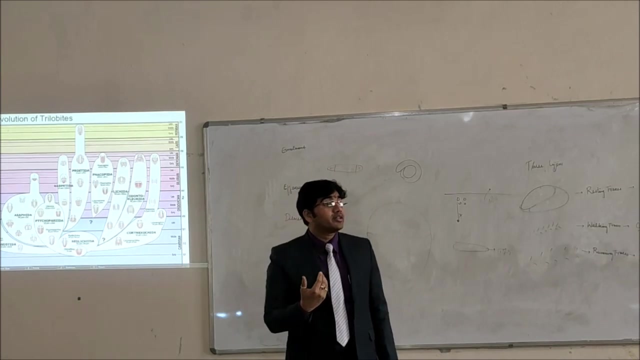 Then what are the various stages of development in the trilobite? So the life cycle you have to draw, discussing the pulaspis, medaspis and pulaspis stages, Then you can get questions of what are the three types of eyes in trilobites. 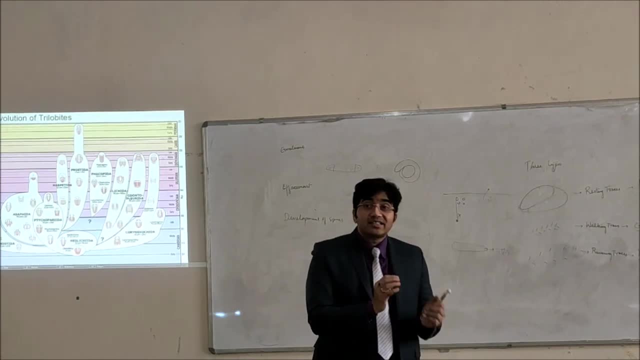 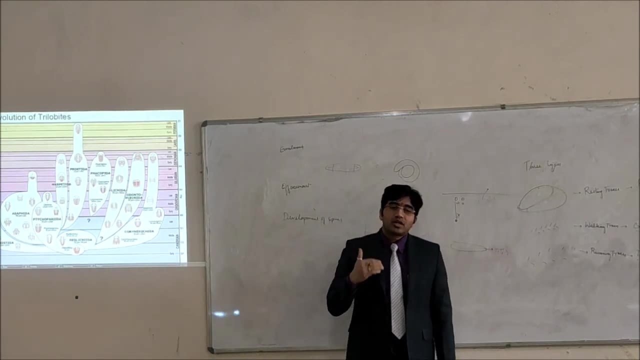 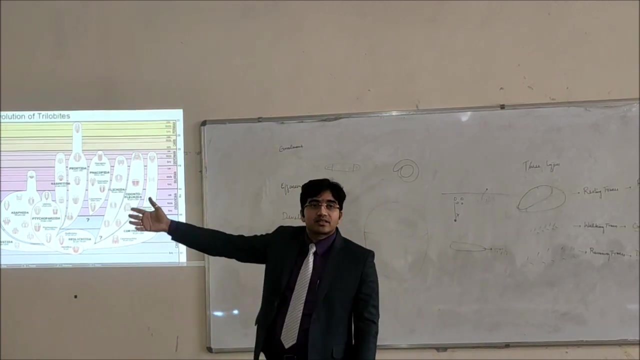 What is the importance of calcitic lenses and static arrangement in the trilobite eyes? So these are the things which you should think upon and then try to answer those questions. Then you can have this question discussed in detail. the evolution of trilobites. 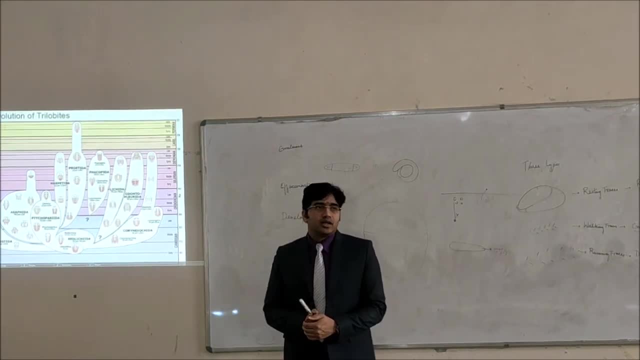 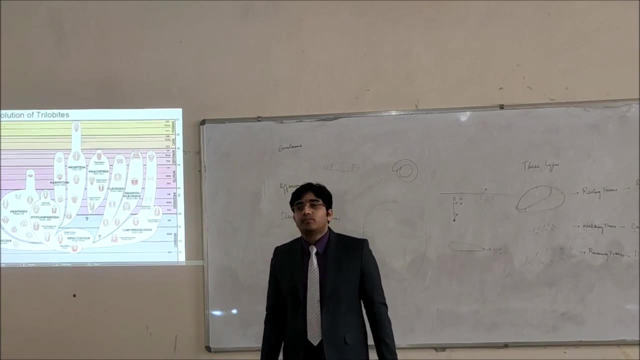 These are the very common questions which are asked in the ASI exams. And learn to make these diagrams. Learn to make these diagrams, so it will help you. Any questions, Sir? where did the evolution of phacopetal come from? 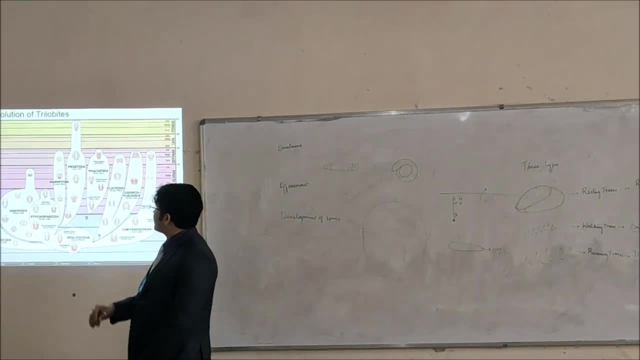 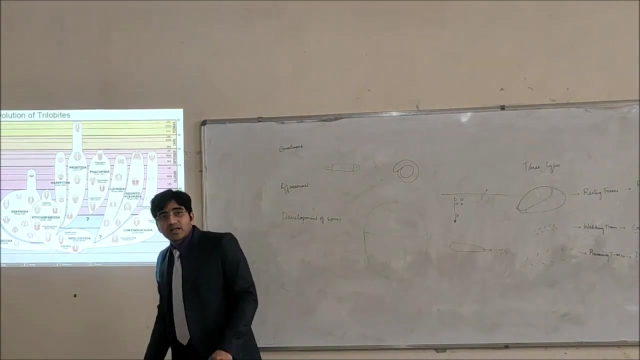 Phacopetal. Now the answers to this question mark we probably don't know. First of all, what did it bring? Then, after that, Phacopetal, Phacopina, Phagobina. So these are the classes of those orders. 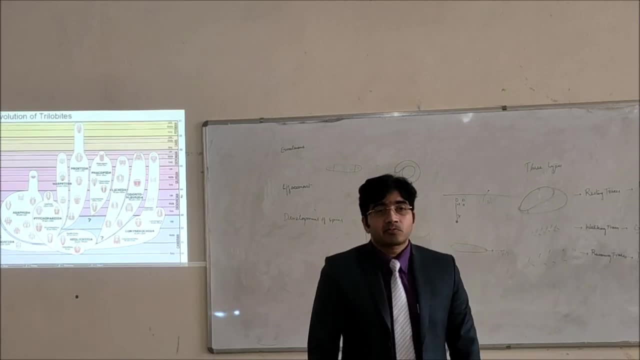 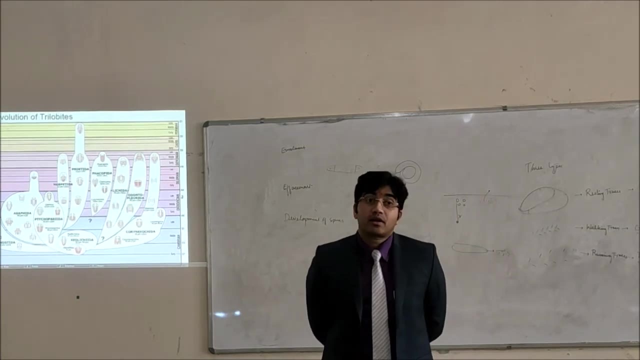 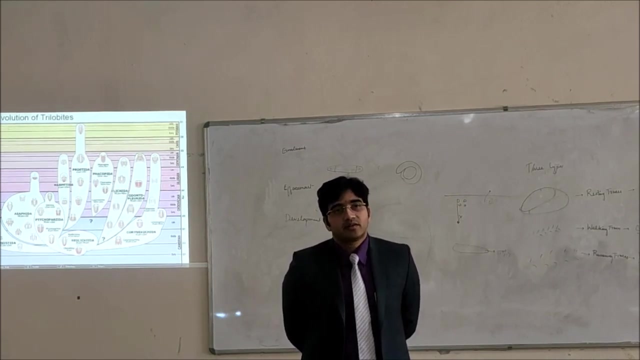 Sir, can we be also be ordered phacopeta? Look, if we go by the classification scheme, we can bring them by the class order genus. So at each stage there will be evolution. Starts with genus. Starts with genus. 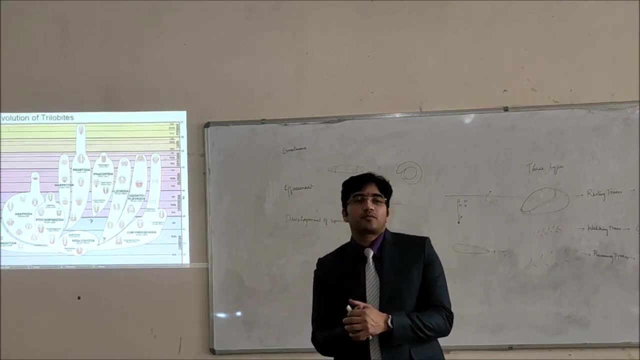 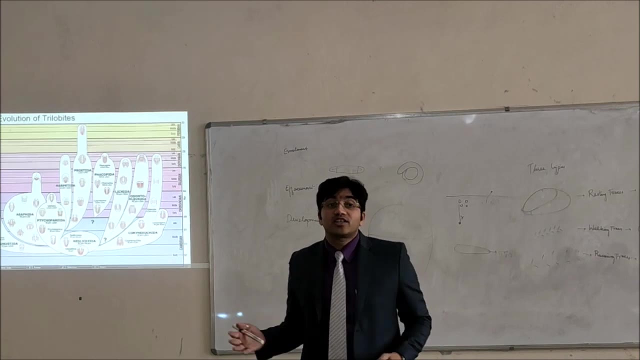 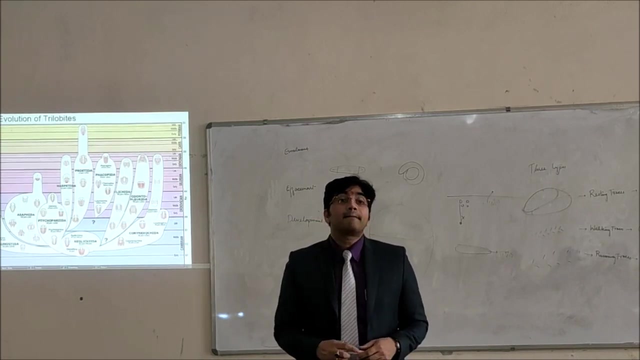 The genus and species are the last smallest kingdom phylum class order: genus and species. So genus and species are the last. that is the finest evolution. That is the finest evolution, Is it okay? Why did you start from the literature? 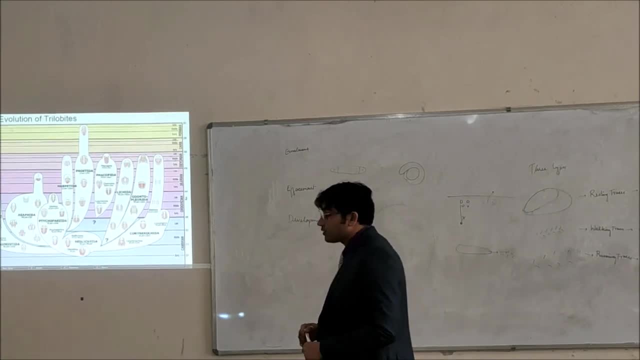 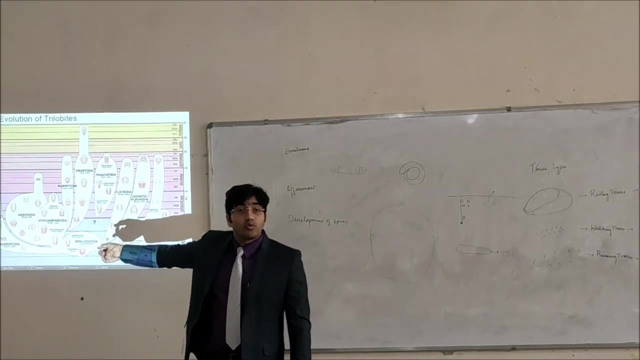 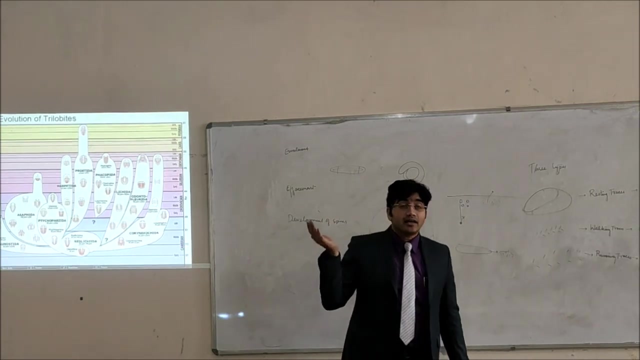 You came from the start. From what otherwise? You started from the literature, from the chemicals. I was the first one. What about its ancestors? Ancestor groups were not trilobites, They were idiotaraforms. I am telling you that the red lichida, or trilobite ancestor, was not an arthropod. 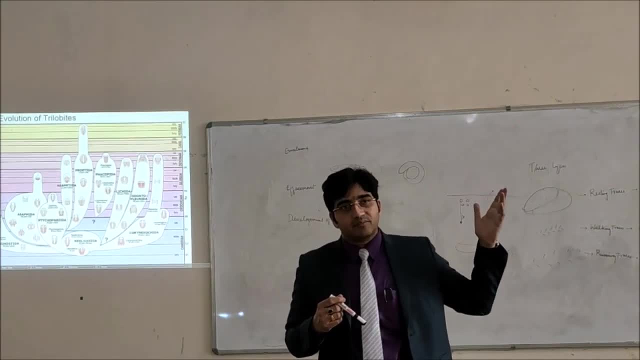 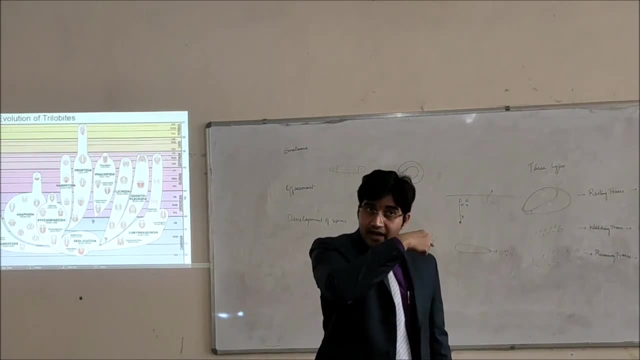 It was an idiotaraform, which is a completely different group of our ancestors. It started from that. Now, when we study mollusks, mollusks are a capybara genus, which is again an idiotaraform, But we do not consider it to be a mollusk. 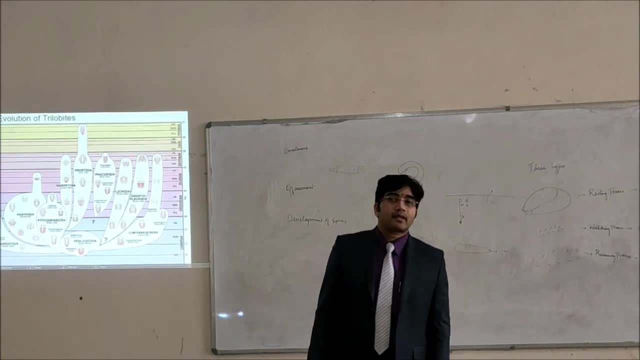 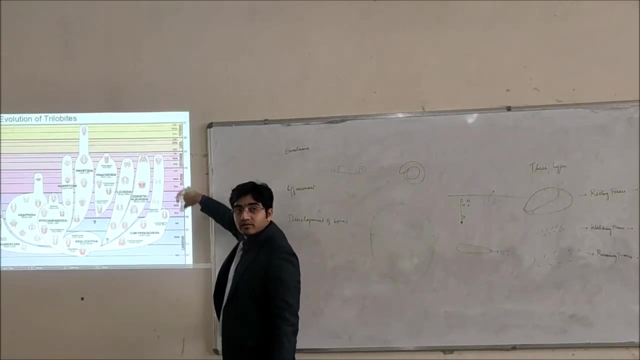 Okay, Sir, if there is a question. Okay, Is it okay? Yes, Major evolution period and trilobites. Is this yours? Yes, it is, And there is also a sensor in it. Okay, Sir, do you represent the index fossil? 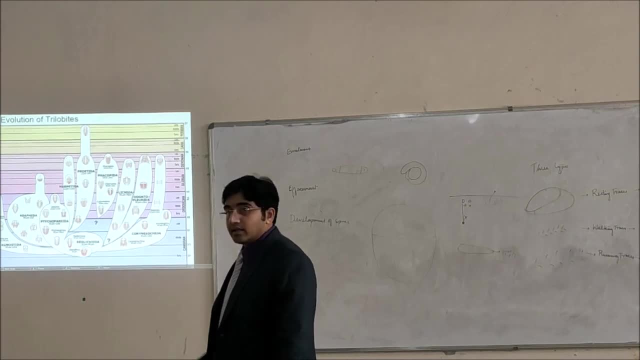 Yes, Which index fossil Aspirin, Aspirin, Aspirin index, Aspirin index, Is it so? Yes, it is. I mean, did you understand? Yes, I understood. See, how do we know the index fossil? 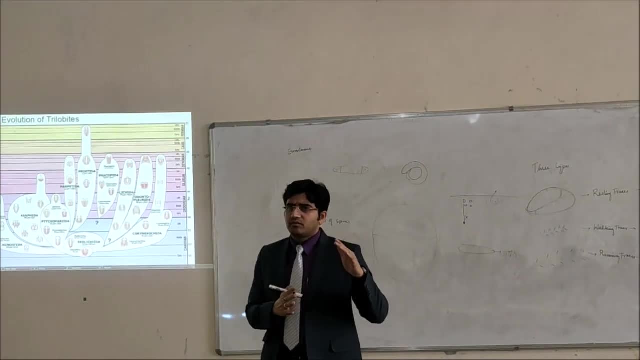 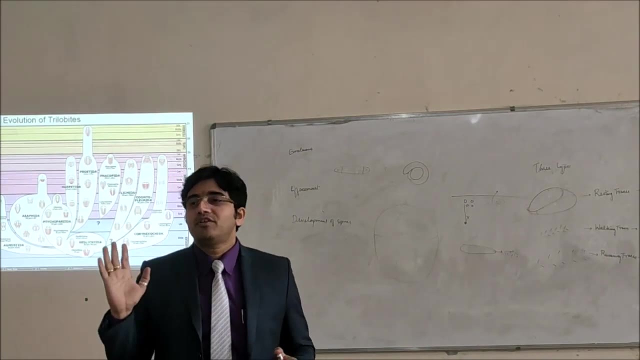 Which is given to us at any time period. We consider these as 90% of these, which is 100% accurate. So the age of these things is 10 years. In case of ileobites, the age of these things is 30 years.